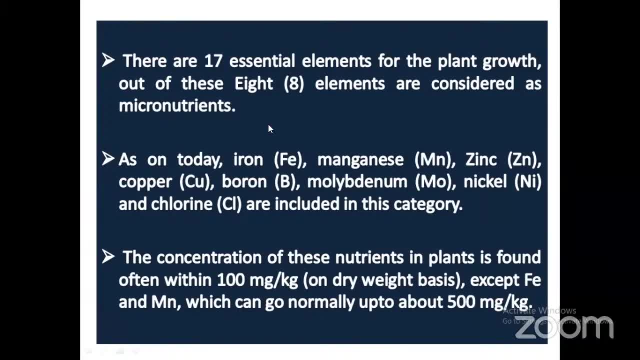 We will not count it, It will take our time. So directly, you remember that there are eight elements that are micronutrients And, as on today, iron, manganese, zinc, copper, boron, molybdenum, nickel and chlorine. They are included in this micronutrients category. 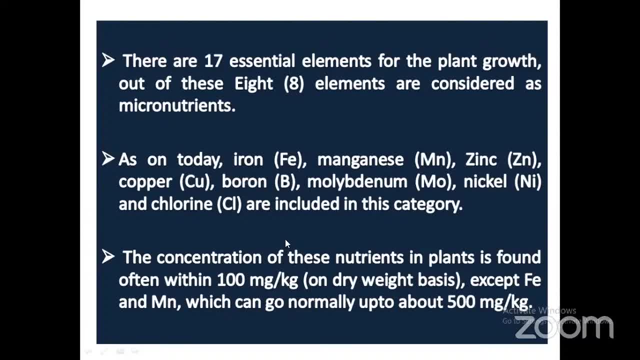 The constant, as I said, that micronutrients are the nutrients that are required in less amount. but what is the exact that less amount, quantitatively, we must know. So the concentration of these nutrients in the plant is found of Fenomena Dispersion. 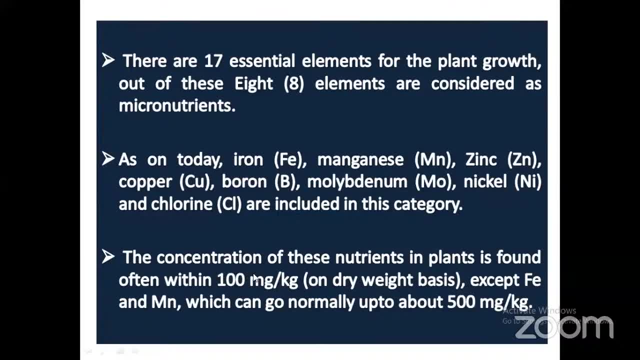 Fenomena, Fenomena, Desperation, Desperation, Fenomena. the concentration of these micronutrients in plant is found often within 100 mg per kg. what is this mg per kg, any one of you? is it ppm or ppb? 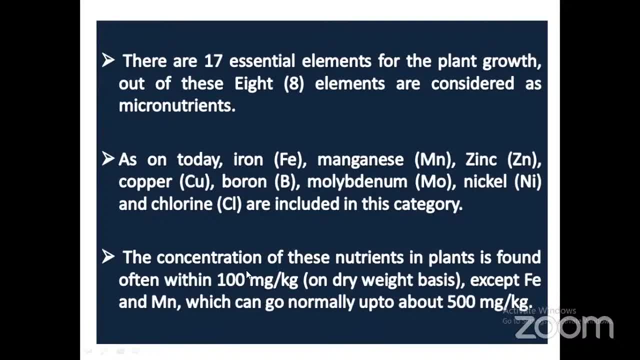 ppm. yeah, so the concentration of micronutrient plant is often within 100 ppm, except iron and manganese, which can go normally up to around 500 ppm also. so generally we can say that micronutrients are those nutrients that are required by the plant in means it is less than. 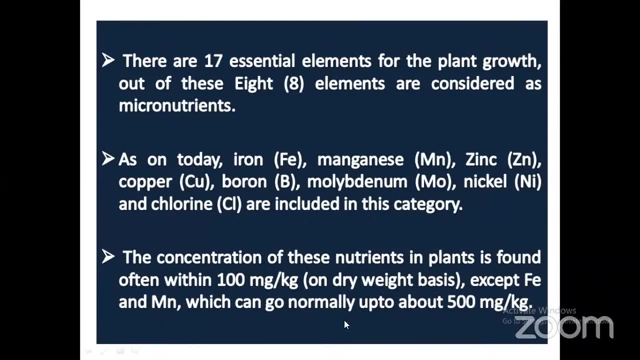 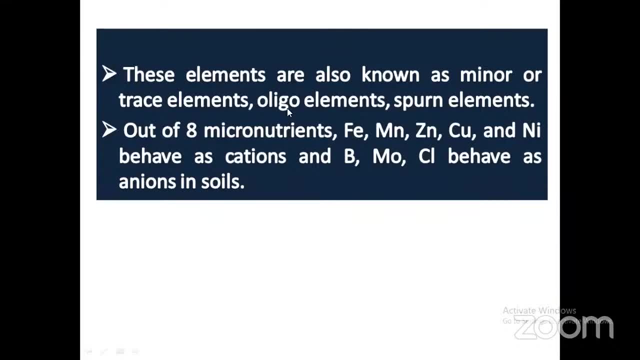 100 ppm. okay, exception is there with iron and manganese. that can go up to 500 ppm also. now these elements, these are some of the other names of micronutrients that can be asked in objective questions. the micronutrients are also known as minor nutrients. 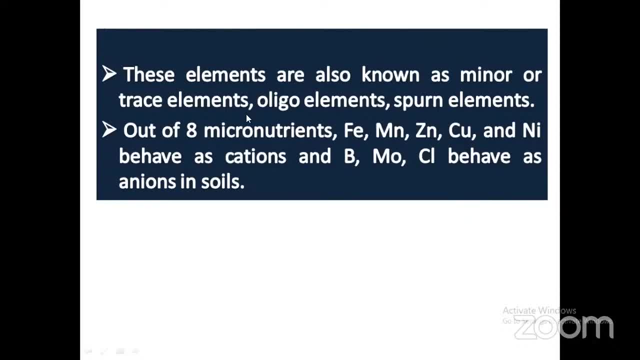 trace elements, oligo nutrients, oligo elements or spurn elements, so you should remember these name at least. and out of eight micronutrients, this: iron, manganese, zinc, copper and nickel- they behave as cations. and boron, molybdenum and chlorine: they behave as anions in the soil and the chemistry of 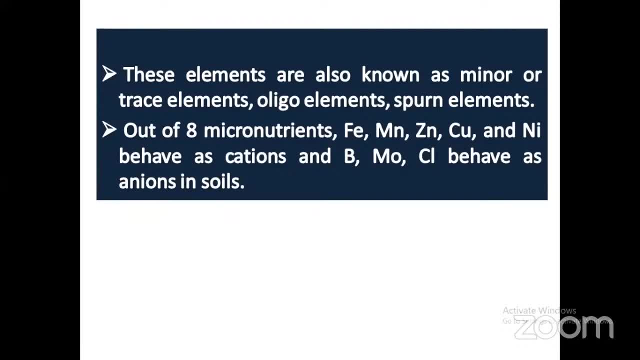 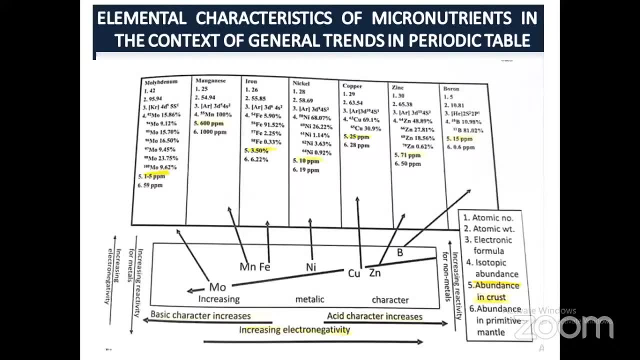 micronutrient cations is different from that of micronutrient anions, so we'll discuss them one by one and we'll see how they are behaving differently. now you see the elemental characteristics of micronutrients in the context of general trends in the periodic table. so if you see the atomic 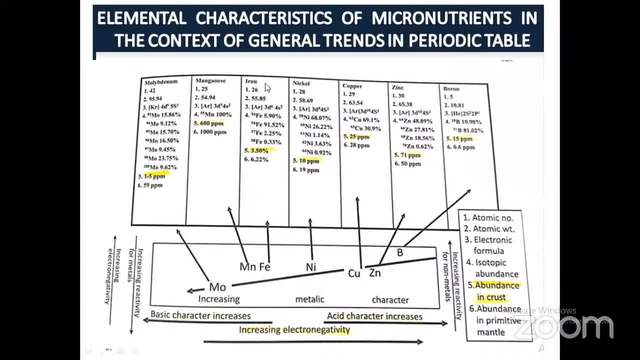 number of molybdenum 42, manganese 25, iron 26, nickel 20 and manganese 25. manganese 25, iron 26, nickel 28, copper 29, zinc 30, boron 5. you need not to remember all the information about these elements. 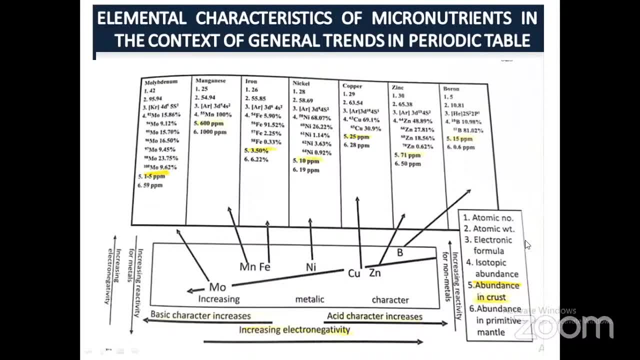 but yes, at least you should know the atomic number plus their abundance in the earth crust. you must have read it in pedology section also that molybdenum in the earth crust is around 1 to 5 ppm. this manganese is 600 ppm. iron 3.5 percent, nickel 10 ppm. copper 25 ppm. 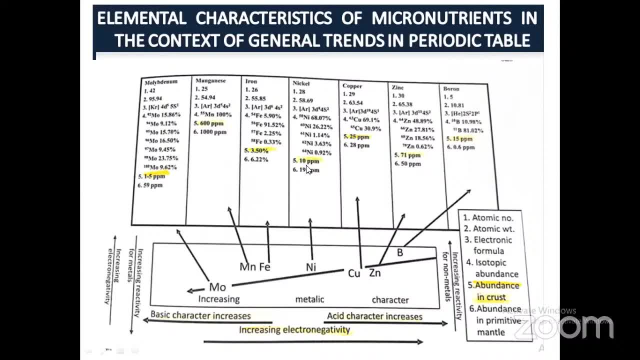 so these of presence in the Alrightrom es. as for thedzobites 소개 side, as I mentioned, this manganese is 600 ppm, iron 3.5percent, nickel 10 ppm, copper 25ppercent, nicr 18 percent, zinc 71 and boron 15 ppm. At least you should remember this atomic number and their abundance. 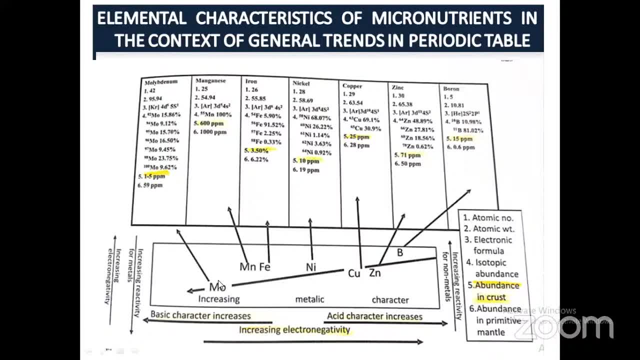 in the earth crust. Another thing is, when we go from this molybdenum and to this boron, there is increase in the electronegativity. The electronegativity of this boron is highest if we see all these micronutrients and this molybdenum is least. Now, before seeing the trend, let us first 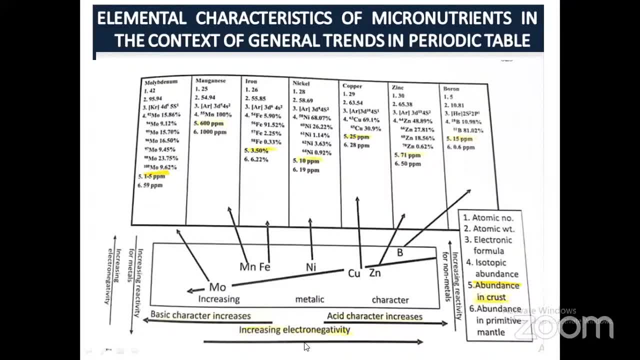 understand what this electronegativity means. If anyone of you want to tell me what electronegativity means, you please proceed. If no, you simply say no, so that I move ahead. No one, Okay? so electronegativity is the tendency of any atom, of the element, to attract shared 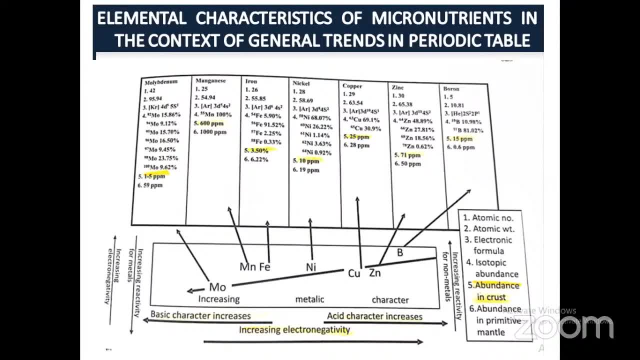 electrons. So it is tendency of any element to attract electrons. So this boron is having high electronegativity means it is having the tendency to attract electrons, and this molybdenum is having least electronegativity. if we see these, 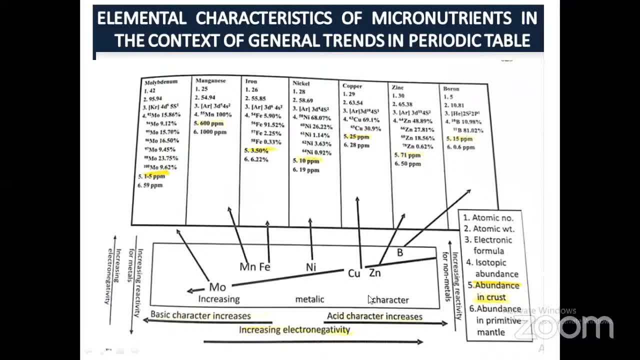 elements. Now this electronegativity is affected by the atomic number, The element that is having least atomic number. you see, this boron is having five atomic number. that means electrons surrounded. electrons around this boron are very less, So they are nearer to the nucleus, So less the atomic 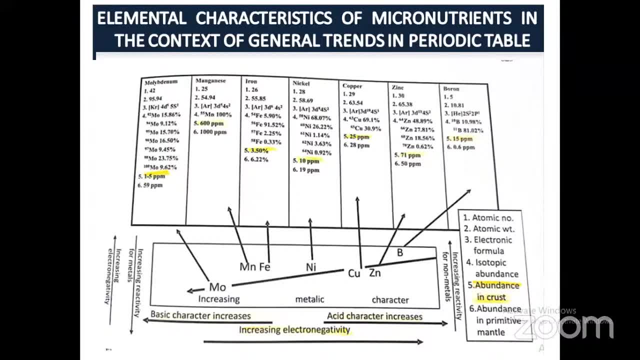 number and the distance at which these valence electron reside from the charged nucleus. If the distance between the nucleus and the electron surrounding that atom is less, that means positive charge is relatively more, So electrons can be attracted to that particular element. So 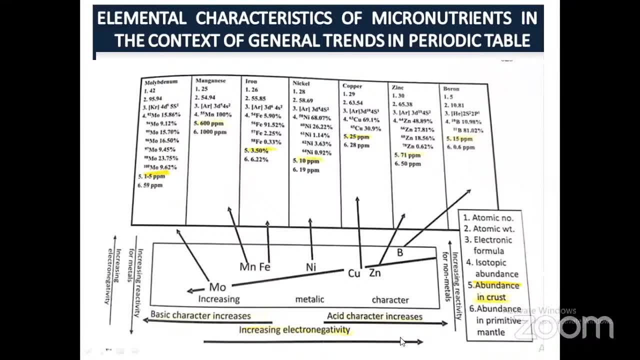 as the atomic number of electrons is less than the atomic number of electrons around this boron, the atomic number decreases. electronegativity increases. This is one thing. Another is acid corrector increases from molybdenum to boron. So boron is behaving more acidic and molybdenum is. 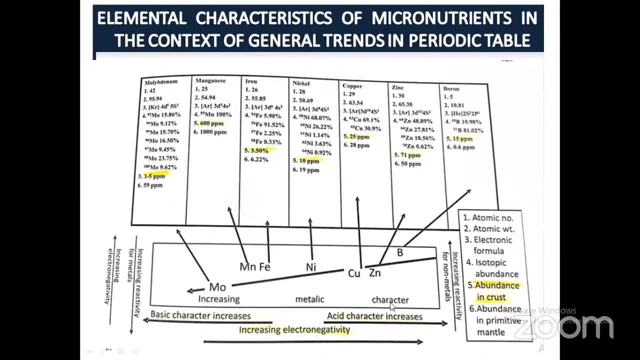 behaving basic in nature. So what is this acid corrector means, you see, Acid corrector is the ability or tendency to lose a proton. So boron is having tendency to lose the proton easily and molybdenum is having less tendency to lose the proton. So towards boron, this acidic corrector. 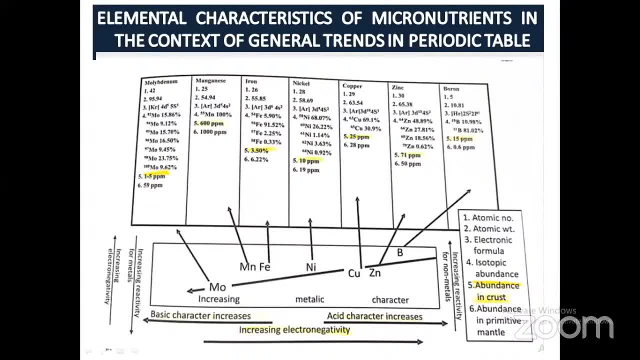 increases. You see, as we move from left to right in a periodic table, the atomic size of the element decrease. If the atomic size of the element decreases, which means electronegativity increase, Jitna kam atomic size hoga utna zyada electronegativity, hogi Electrons ko bahut. 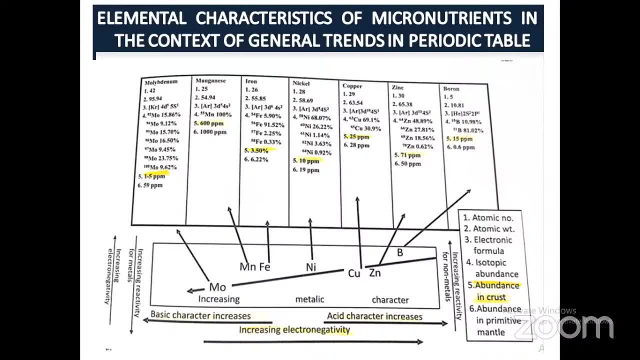 asani se ho attract kar lega, Aur agar electrons ko accept asani se kar raha hai. that means it is more polar, So it is easy- relatively easy- to lose proton, So boron acidic corrector is more, and this molybdenum is behaving like a basic. So from this slide, what is important to remember is: 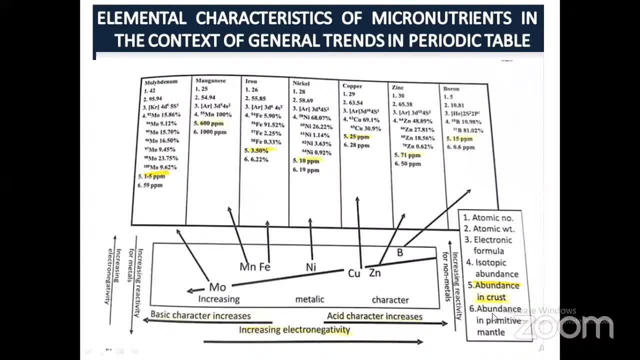 the atomic number of all the elements, their relative abundance in the earth crust, electronegativity, behavior of all the elements. At least you should know the sequence, or agar, wo bhi yaad ni rakhna, Toh you should remember which one is more electronegative. 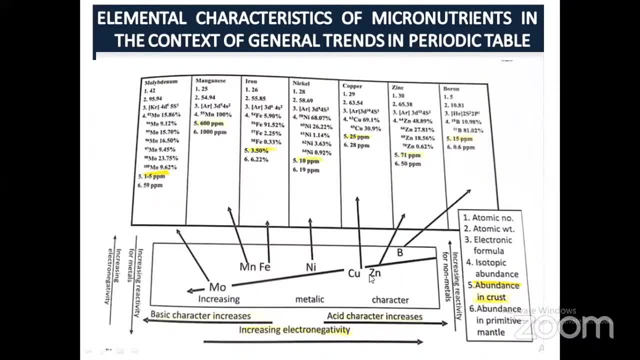 and which one is least. Okay, this is the least, While taking in mourning will not be expected from you. Another is acid corrector behavior and basic corrector behavior. So this is this slide is, for this purpose, only to get you the general idea of all these micronutrient elements. Now moving ahead: Geochemistry. 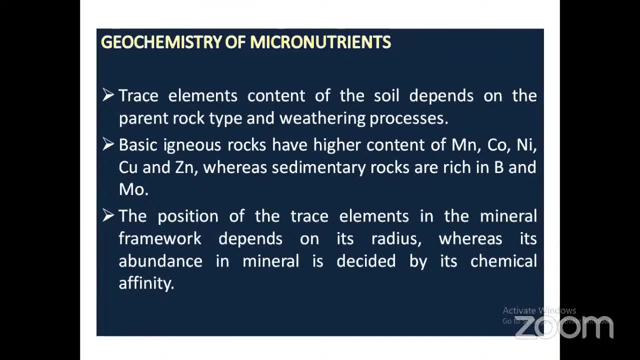 of micronutrients. if anyone of you want to tell whether my speed is okay to all of you or I should go little slow. Yeah, it's okay, bhaiya. So geochemistry of micronutrients. you see trace effect. Now you are getting kind of used to the analysis. It is running through Excel and because I get petits plus scale. So then you exposed them to OK k new in uimagina uimimia k wNo k to rubbish Now going ahead. Geochemistry of micronutrients. If anyone of you want to tell whether my speed is. 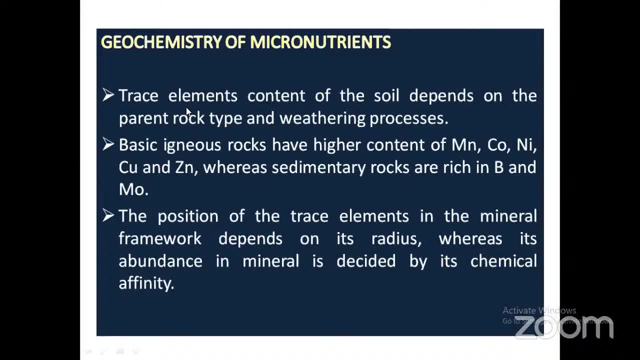 micronutrients. you see trace elements. this is the other name of micronutrient. only trace elements. content of the soil depends on the parent rock type. which element is there in the soil? it depends on the parent rock, because ultimate source of these nutrients in the soil is the parent rock. 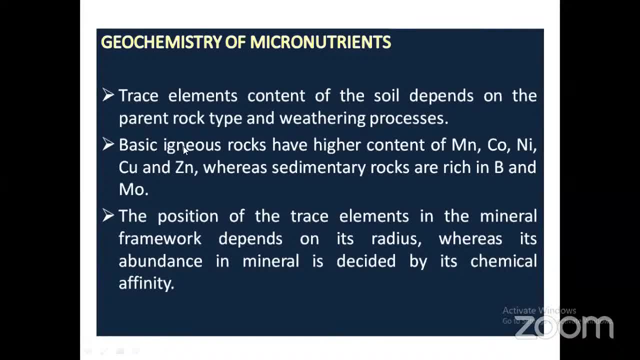 and the weathering processes. we know that there are three kinds of rock: igneous, sedimentary and metamorphic. and under igneous rocks, we also know that there is acidic rock, basic rock, ultra basic. so this basic igneous rocks have higher content of manganese, cobalt, nickel, copper and zinc, whereas 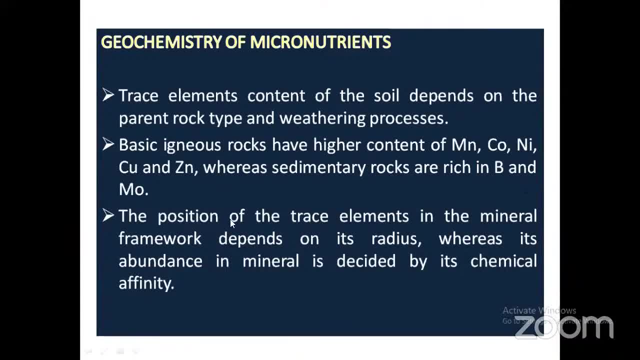 sedimentary rocks are rich in boron and molybdenum, and during the crystallization of the minerals in the rock formation, trace elements enter in the framework of the minerals. when there is crystallization of minerals and when there is formation of the rocks, these trace elements enter into the framework. 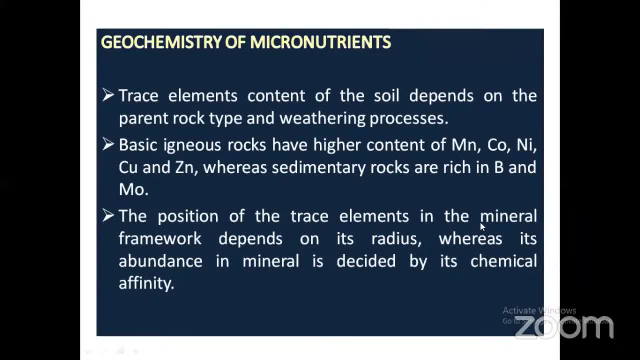 of the element and the position of these trace elements in the mineral framework. it depends on its radius. we know that mineral. there are different structures of minerals. now, one is to one, two is to one, two is to one is to one. you must have read it in pedology section. so, depending upon the size of the 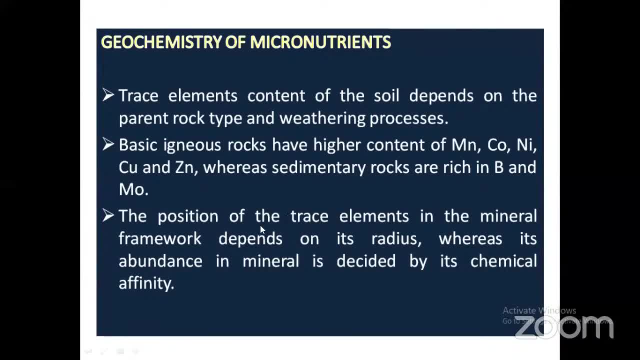 particular element. this trace elements can take position in the mineral framework, whereas its abundance in the mineral is decided by its chemical affinity. the element which is having more affinity towards means if it is more reactive, then it will be more abundant in a particular mineral. so the position of the trace element depends on its radius and its abundance depends. 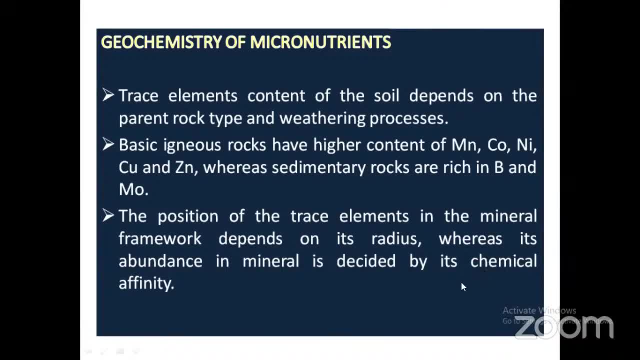 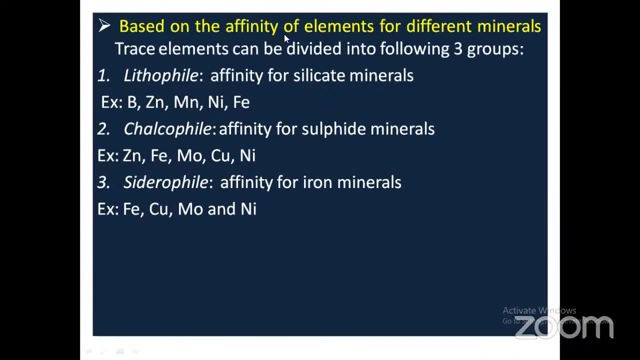 on the chemical affinity. more affinity it is having. more will be the particular element in the mineral and based on the affinity of the elements. for the different minerals, trace elements are divided into three groups based on their affinity. right, so it is deciding the abundance of the mineral. 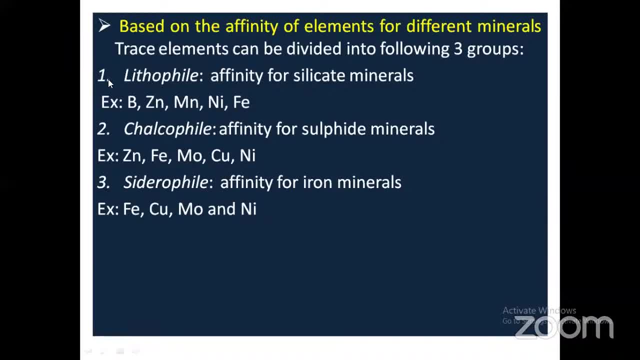 right. so, based on the affinity, we have three kinds, three groups. one is lithophile, another is chalcophile, next is siderophile. lithophile is one that is having high affinity for the silicate minerals, and the elements that comes under this category are boron, zinc, manganese, nickel and iron. 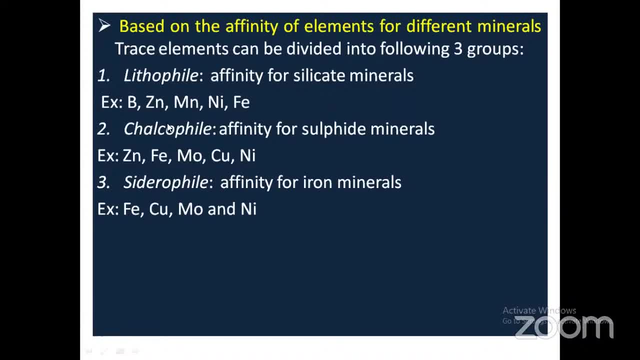 so they are lithophiles and they have high affinity for the silicate minerals. another is chalcophile. they are the elements that have that are having high affinity for sulfide minerals. they form covalent bond with the sulfide minerals. sometimes it is asked in exams that which one of the following group of elements form covalent bond with the: 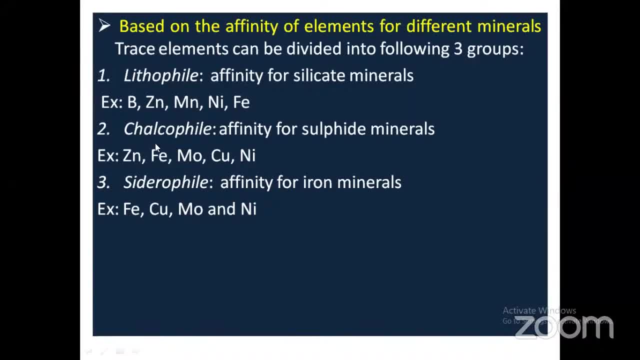 sulfide minerals, so it is chalcophile. Examples are zinc, iron, molybdenum, copper and nickel. another category is siderophile. These are the elements that are having high affinity for iron minerals. examples: iron, copper, molybdenum and nickel. another category is also there, which 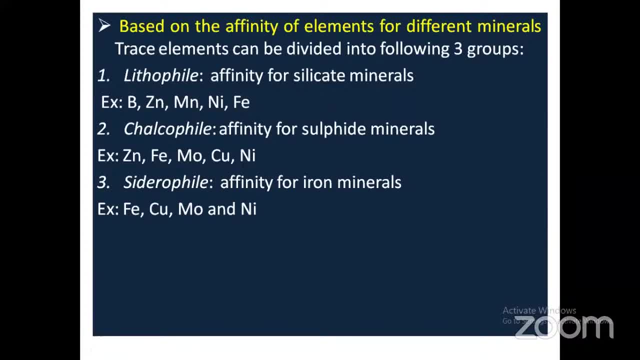 Which one is left? Any one of you Lithophile, sargophile, siderophile? One more is there? Yes, Okay, fine, Another is repeat, please, I'm not getting you. You please speak it again: Atmosphines. 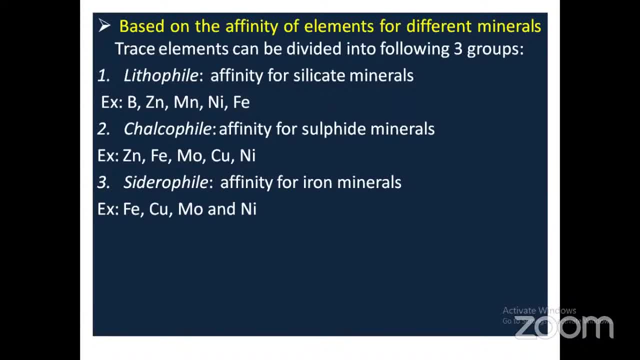 ma'am. Okay, fine, So atmosphile is also one category, means the elements that are present in the atmosphere, But here we are talking about the affinity of elements to different minerals, right? So that is why atmosphile 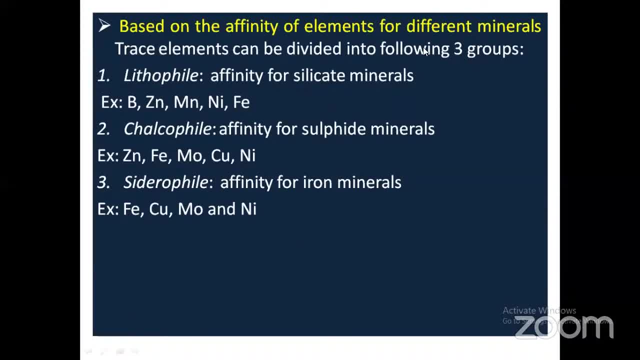 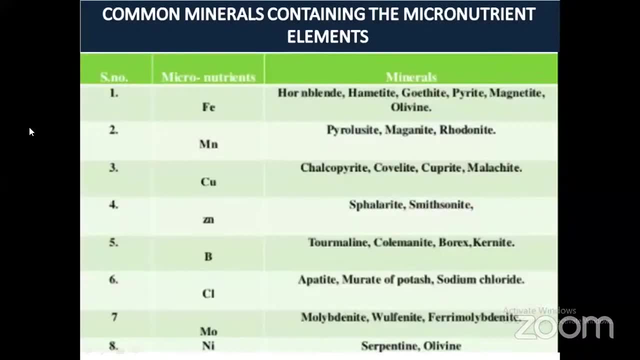 category I have not written because we are talking about affinity to different minerals only. okay, Now moving ahead, coming to different sources of these minerals: micronutrients: there are different minerals in the earth crust and they are the sources of micronutrients. 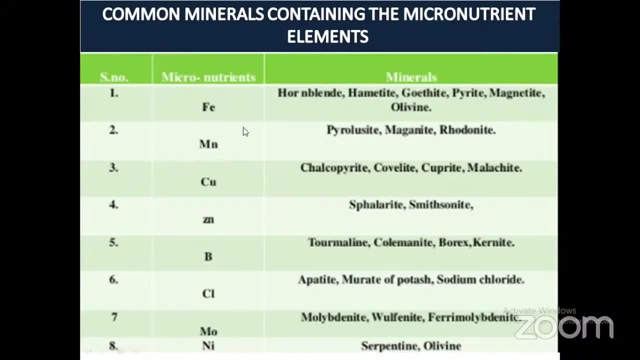 and this slide is very important from exam point of view. In most of the times I have seen objective questions from this particular slide that a particular mineral is given and you are asked which means this particular mineral is a source of which micronutrient? 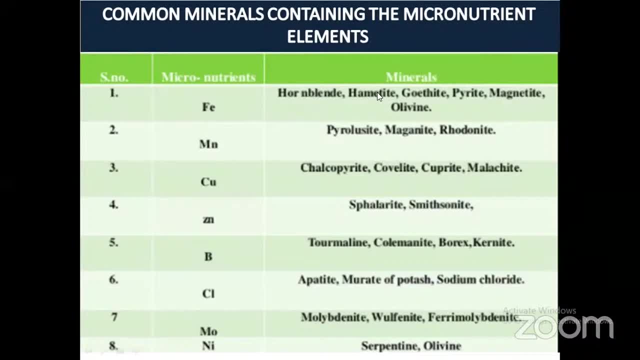 okay, So iron, we have hornblende, hematite, goethite, pyrite, magnetite, olivine, and this pyrite is other name of pyrite. any one of you Fools gold ma'am? 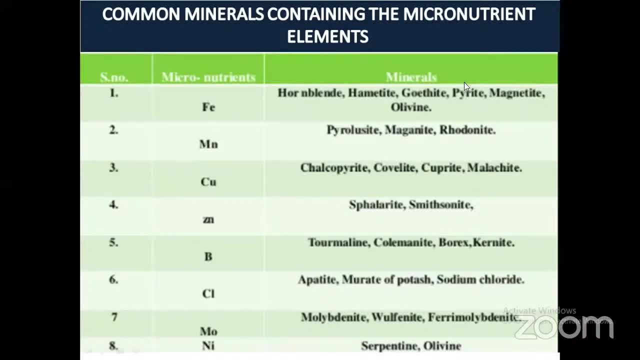 Yeah, wonderful. And its chemical formula, Marcosite, FES2.. FES2, yeah, FES2.. Marcosite is also one of the polymorph of pyrite. yeah, but this pyrite is FES2 and it is. 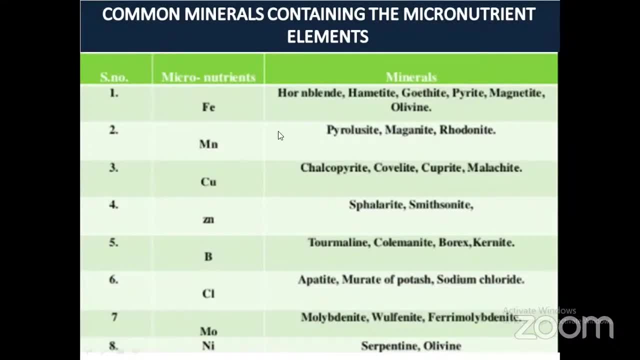 Fools gold. okay, So this question can also be asked. So iron minerals are hornblende, hematite, goethite, pyrite magnetite, olivine, Manganese minerals, Pyrolocyte magnetite. 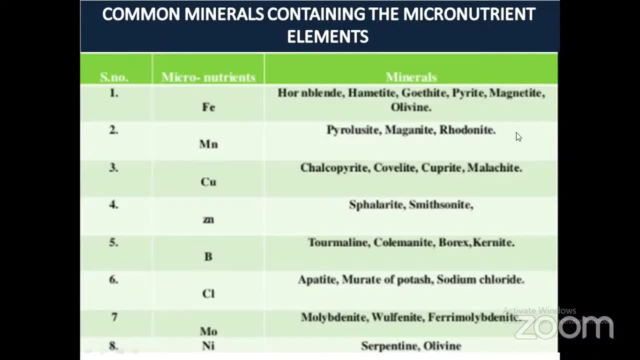 magnetite. is also there rhodonite, any other manganese mineral, if you know? Yes, Other than this pyrolocyte, rhodonite magnetite? Have you heard of rhodochrosite? Yes, No, Okay. 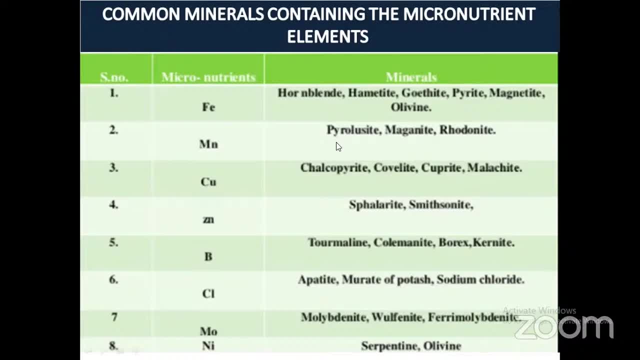 you're right. Another manganese mineral is: you write it is sometimes asked in exam. You write rhodo, r-h-o-d-o and c-h-r-o-s-i-t. rhodochrosite. Another is hosmenite: h-a-u-s-m-a-n-n-i-t. 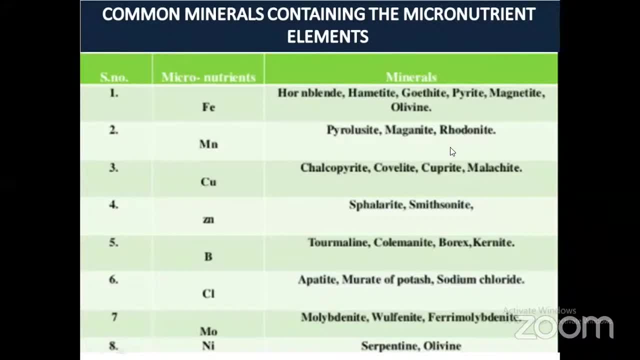 So pyrolocyte, magnetite, rhodonite, rhodochrosite, hosmenite- these are manganese minerals. Generally, this pyrolocyte is asked in exam, but yes, we should have an idea of all. 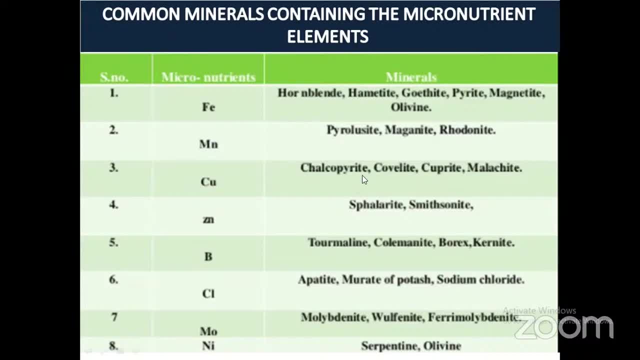 Next is copper. So copper minerals are chalcopyrite, covalite, cuprite, malachite, One more mineral that is. I have seen in recent objective books that they are asking that particular mineral also. So if you, 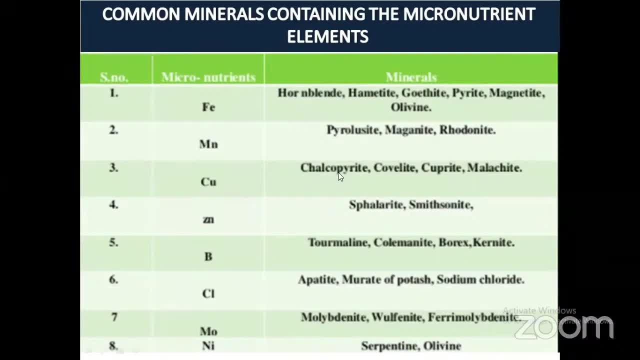 want to tell me any other mineral of copper? any one of you? hint for you. it starts from the A, capital A. It's a right one. Yeah, wonderful. So copper minerals. you write chalcopyrite, covalite. 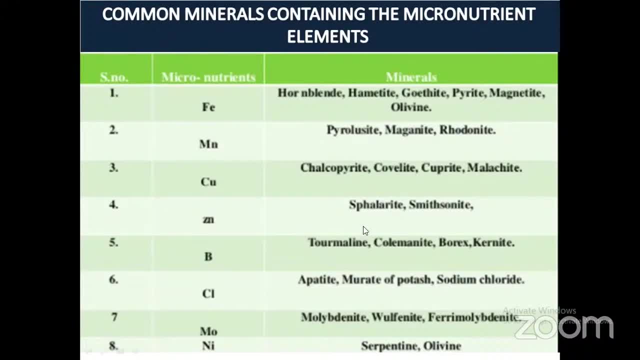 cuprite, malachite and azurite. Okay, next is zinc. Zinc containing minerals are sphalerite, smithsonite hemimorphite is also there, So sphalerite, smithsonite hemimorphite. 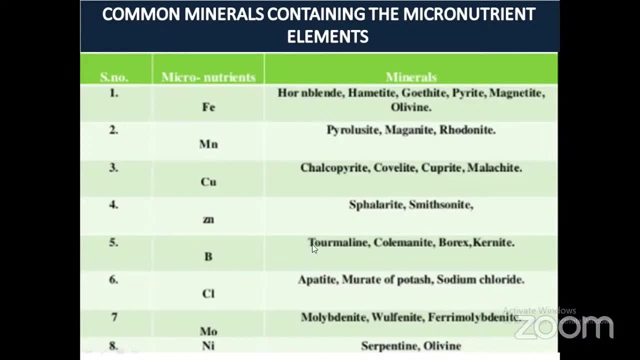 Boron containing minerals, tourmaline- very common question- chalamanite, borax, carnite. Another is chlorine containing minerals. So it is apatite murate of potash, KCL, sodium, chloride, NaCl. 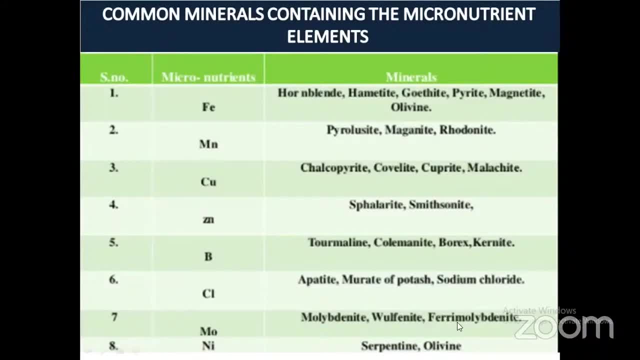 molybdenum containing minerals: molybdenite, wolfenite, ferrimolybdenite- Another molybdenum containing mineral that is asked in objective question. you write: it is sphalite, P-O-W-E-L-L-I-T-E. 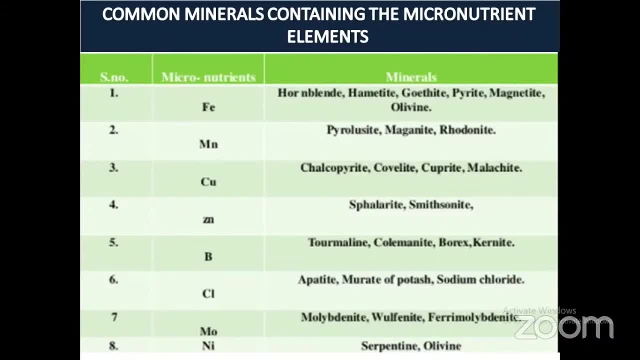 sphalite. this is calcium molybdenate C-A-M-O-O-4.. So molybdenite, wolfenite, ferrimole molybdenite. another is sphalite Nickel containing. 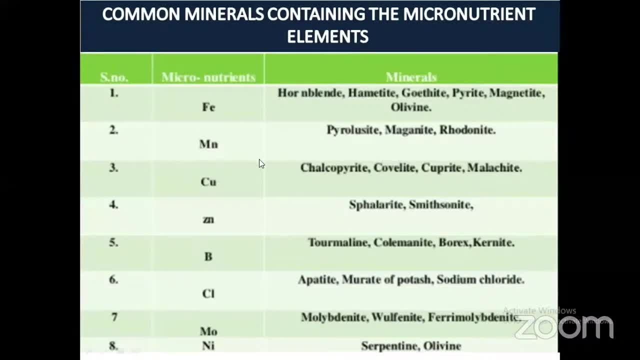 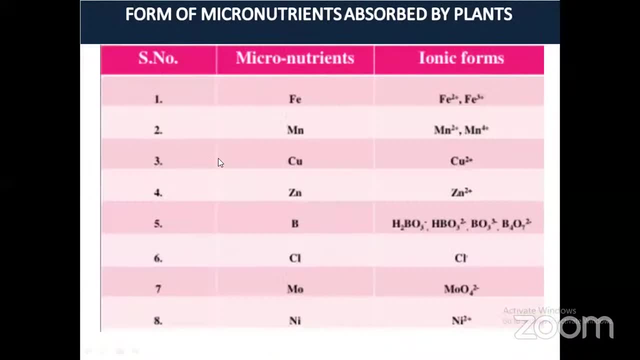 minerals: serpentine, olivine. This is very important table, so we will show it carefully. Now, moving ahead, as we have seen in the starting slides that there are certain micronutrients that are taken up by the 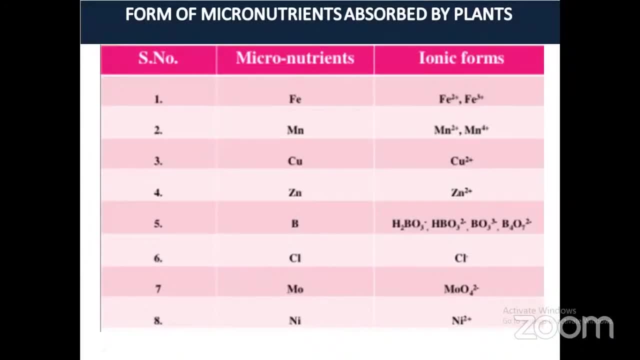 plants in cationic form and there are certain micronutrients that are taken up by the plant in anionic form. More specifically, there are five cationic micronutrients and three anionic micronutrients, So their ionic form. 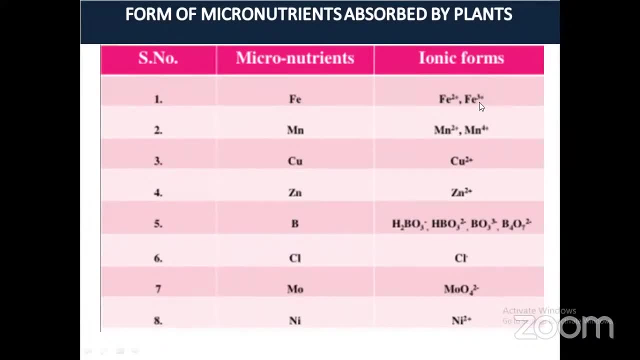 iron is taken up by the plants in Fe2+, Fe3+, ferrous and ferric form. which one is ferrous and which one is ferric? Fe3+ ferric, Fe3+ ferric- yeah, So it is ferric. and 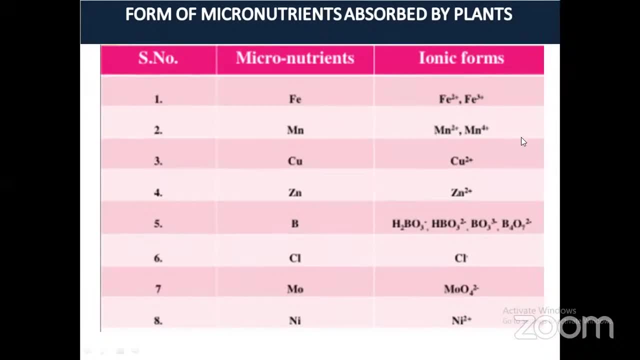 this one is Fe2+ ferrous form. Magnesium in Mn2+, Mn4+, copper in Cu2+, zinc, Zn2+. boron is mainly taken up by the plants in boric acid form in neutral H3BO3,. 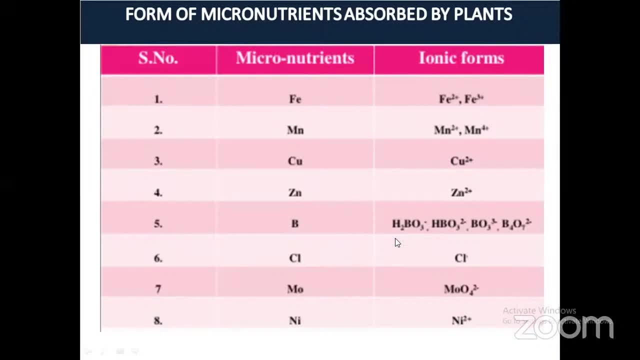 but yes, other forms of boron. that means that can be converted. that is H2BO3-. we will see this one by one. So these are the different ionic form of boron. Now chlorine is taken up by. 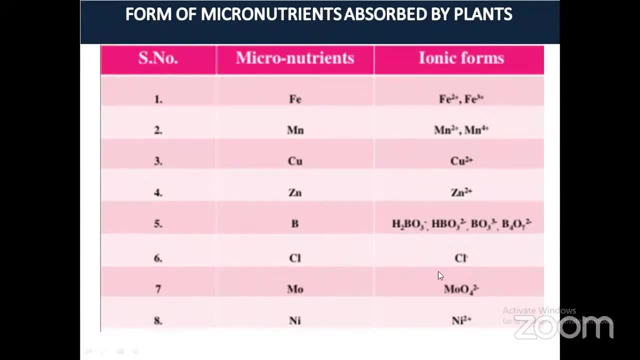 the plant in chloride. this is an ionic form. molybdenum in molybdenum in iron, nickel, Ni2+. So these are the ionic forms of these micronutrients. Now taking these micronutrients. 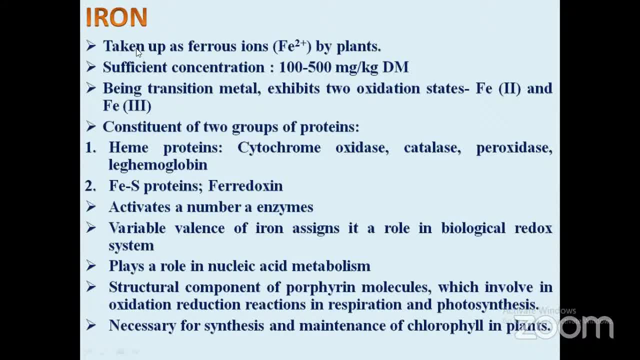 one by one. first one is iron. it is taken up by the plant as ferrous form, Fe2+ form, by the plant In soil. ferrous and ferric form are Fe2+ and Fe3+. both are there but plant. 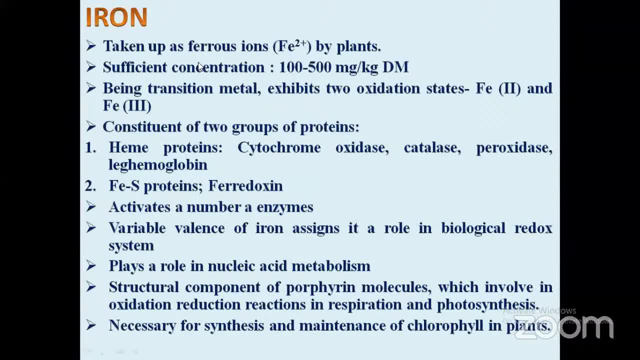 take up this ferrous form, Fe2+, and the concentration of iron in the range of 100 to 500 ppm in mature leaf tissue is regarded as sufficient for optimum crop production. So the sufficient concentration of iron for optimum crop production is 100 to. 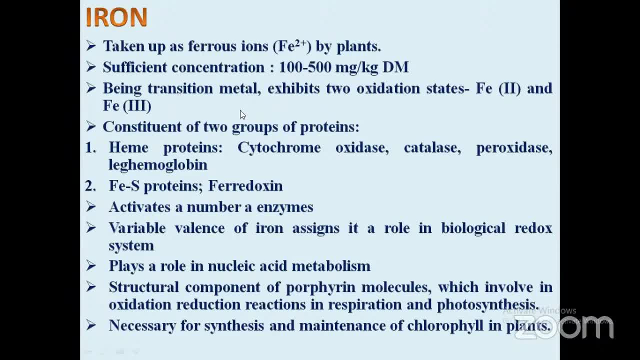 500 ppm. And since this iron is transition metal, so it exhibits two oxidation states: Fe2+ and Fe3+. it is constituent of two groups of protein: One is hemiprotein, another is iron-sulfur protein. So 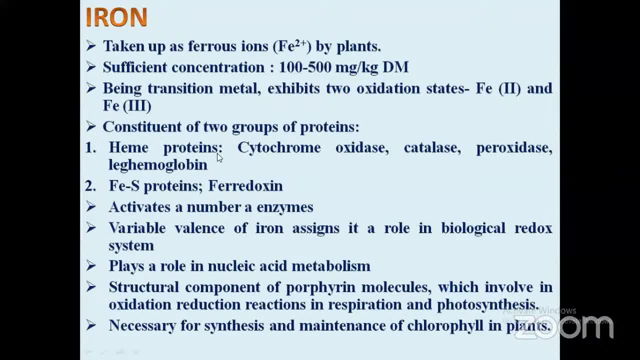 hemiprotein means it is one that contains iron in porphyrin complex. So hemiproteins are those proteins that contain iron in porphyrin complex. So what is this? porphyrin means Porphyrin. 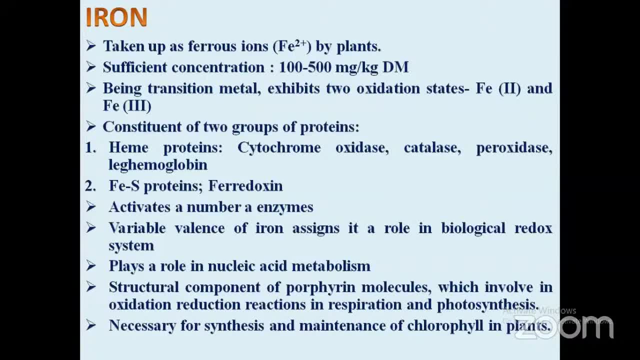 means it is an aromatic macro-cyclic compound. So it is a ring-type compound that consists of four bridging carbon units. You must have read the structure of chlorophyll. I guess There are four pyrrole rings and magnesium is. 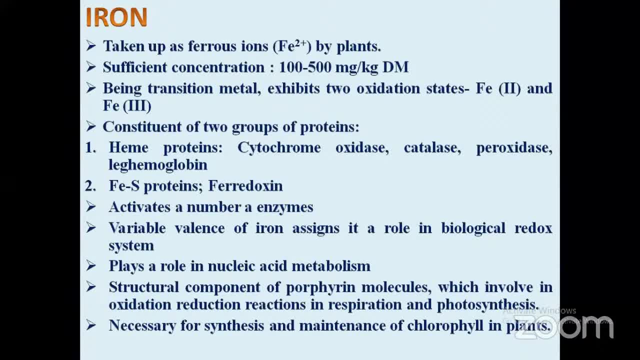 in center right. So porphyrin means this cyclic compound. So hemiproteins are those proteins that contains iron in the porphyrin complex And the examples of these hemiproteins are cytochrome oxidase. 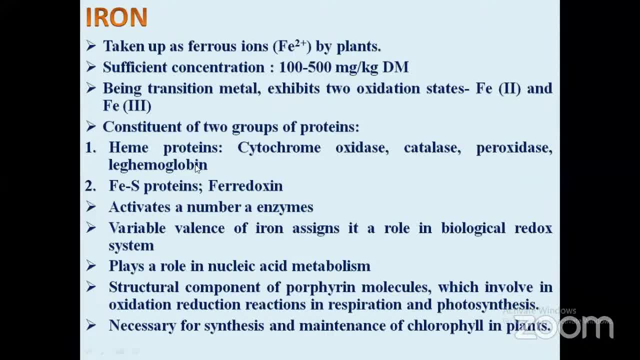 these are the enzymes: catalase, peroxidase, leg hemoglobin. Another is iron-sulfur protein, And the example of this kind of protein is ferredoxin. So iron is a component of hemiproteins and 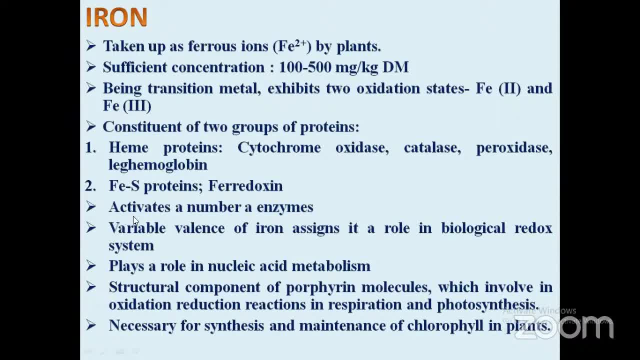 this iron-sulfur protein, that is, ferredoxin. This iron activates a number of enzymes and, because of its variable valency, it is assigned the role of biological redox system. So, since it is having variable valency- 2 and 3. 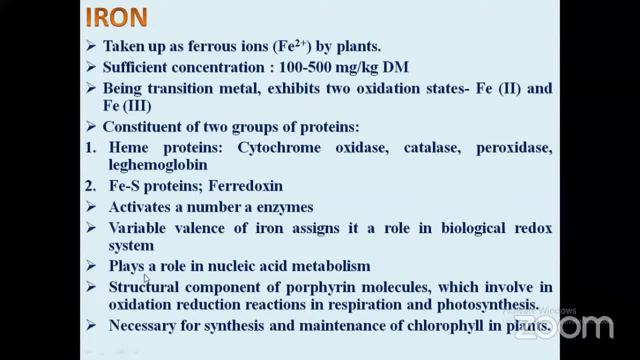 plus. so it is having role in the redox system, It plays a role in nucleic acid metabolism and it is a structural component of porphyrin molecule which is involved in oxidation of reactions in respiration and photosynthesis, and it is necessary. 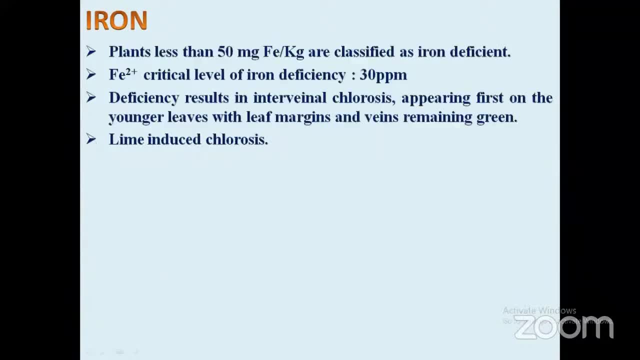 for synthesis and maintenance of chlorophyll in the plants. Now the plants that are having less than 50 ppm of iron are classified as iron deficient. Somewhere it was written that Fe2 plus critical level of iron deficiency means if the Fe2 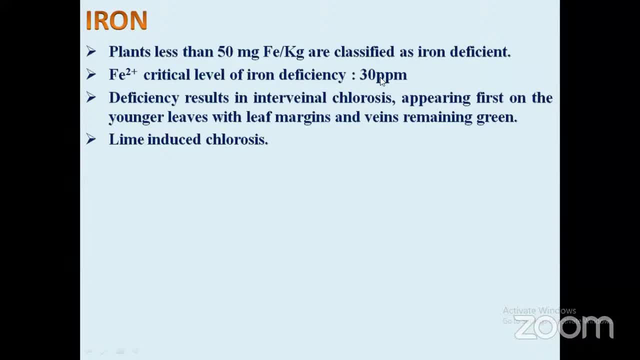 plus concentration in the plant is less than 30 ppm, then there is deficiency of iron, right? So these are two statements. One is saying that if the plant is having less than 50 ppm of iron, it is iron deficient. Another is: 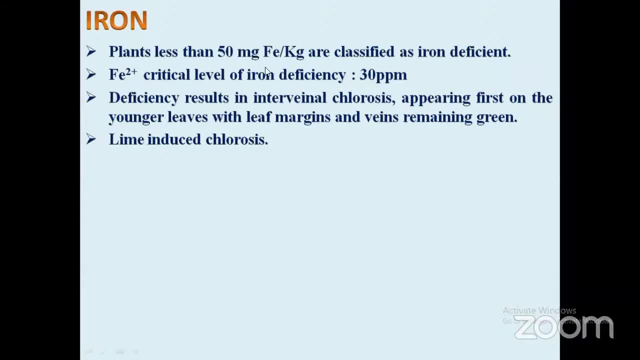 saying: if it is less than 30 ppm of iron, then it is deficient. So if you are able to find out the difference between these two statements, you tell Anyone of you, Ma'am. in first one, iron may be in. 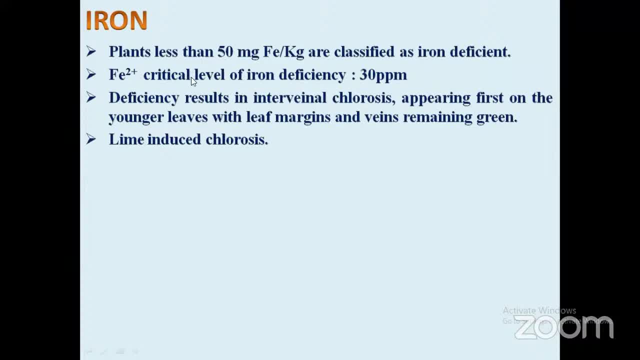 form of terry. Okay, Any other one to tell any difference. if you are able to find out, Anyone of you want to try. This is one thing that could happen means if it is Fe3 plus and this is Fe2 plus. 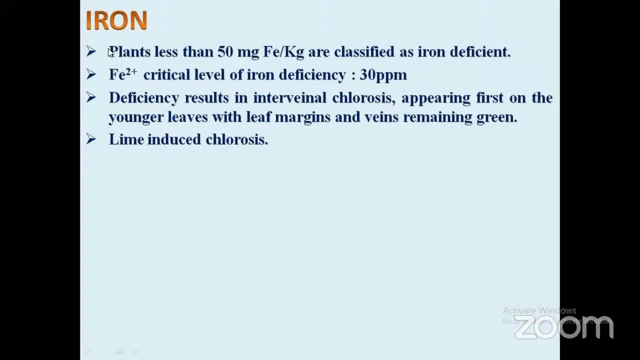 Or kuch. koi sochna chayega, ki kya ho sakta hai possible difference. dono mein Galat hi to hoga. soch to sakte hai na Bolo. Okay, fine, Nahi bolna. 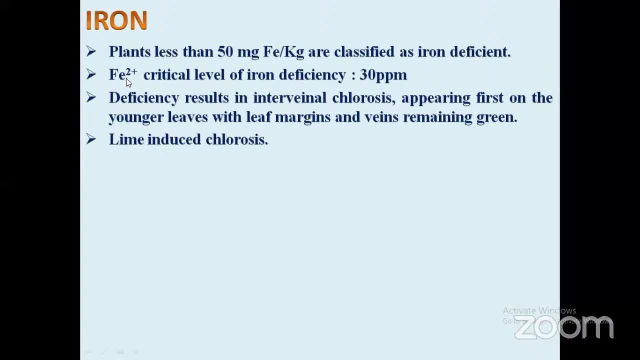 theek hai. So this is saying that if Fe2 plus this ferrous, if it is less than 30 ppm, then it is deficient in plant. This one is not for ferric, actually, this is for total iron Ferrous. 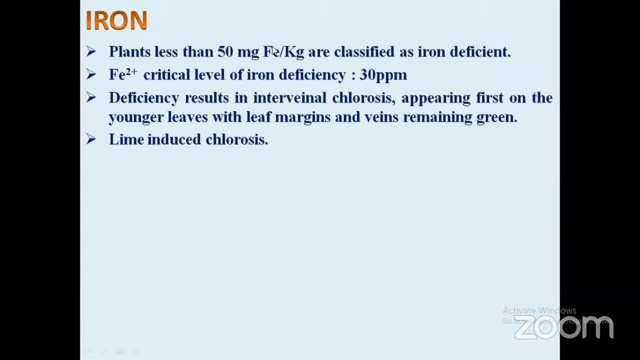 and ferric, both Okay. this is for total iron. So if total iron content is less than 50 ppm, then it is iron deficient, and if ferrous- specifically it is asking- it is less than 30 ppm, then it is iron. 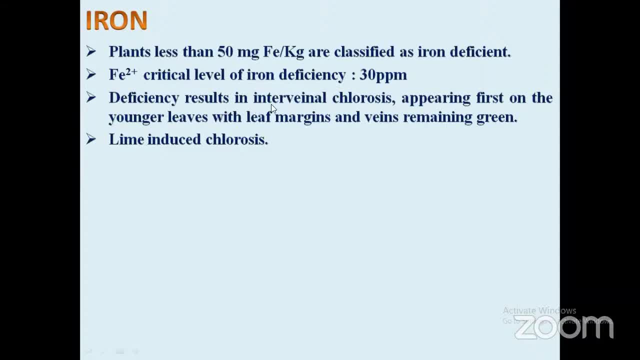 Now the deficiency of iron results in intervenal chlorosis appearing first on the younger leaves, with leaf margins and veins remaining green. So if iron deficiency is first appearing on the younger leaves, you tell whether iron is mobile or immobile in plant. 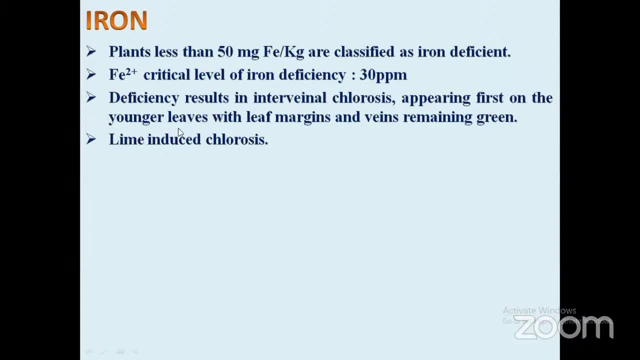 Immobile. Yeah, So if deficiency is seen in the younger leaves, it is immobile and unneeded. Another is lime-induced chlorosis. Because of the lime application there is deficiency of iron and that induced chlorosis. So it is. 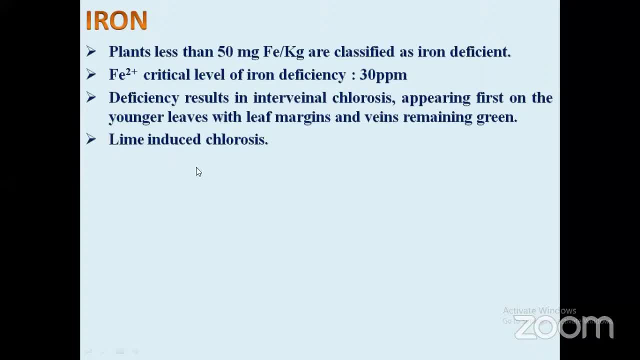 very common question in exam. Which of the following element causes lime-induced chlorosis? So it is iron. That means because of the application of lime. what does this lime do? What is the effect of lime on soil pH, Whether it increases or? 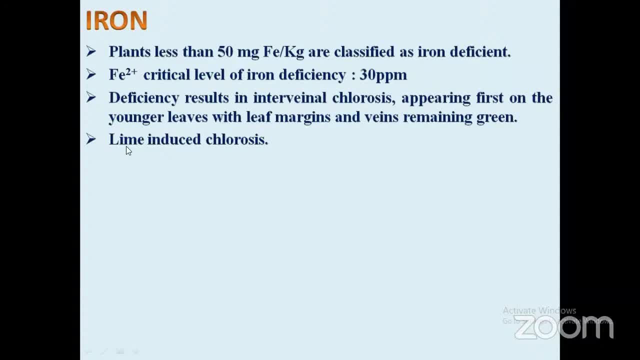 decreases soil pH. Decreases soil pH. Decreases soil pH. Increases soil pH. Okay, Those who are saying that it decreases soil pH. you tell me whether lime is applied in acidic soil or alkaline soil. Yes, Acidic soil. 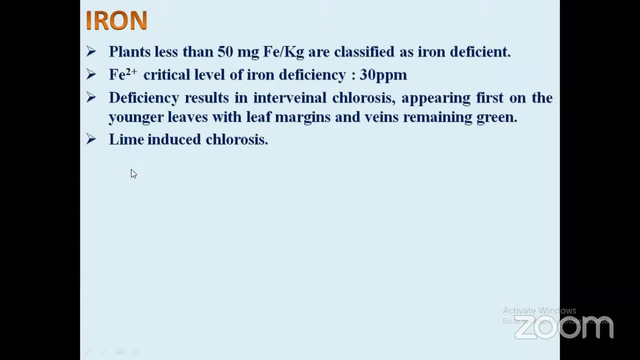 Lime is applied in acidic soil. So if lime is applied in acidic soil, that means definitely it is increasing soil pH. That is why it is applied in acidic soil. No, So because of the application of lime, the pH of the 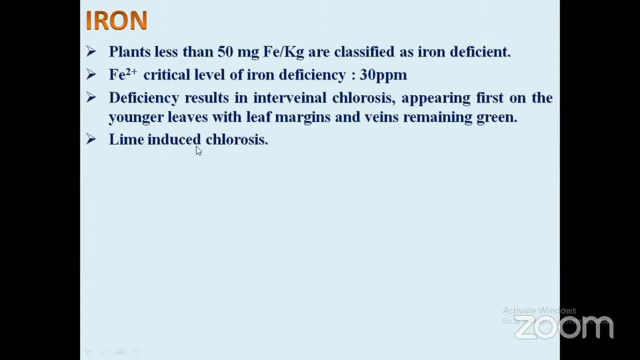 soil increases And if pH is increased, that means it is there is deficiency of this iron. I will tell you what is the effect of pH on all the micronutrients means, cations and anions. This we will see in the subsequent. 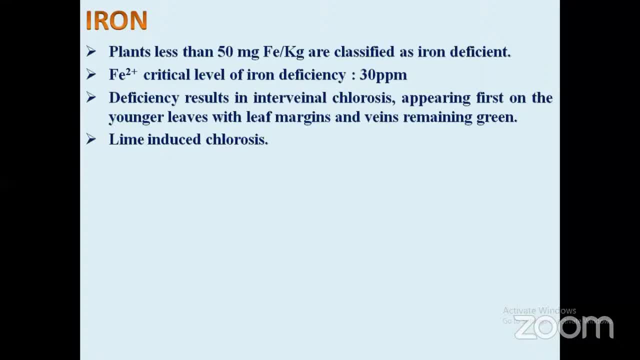 slides, But yes, for now you keep this information with you that because of the application of lime, the pH increases And if the pH increased then there is deficiency of iron And because of deficiency of iron, there is chlorosis. 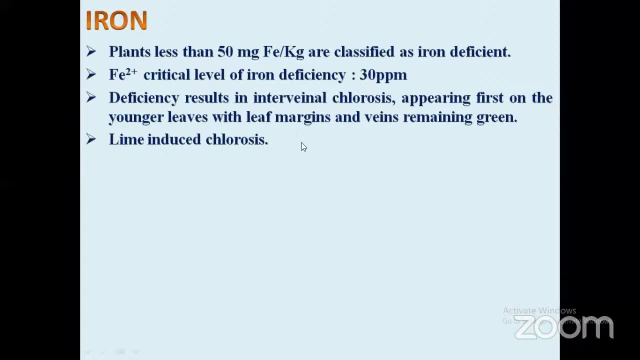 So that is why this lime-induced chlorosis is because of iron deficiency. Okay, Now moving ahead, And one more thing you can write over here. in this lime-induced chlorosis you write that soil iron concentration is high. We have seen when 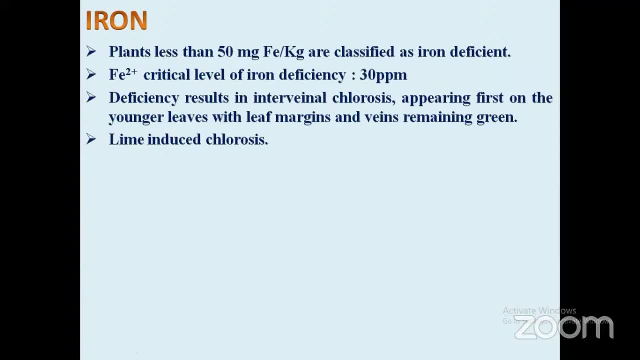 I was telling you about the concentration of these micronutrients, I told you that all the micronutrients are within the range of 100 ppm, but this- iron and manganese- there is exception that it may go up to 500 ppm also. 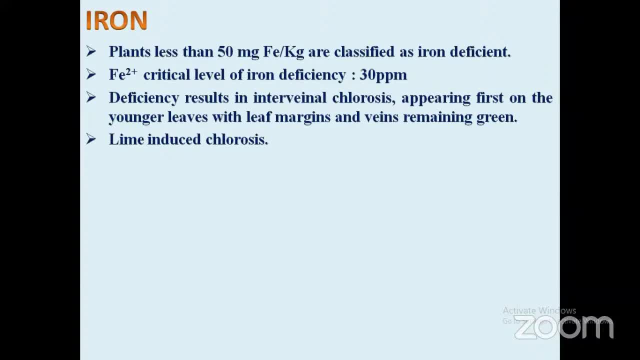 right. So soil iron concentration is high, but it can become unavailable for absorption if soil pH is higher than 6.5.. If the pH of soil is higher than 6.5, even if the concentration of iron in soil is high, 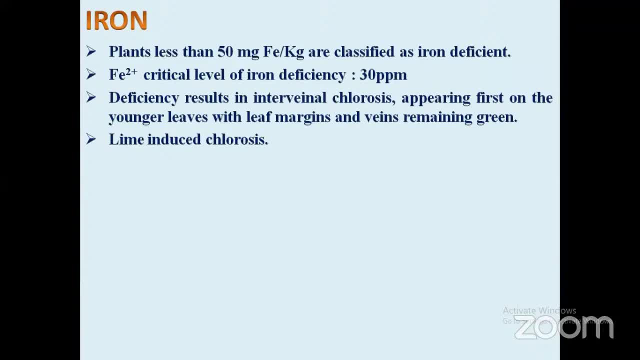 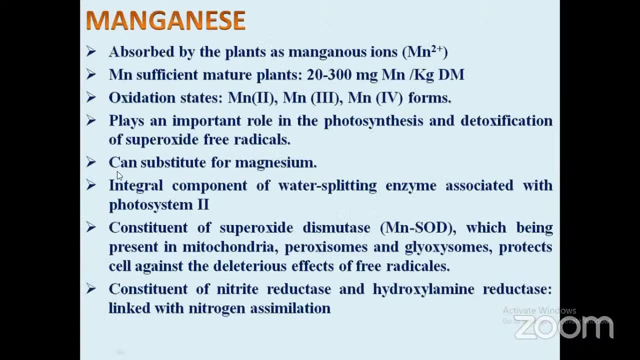 still, it will not be available to the plant. So you remember the pH more than 6.5, this iron, this lime-induced chlorosis will be there. Okay, Now moving ahead to another micronutrient cation, that is. 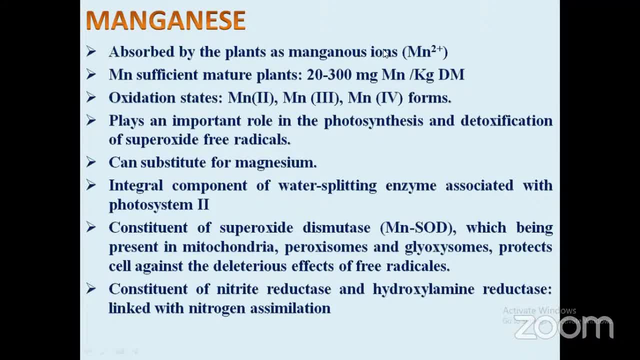 manganese, So it is absorbed by the plant as manganese form. Mn2+ and healthy manganese sufficient mature plant contains 20 to 300 ppm of manganese. It is a transition metal and it is present in plant in Mn2+ but it is 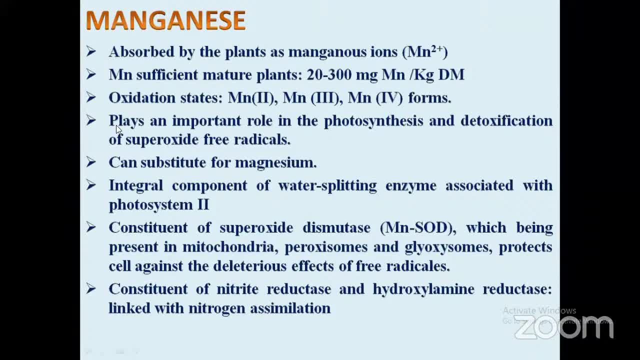 easily oxidized to Mn3 plus an Mn4 also Okay, And it plays an important role in the photosynthesis and detoxification of the superoxide-free radical. This is very important function of this manganese that it plays role in the detoxification. 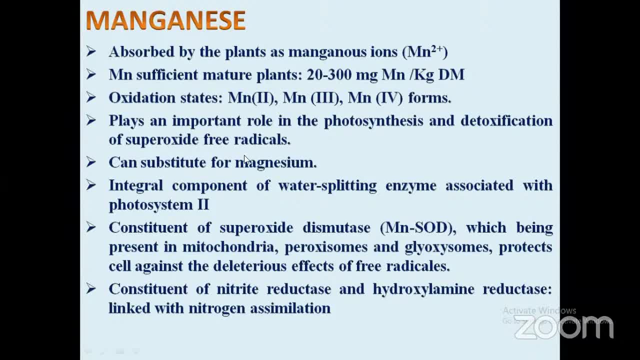 of superoxide-free radicals. Now question comes: what is this superoxide-free radical right? So you see, it is primary oxygen-free radical which is produced in the mitochondria via the slippage of an electron from electron transport chain. 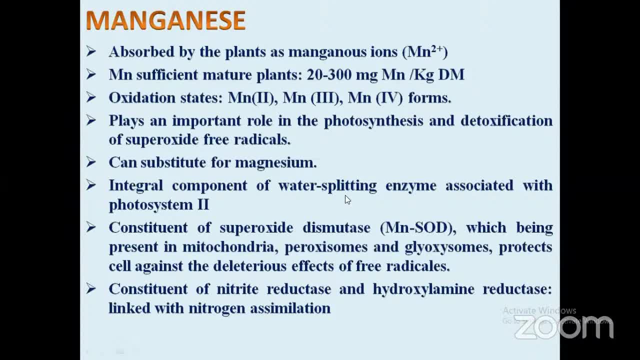 to molecular oxygen. If we have a molecular oxygen- O2, right. And if this oxygen gets an electron, then there will be O2 and there will be electron. Negative charge will be there with the oxygen, right. So this is. 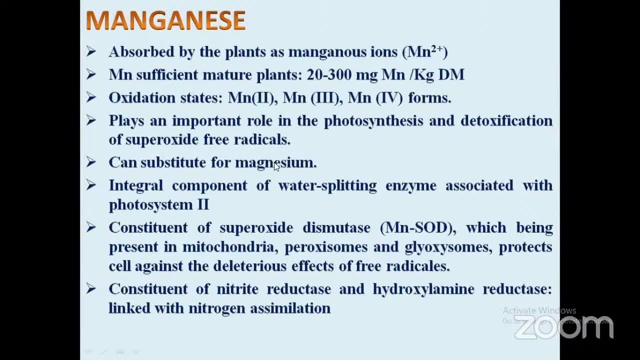 free radical, So when primary oxygen takes up the electron from the electron transport chain to become a molecular oxygen with a negative charge. this is what we call a free radical and it is unstable and it is highly reactive. So it is highly reactive. 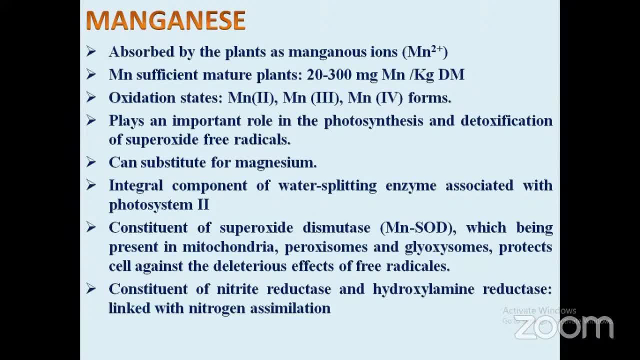 So what does it do? It reacts with the cell wall and degrade the cell. So it is very important to capture this free radical, and this work is done by this manganese. Okay, so manganese play an important role in detoxification of superoxide. 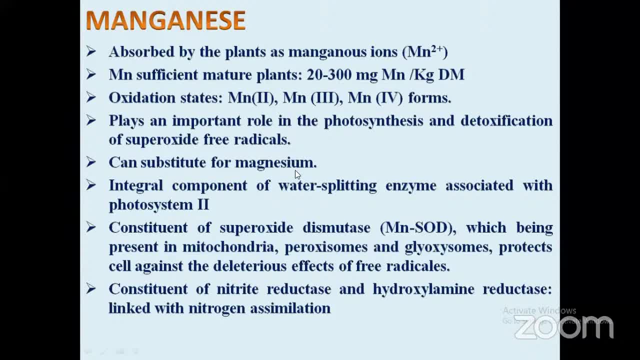 free radicals, This you remember. It can substitute for magnesium and it is an integral component of water splitting enzyme which is associated with photosystem 2.. This is also very important question very frequently asked in exam: that which of the following micronutrient? 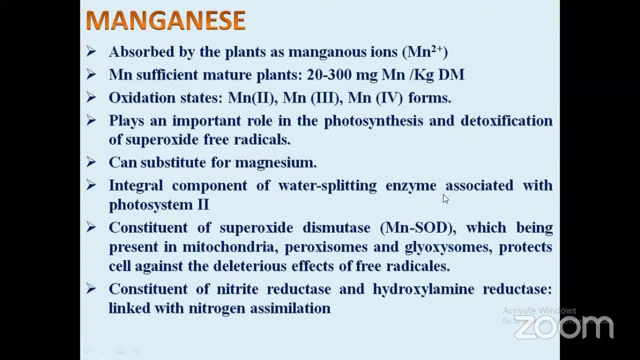 or which of the following element is a component of water splitting enzyme which is associated with photosystem 2. So it is manganese, As we have seen that it of superoxide dismutase. So it is manganese: SOD superoxide dismutase. 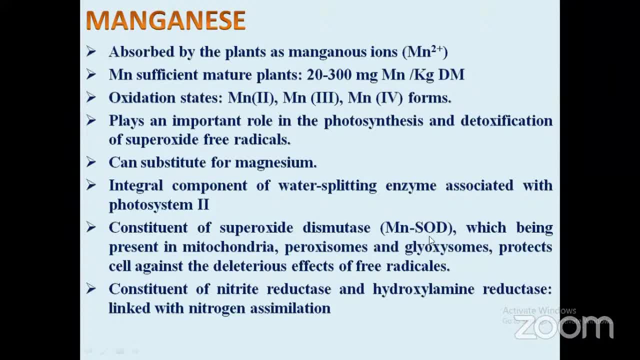 which being present in. it is also asked in exam that manganese, SOD, manganese superoxide dismutase- is present in which cell organelle? So it is present in mitochondria, peroxisomes and glyoxisomes. Whatever way you want to. 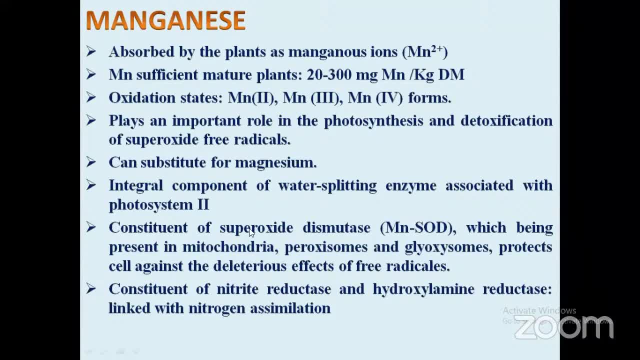 remember, you remember this one: Manganese SOD in mitochondria, peroxisomes and glycosomes, and it protect the cell against the deleterious effect of free radicals. It is a constituent of nitrite reductase and hydroxylamine. 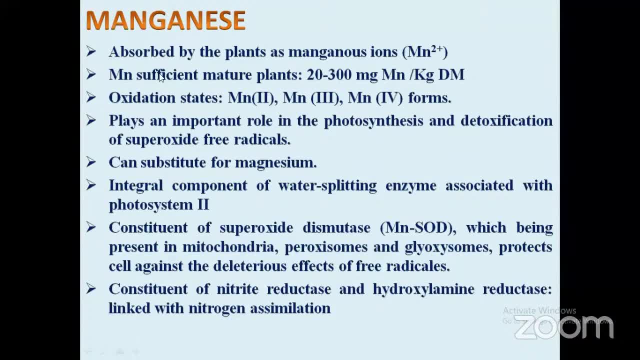 reductase and hence it is linked with nitrogen assimilation. So manganese is a constituent of nitrite reductase, hydroxylamine superoxide, dismutase, water splitting enzyme. These are the important functions of manganese. Now 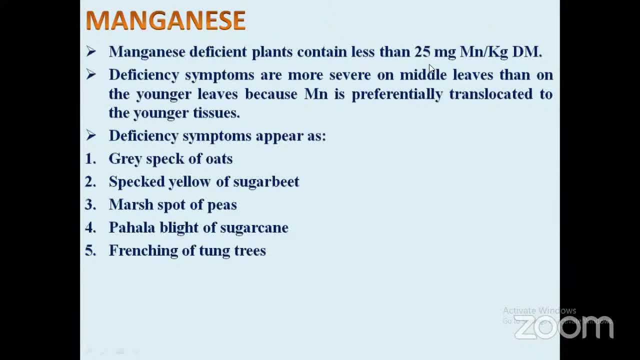 moving ahead. Manganese deficient plants contain less than 25 ppm of manganese. So if it is less than 25 ppm, it is more severe on the middle leaves than on the younger leaves, because manganese is preferentially translocated to the younger leaves. 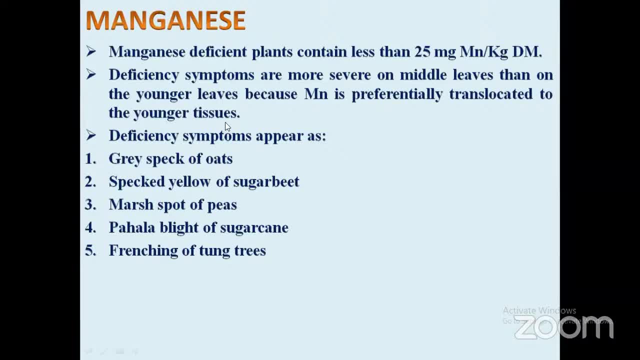 This is a mobile element in the plant so it moves to the younger leaves and hence its deficiency is not seen on the younger leaves, like iron, So its deficiency is seen on middle leaves. These are the common deficiency symptoms of manganese. This you may 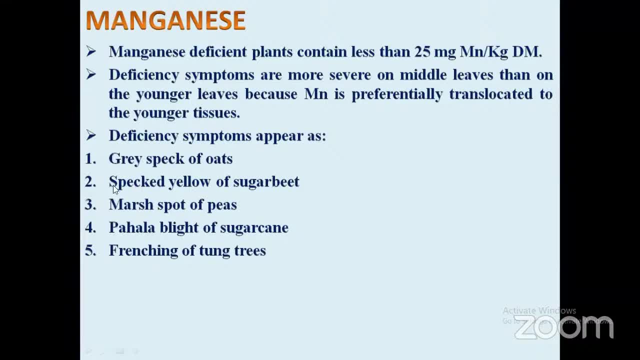 find very frequently in exams: Grey speck of oat speck, yellow of sugar beet, marsh spot of peas, pahala blight of sugar cane and frenching of tongue cream. So these are the deficiency symptoms of manganese Okay. 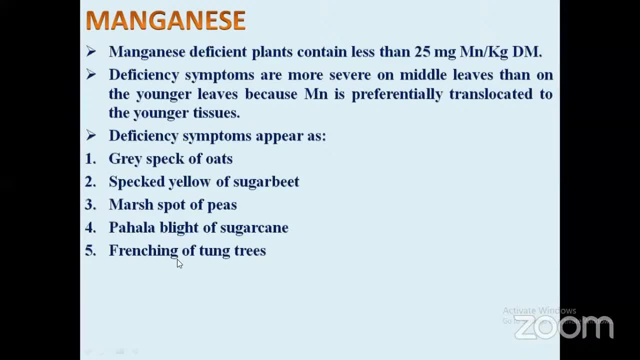 if anyone of you want to tell me what do we understand by this frenching, Anyone? Okay, fine, Abhi next slide mein batati hum mein frenching means kya. But for now you keep this information with you, that frenching of. 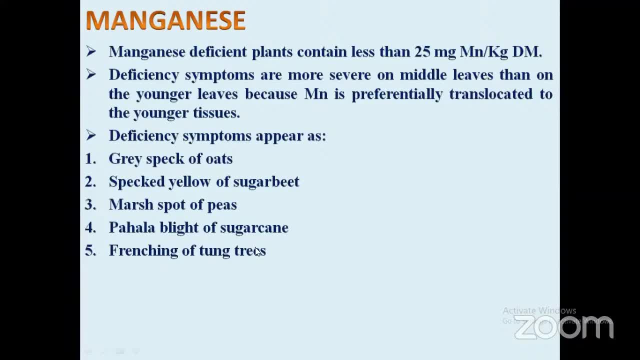 tongue trees. Next we'll see frenching of citrus. that is because of different micronutrients. So frenching of tongue, frenching is actually mottling. Okay, there is variegated some part of the leaf, there is another color, some. 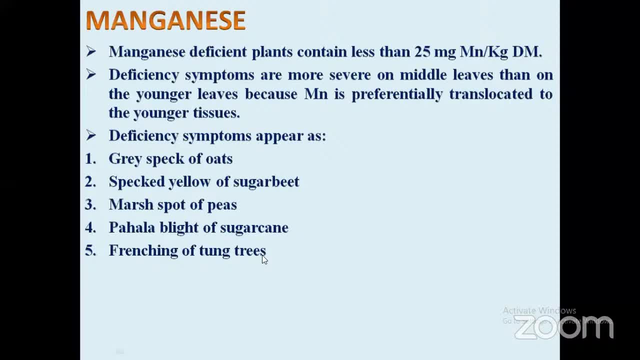 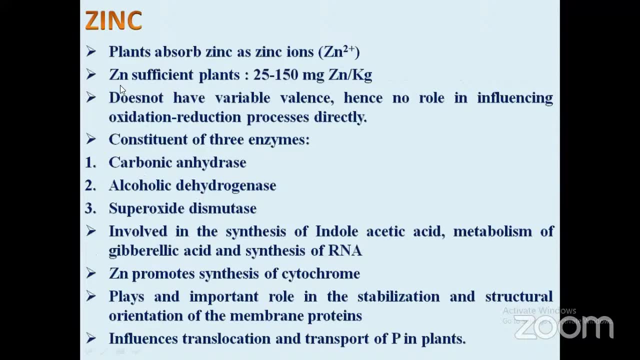 part of the leaf is having another color, that is mottling. So frenching of tongue trees is because of manganese. Okay now moving ahead to another micronutrient, that is zinc. So plant, take up zinc as Zn2 plus. 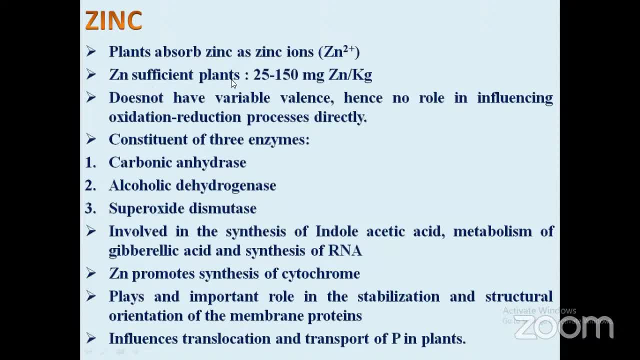 ion and the zinc sufficiency content in plant is 25 to 150 BPM and the zinc does not have variable valence. It is only Zn2 plus. Hence no role in influencing oxidation reduction processes directly. It does not influence oxidation means. 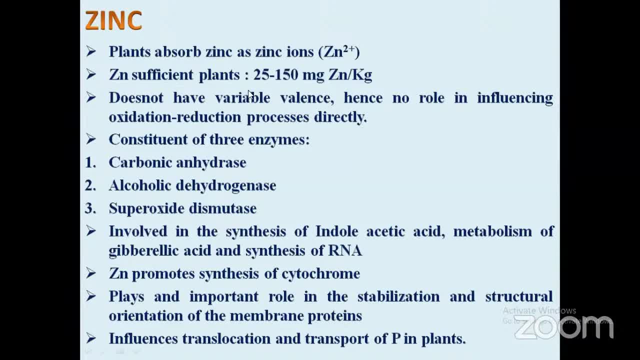 reduction processes directly because it does not have any variable valence. It is constituent of three enzymes: carbonic anhydrase, alcoholic dehydrogenase, superoxide dismutase. You see superoxide dismutase. we have seen in manganese also. So 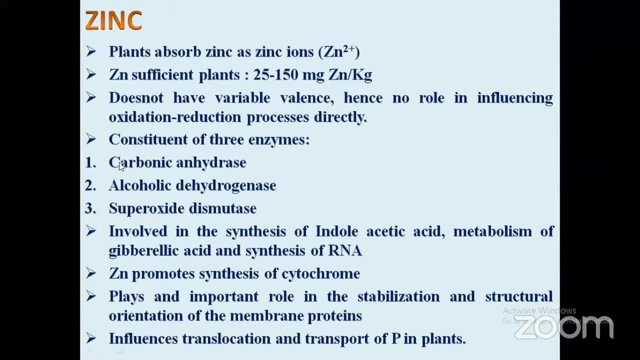 that was manganese SOD. This is zinc SOD. Okay, so carbonic anhydrase, alcoholic dehydrogenase, superoxide dismutase. the constituent of these enzymes is zinc, and zinc is involved in the synthesis of indole acetic acid metabolism. 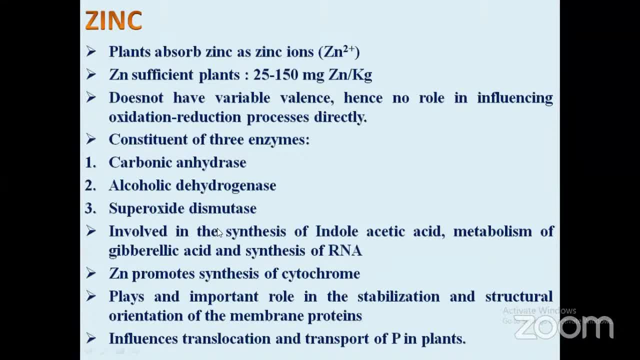 of gibralic acid and synthesis of RNA. Very important function of zinc that it is involved in the synthesis of indole acetic acid. This is auxin. So if there is deficiency of zinc that means there is less auxin, and if 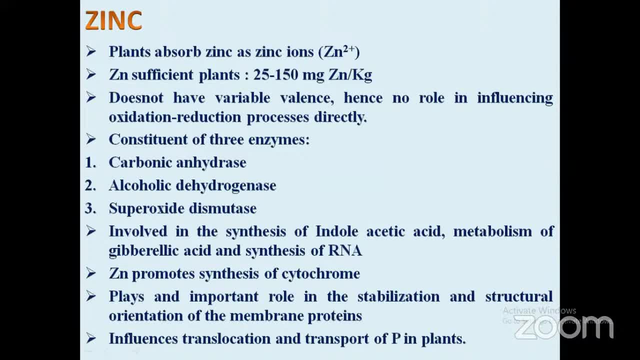 auxin is less, the leaves or the cell will not grow. So because of the deficiency of zinc, the leaves are little, very small. small leaves are there and it form a bushy like structure. This is what we call rosette structure. This 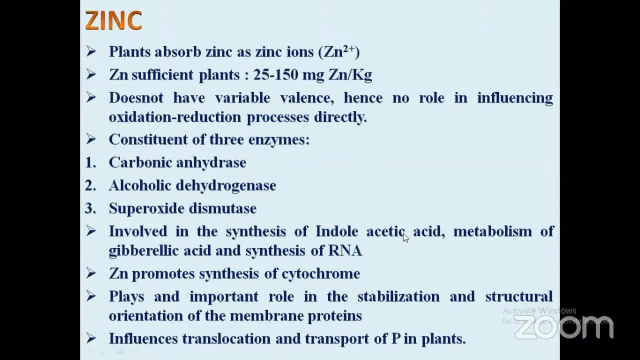 is because of the problem in the synthesis of indole acetic acid because of the deficiency of zinc. So zinc is involved in the synthesis of indole acetic acid, metabolism of gibralic acid and synthesis of RNA. Zinc promotes synthesis of 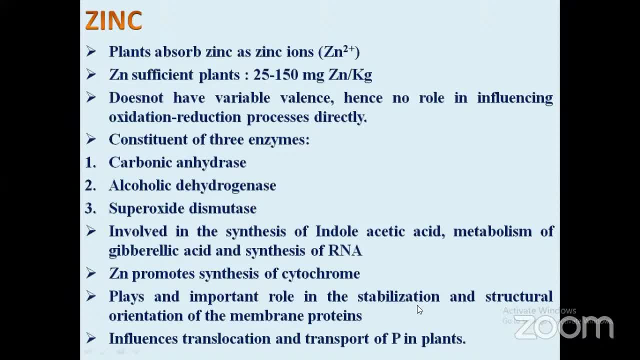 cytochrome also, and it plays an important role in translocation and transport of phosphorus in the plant. You tell whether zinc and phosphorus are synergistic in nature or antagonistic. Zinc and phosphorus: very frequently asked in exam. they are antagonistic. 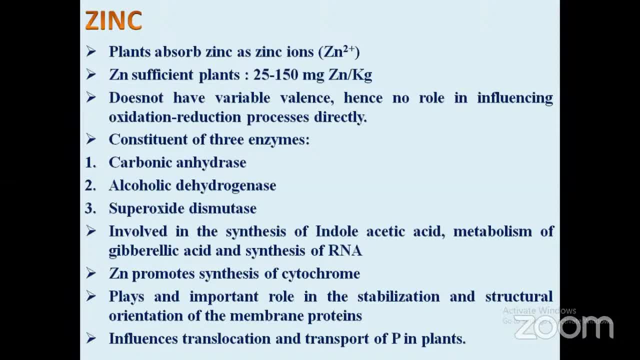 and under zinc deficiency. excessive translocation of phosphorus results in the phosphorus toxicity. If there is deficiency of zinc, definitely phosphorus will be more and there can be phosphorus toxicity also. Now zinc deficiency. you see, if the plant contains less than 15, 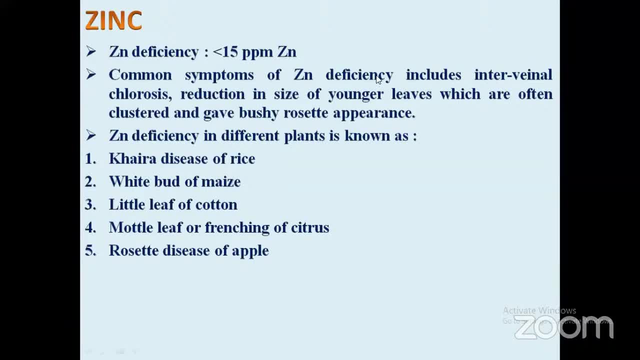 ppm of zinc, then it will be deficient, and common symptoms of zinc deficiency includes intervenial chlorosis, reduction in the size of the younger leaves, as I told you, which are often clustered and gave bushy rosette appearance. this is because of the less indole. 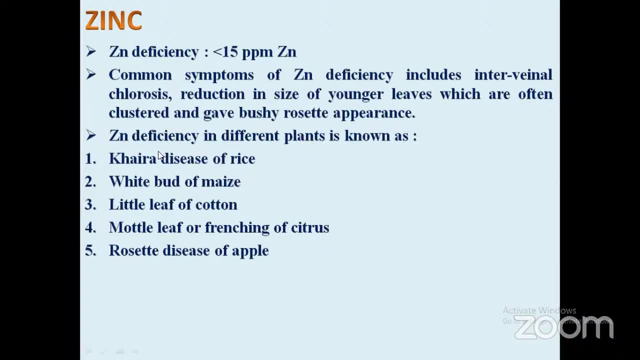 acidic acid production because of zinc deficiency. different means. zinc deficiency in different plant is known by different names. these are used to ask this disease of rice is because of zinc deficiency. it was discovered. by whom? you tell in different ways. this disease is usually asked this is due. 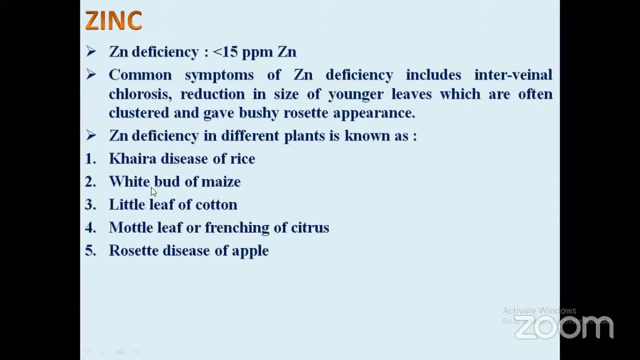 to zinc deficiency discovered by another. is little leaf of cotton, frencing is mortal leaf only. frencing of tongue trees was because of the manganese right and frencing of citrus is due to zinc deficiency. that is why I emphasized more on frencing. 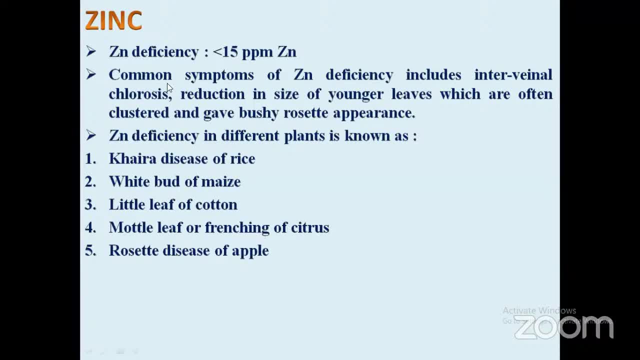 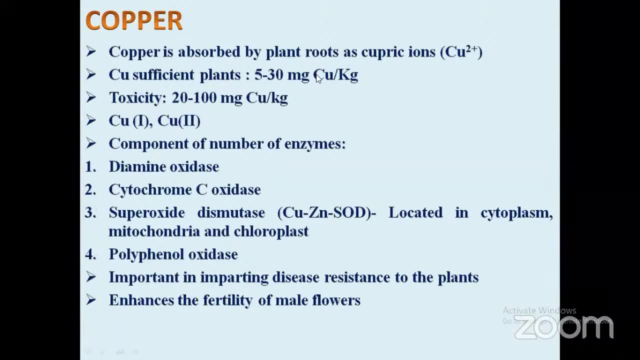 in last slide, so that you remember frencing of citrus because of zinc deficiency, frencing of tongue trees because of manganese deficiency. another is rosette disease of apple. now, moving ahead to another micronutrient cation, that is copper. so copper is absorbed. 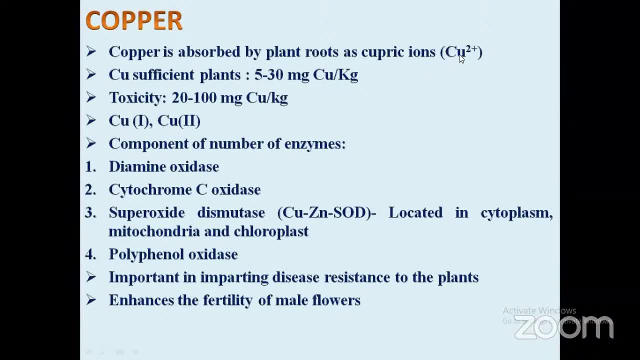 by plant roots as cupric acid, cupric ion sufficient plants. if they contain copper between 5 to 30 ppm, then they are sufficient, and if it is between 2200 ppm, then it is toxic to the plant. copper exists as cu plus and cu 2. 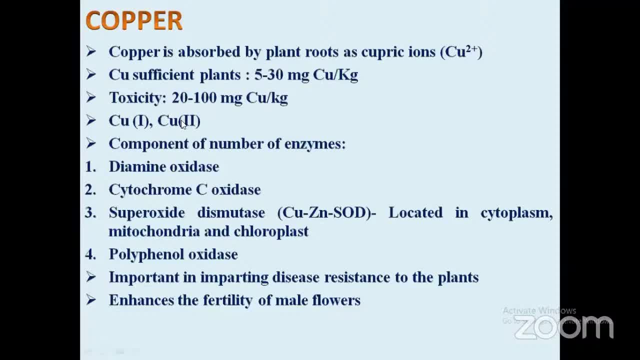 plus. so this is cupric form, this is cupric form plant. take up this cu 2 plus cupric form and this copper is a component of number of enzymes like diamine oxidase, cytochrome oxidase, superoxide dismutase, zinc, SOD. 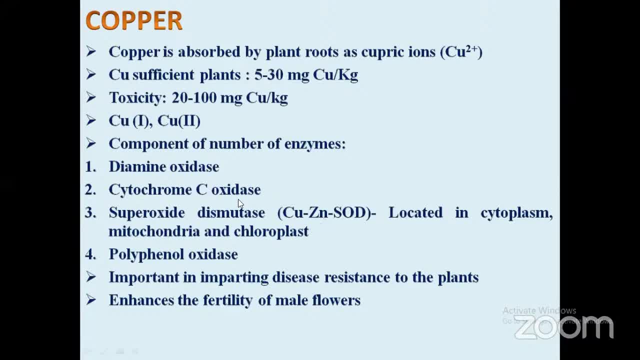 we have seen. so this copper and zinc SOD- they are together actually. so copper- zinc superoxide dismutase. this is located in cytoplasm mitochondria and chloroplast. I am emphasizing this again because they use in objective question. they used to ask what is. 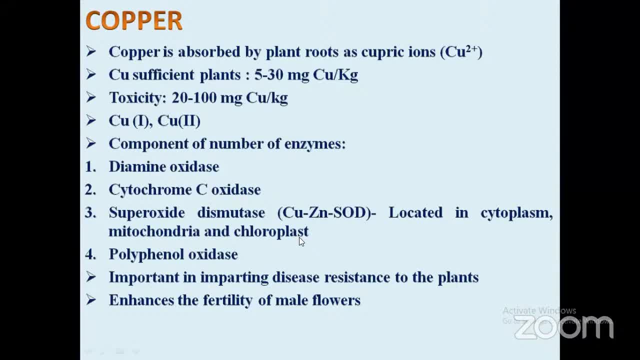 means where is this super magnesium superoxide dismutase present- three organelles, I told you- and this copper zinc, SOD is present in another three organs that are cytoplasm, mitochondria and chloroplast. so this is important. you remember this. it is also 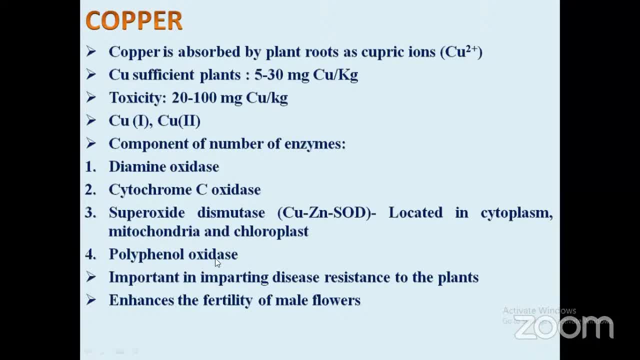 a component of polyphenol oxidase. this copper is a component of polyphenol oxidase which is involved in lignin biosynthesis. you write this polyphenol oxidase is involved in lignin biosynthesis, so it can be asked in exam directly that. 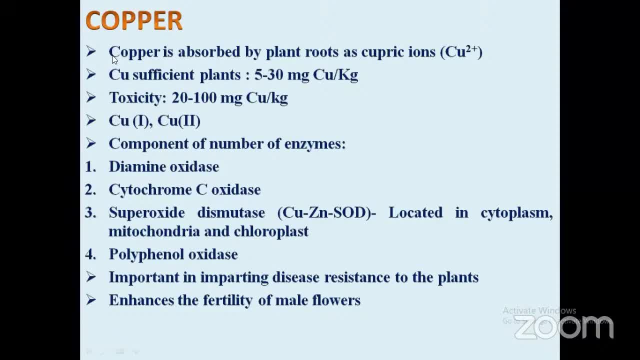 which of the following element plays role in lignin biosynthesis? it is copper. it is important in imparting disease resistance to the plant. this copper is a micronutrient that is important in imparting disease resistance to the plant. if I ask you which of the 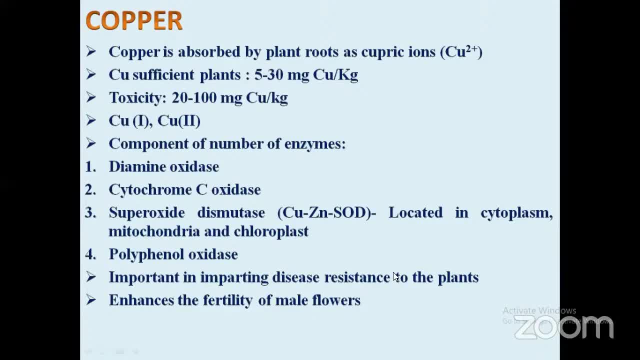 macronutrient impart disease resistance to the plant. you tell potassium, potassium, wonderful. so in micronutrient it is copper that is imparting disease resistance and in macronutrient it is imparting disease resistance to the plant. this copper enhances the fertility of the 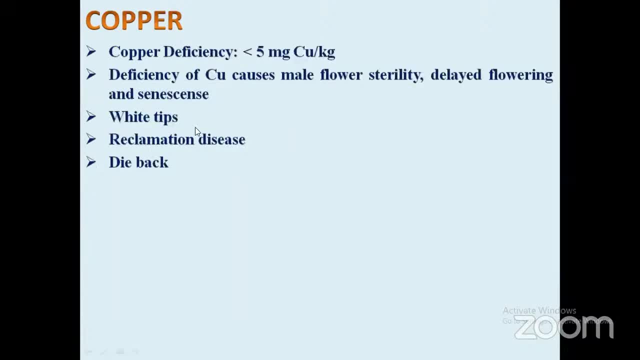 male flowers also. another is: if the plant contains less than 5 ppm of copper then it is deficient and the deficiency of copper causes male flower sterility, delayed flowering and senescence. another symptoms or another disorders because of this copper deficiency are white tip reclamation. 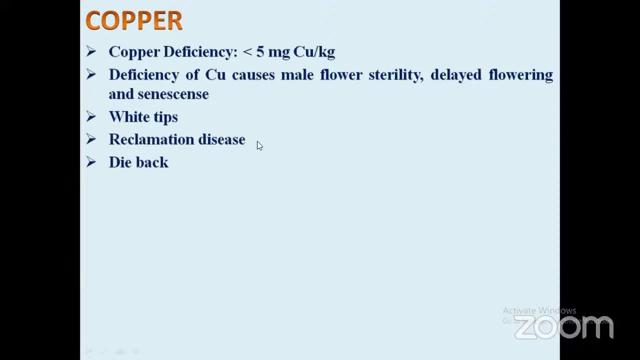 disease and diabetes. so this is very frequent question in exam that reclamation disease is caused by which of the following element deficiency? so it is copper. so what is this reclamation disease? anyone of you want to tell? you must have heard that copper deficiency causes reclamation. 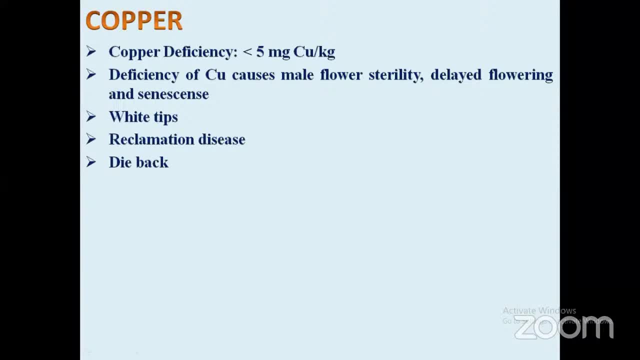 disease. so what is this reclamation disease? reclamation means try, sir. is there anything which is has to be improved? ok means if anyone reclaims reclamation for anything. if it is reclamation for anything, then will it become copper deficiency or or any particular specific reclamation. 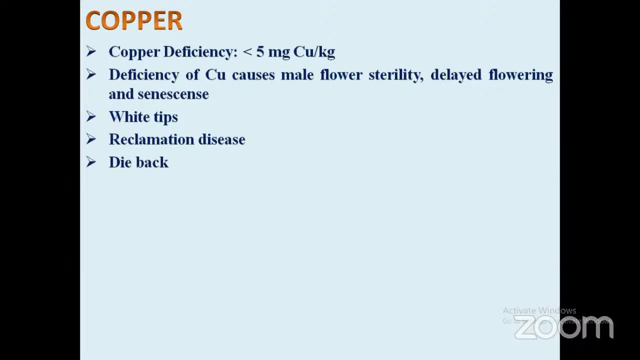 or reclamation of sodic soil. ok, one is saying sodic soil yes. another one you say: when we apply calcium in acidic soil, it increases its deficiency of copper, forms the deficiency of copper. If the pH increases, then all the micronutrients should be deficient. 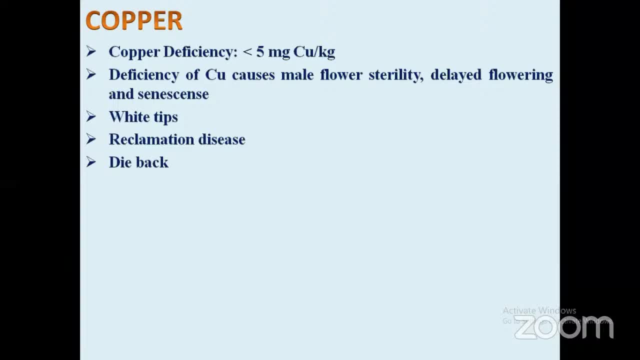 So should we call it a reclamation disease for all the micronutrients? You are thinking right, Everyone is thinking right. I didn't think a little bit about sodic. If pH increases by adding lime to acidic soil, then it will become copper deficient. 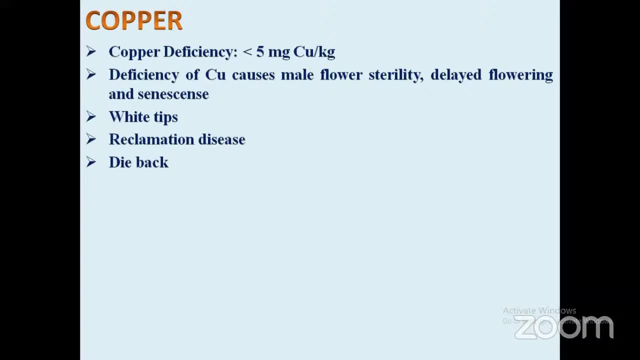 That is very correct. But this reclamation disease- it is a name given because this copper is having very high affinity for organic matter. If we add FIM to any soil for reclamation, all of you understand Hindi, right? Yes, ma'am. 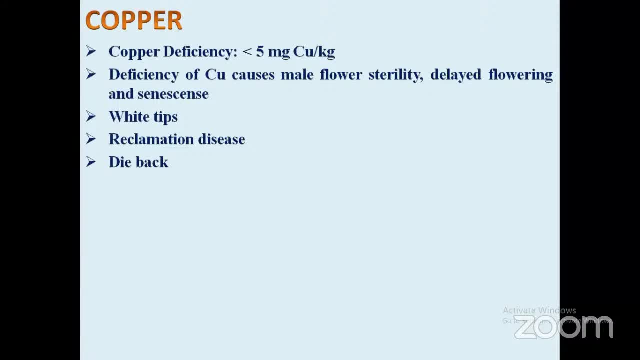 So if we add FIM to any soil for reclamation, we add organic source and this copper is having very high affinity for organic matter. So if we add FIM then all the copper gets bind in it and because of that copper deficiency- 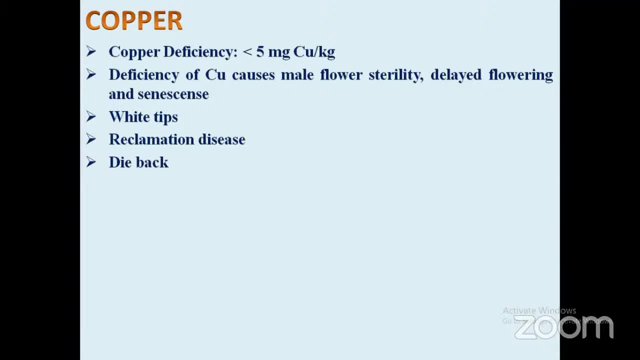 is happening. So this specifically is said for copper, Because copper, Copper is having high affinity for organic matter, right. So reclamation disease: it is a disorder that affects crop growth on reclaimed land, which is caused by the deficiency of elements like copper. 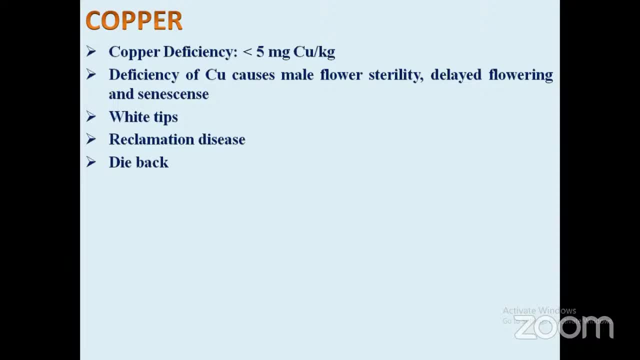 Making sense to all of you. Yes, ma'am, Now moving ahead. Ma'am, please repeat. Okay, You see, reclamation disease means we are reclaiming any soil. If there is any problem in it, we correct it. 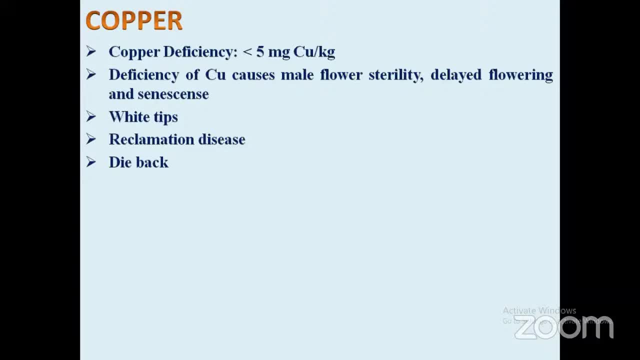 Okay, And because of correcting, copper gets deficient. So if we add FIM to any soil or any organic matter, then copper is very easily very tightly bind to this organic matter because copper affinity is more for organic matter. It is having high affinity for organic matter. 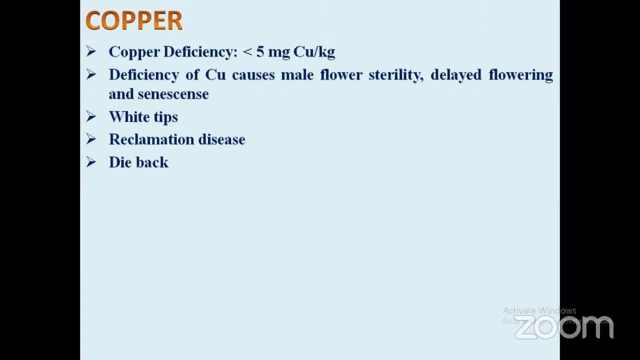 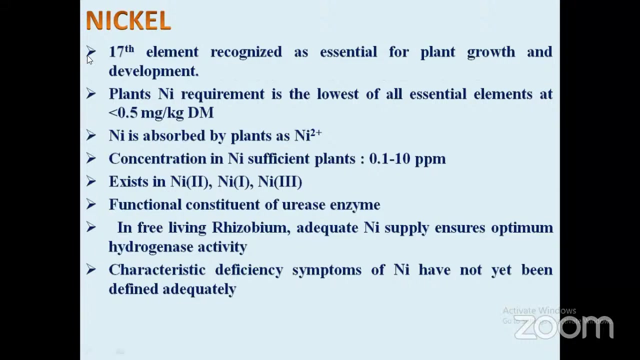 So we added FIM to soil. copper got bind to FIM and plant didn't get it, Because of which copper deficiency happened. way making sense? yes, thank you. now moving ahead to another element, that is nickel. so this is the 17th element recognized as essential for the plant. growth means the latest essential element. 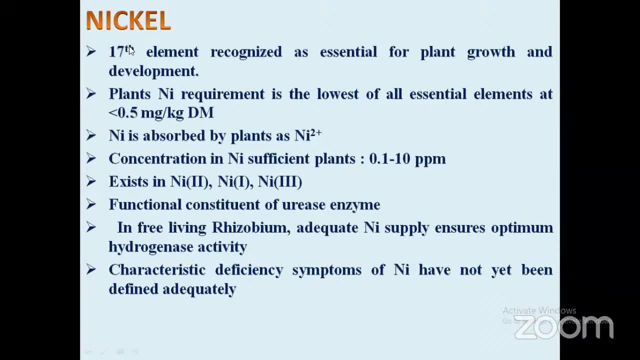 who has discovered the essentiality of nickel? anyone of you brown, 1987. do you know the other names of brown brown? anyone of you brown will carry brown welch and carry carry wonderful. and year: 19, 87, 1987. yeah, why i am emphasizing this? because sometimes we all know when we have started this essentiality. 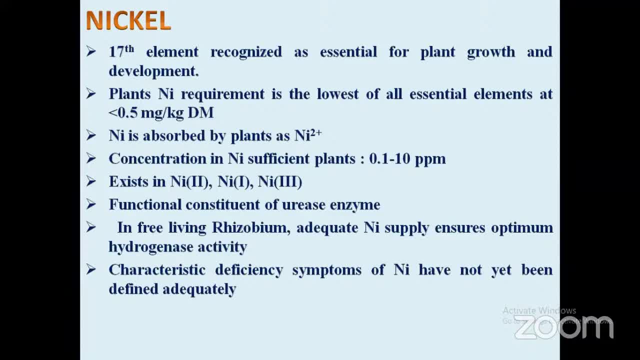 who has given the essentiality of particular nutrient. so we only study one scientist, but if the objective question is that he is a nuclear scientist, then he is a nuclear scientist. if there are two scientists in one option, then what will we do if there is an option of all or both? 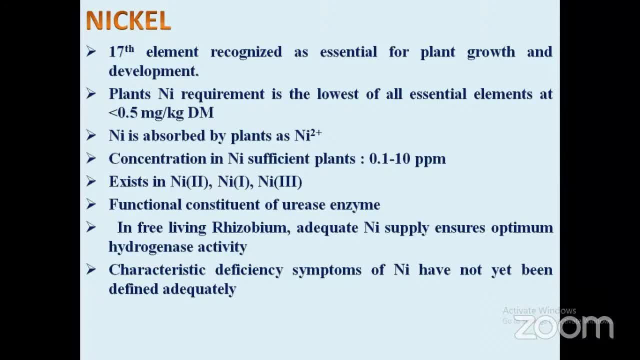 so even if we keep one name, but it is necessary to see everyone's name once. okay, so nickel essentiality: it is the latest micronutrient that is being recognized as essential element by brown, welch and carey in 1987, and plant nickel requirement is the lowest of all the essential element that is less than 0.5 ppm. nickel is a. 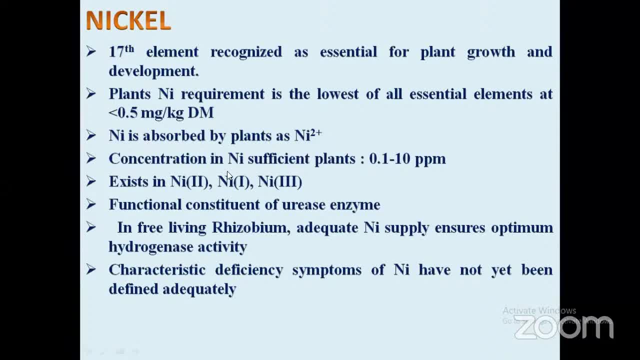 the lowest of all, the essential element that is less than 0.5 ppm. nickel is a absorbed by the plant as ni2 plus. this nickel exists in an i2 plus form, but it can also assume ni plus ni3 plus form also okay, and the concentration of nickel in means the 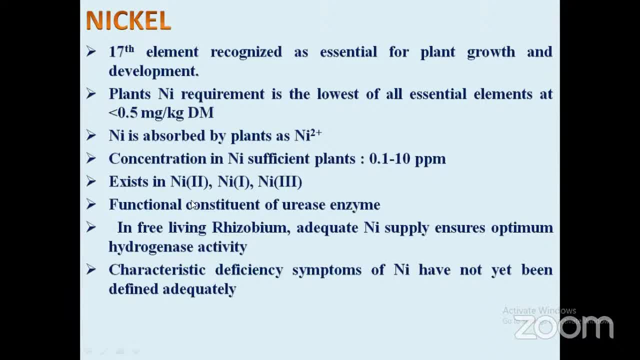 sufficiency range of nickel in plant is 0.1 to 10 ppm. this nickel- very important question- that it is a functional constituent of urease enzyme. this urease enzyme is involved in which process some urea hydrolysis. yeah, so this is a functional constituent of urease enzyme. 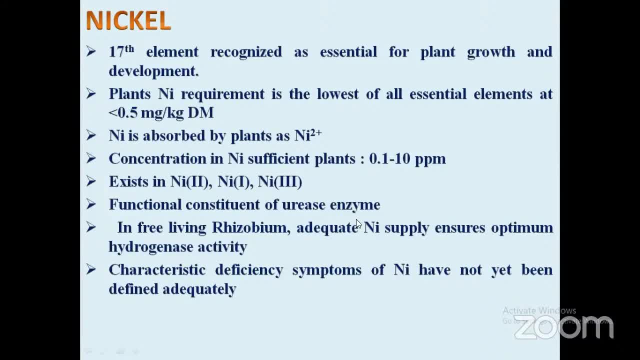 some urea hydrolysis. yeah, so this is a functional constituent of urease enzyme and this nickel is actually a cofactor. you remember that nickel is a cofactor that enables the urease to catalyze the conversion of urea into the ammonium ion. 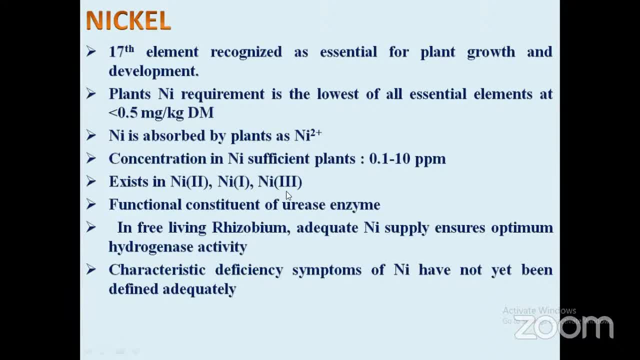 this is a functional constituent. it is not saying that nickel is a constituent of this urease enzyme. this nickel helps in functionality of this urease enzyme because it acts as a cofactor. okay, so nickel act as a cofactor and helps in conversion of this urea. smaller equal to 90% travel time. 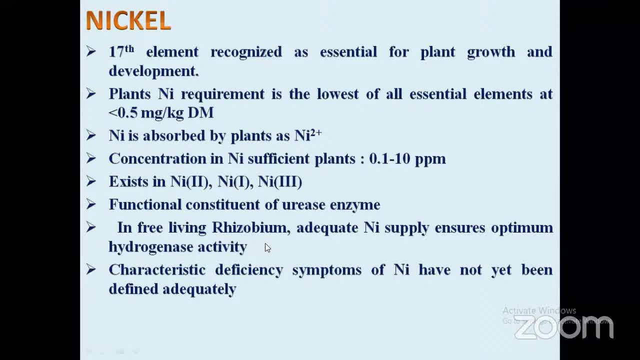 of uea into the ammonium ion and in free living rhizobium. rhizobium is bacteria or fungus, bacterium, yeah. so in free living rhizobium, adequate nickel supply ensures optimum hydrogenase activity. so if there is optimum nickel, so it ensures hydrogen, good hydrogenase. 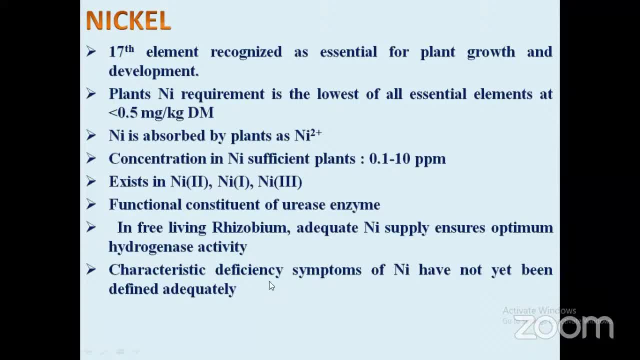 activity in rhizobium. characteristic deficiency symptom of nickel have not been defined adequately. but yes, if in a system where urea is used as a sole nitrogen fertilizer- okay, you see there is in soil- we are applying urea as a single source of nitrogen fertilizer for foliar spray. 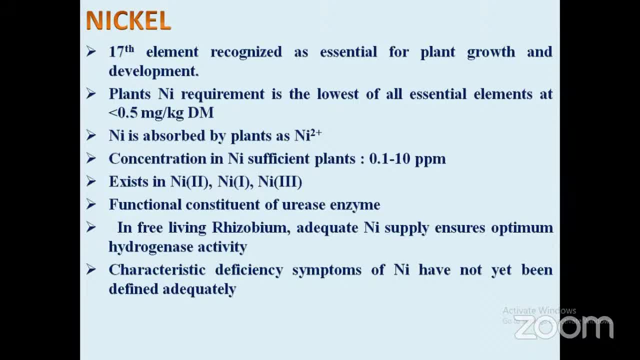 and nickel supply is poor in soil, then what will happen? no ma'am, no. so in the system we are applying urea as a single source of nitrogen fertilizer for foliar spray and nickel supply is poor, then lower urease activity causes urea toxicity to the foliage. 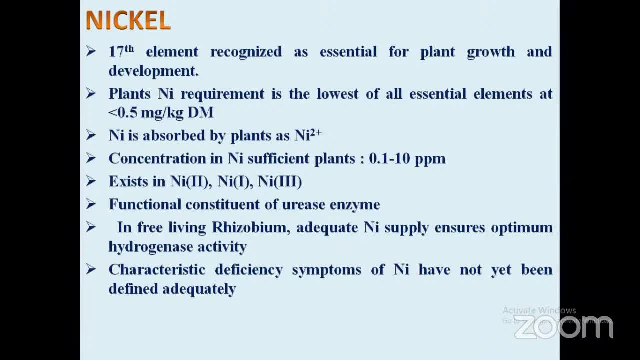 urea urease kaam nahin karega agar nickel nahin hai toh or urea convert nahin ho pahega ammonium form mein. so plant is not going to take that urea but there will be urea toxicity to the. 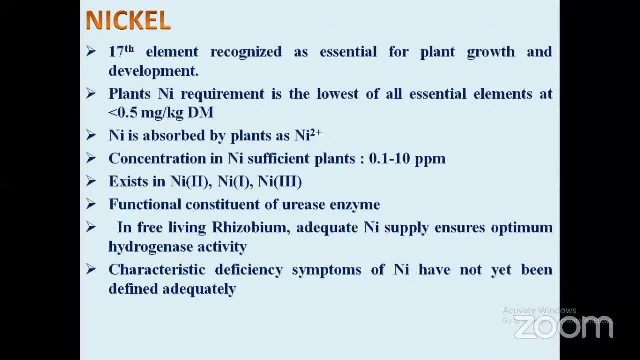 foliage because of the lower activity of urease and this leads to severe necrosis of the root. so if nickel is deficient in the plant and we are applying urea as a source of nitrogen, then there will be toxicity of the urea and this leads to severe necrosis of the root tips. 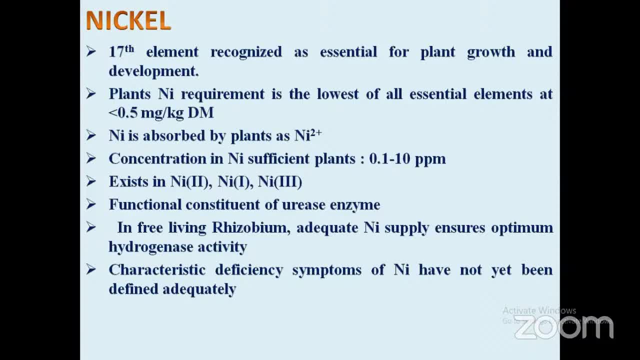 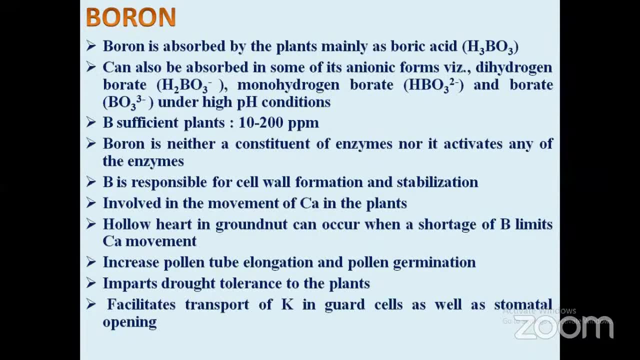 making sense to all of you. yes, yes, ma'am, yes, ma'am. okay, now moving ahead to another micronutrient, that is boron, which is taken up by the plant in cationic form or anionic form. you tell neutral form, neutral form. so boron is taken up by the plant mainly as boric acid, s3bo3, and can also 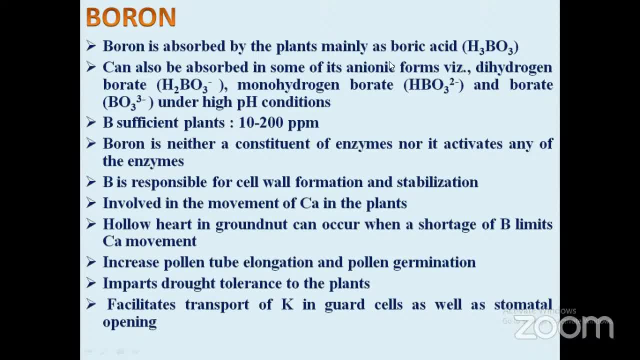 be absorbed in some of its anionic form also. okay, usually it is taken as boric acid, but yes, we can keep this boron in anionic form of micronutrient also because it is absorbed in some of its anionic form. one is dihydrogen borate, monohydrogen borate and borate under high ph conditions. 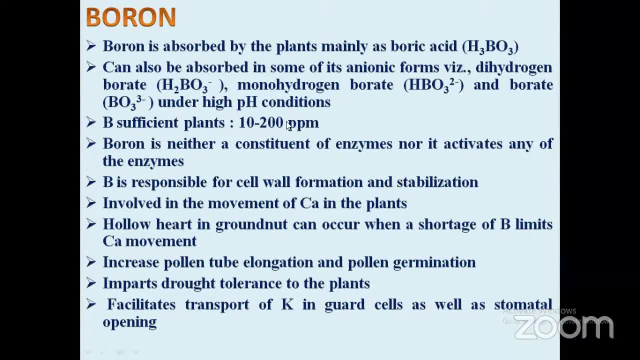 and boron sufficient plants contain 10 to 200 ppm of boron and you see, boron is neither a constituent of enzyme nor it activates any of the enzymes. so boron is not involved in any enzymatic activity, unlike any other micronutrient. so boron is neither a constituent of any enzyme nor it activates any. 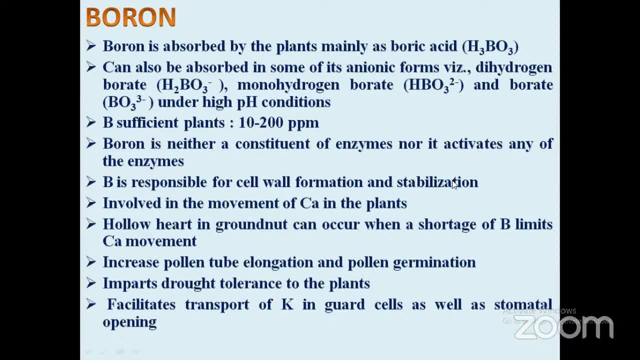 enzyme. it is responsible for cell wall formation and stabilization and this boron is involved in the movement of calcium in the plants. so boron is involved in the movement of calcium in the plants and hollow heart in ground nut can occur when the shortage of boron limits calcium movement. so if 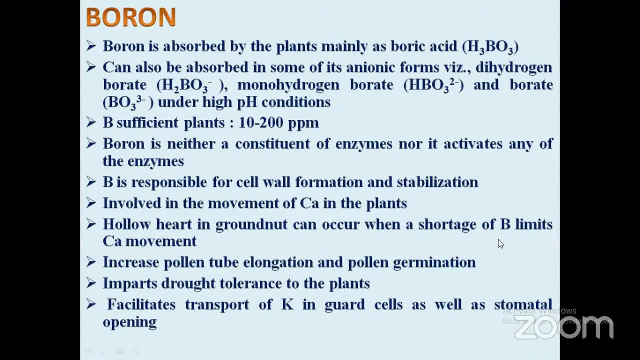 there is means deficiency of boron, then this deficiency of boron may also lead to deficiency of calcium and hollow heart in ground nut. this is because of shortage of boron that limits the calcium movement. okay, and this boron is involved in pollen tube elongation and 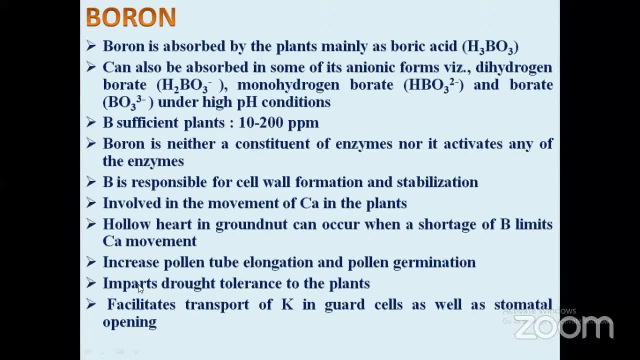 pollen germination. and, and you see, i have told you that because of the boron deficiency, there is deficiency of calcium, right? so you see, if there is boron deficiency in the plant, then there is decrease in the production of indole acetic acid. this boron is also involved in production of 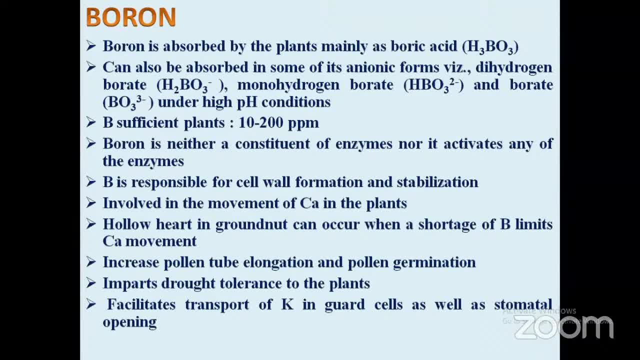 indole acetic acid, iaa. okay, so if there is deficiency of boron, there is decrease in the production of indole acetic acid, and this decrease in the indole acetic acid is responsible for the induction of calcium deficiency. so you remember that boron is involved in indole. 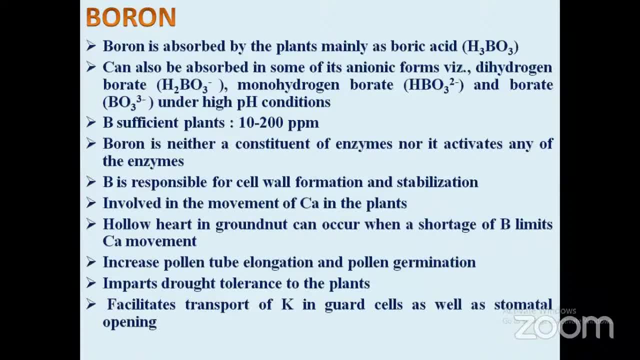 acetic acid production and because of deficiency of boron there is less indole acetic acid and because of that calcium deficiency is there. this boron imparts drought tolerance to the plant. so if i ask you, any macronutrient that impart drought tolerance to the plant? 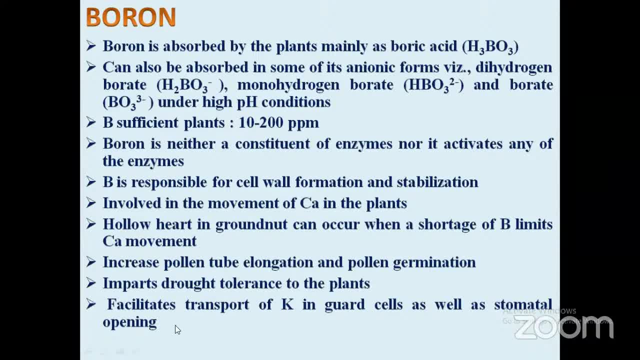 yes, macronutrient. so this boron also imparts drought tolerance to the plant and it also facilitate transfer transport of potassium in the guard cell as well as the stomata opening. so if, if we are saying that boron impart drought tolerance to the plant, that means 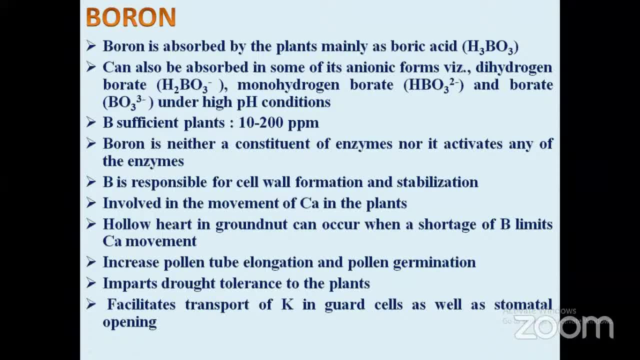 regular boric acid spray will help in mitigating harmful effects of drought. so questions can be asked this way also: that which of the following spray would help in mitigating harmful effects of drought? so it is boric acid spray, because this boron is having the property that 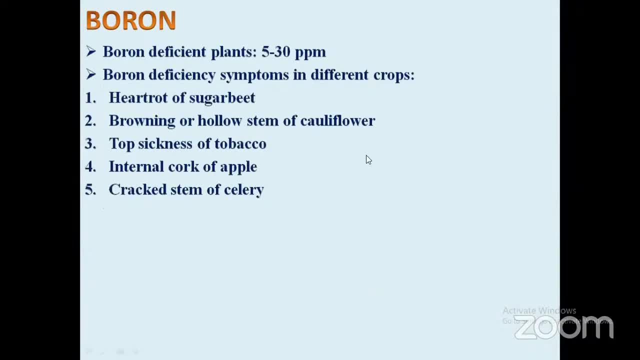 impart draw tolerance to the plant. okay, now moving ahead to the concentration of boron in the plant that causes the deficiency. that is 5 to 30 ppm. if it is less than this range, then there will be deficiency of boron, and boron deficiency symptoms in different crops are heart rot of sugar beet. 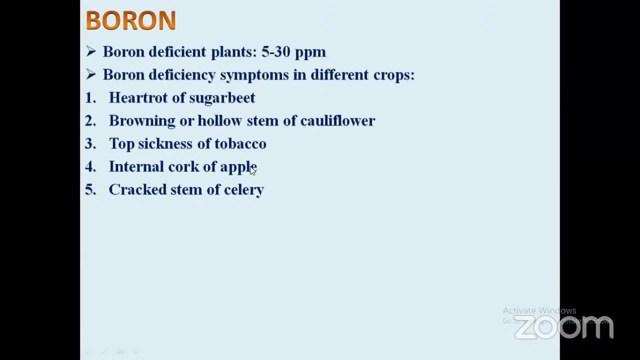 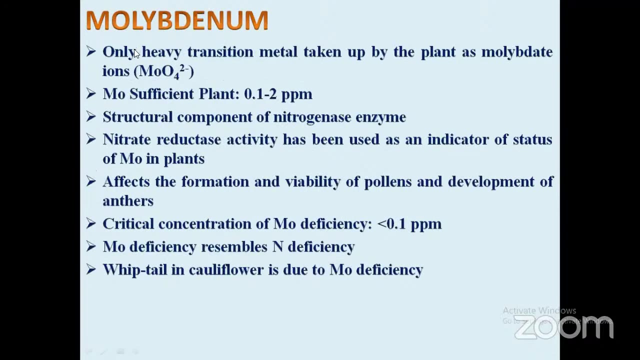 browning or hollow stem of coir, cauliflower, top sickness of tobacco, internal cork of apple, cracked stem of celery. i have tried to incorporate those deficiency symptoms that are very frequently asked in exams. so Oke, thyaane se dekhna. now moving ahead to another micronutrient, molybdenum, which is actually a anionic. 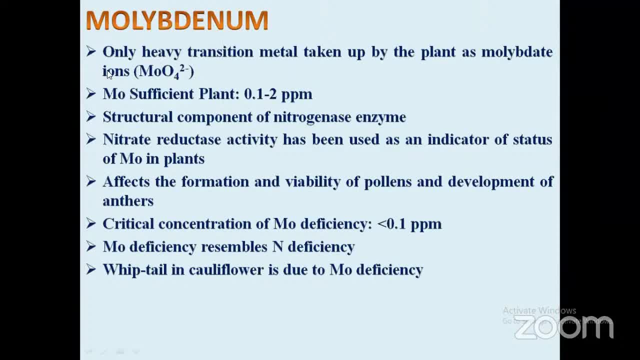 micronutrient. so molybdenum is the only heavy transition metal. so, out of all the elements, this is heavy metal, right, molybdenum. so it is the only heavy transition metal which is taken up by the plant as molybdenum, and the sufficient range is 0.1 to 2 ppm. if it is this, much amount is present. 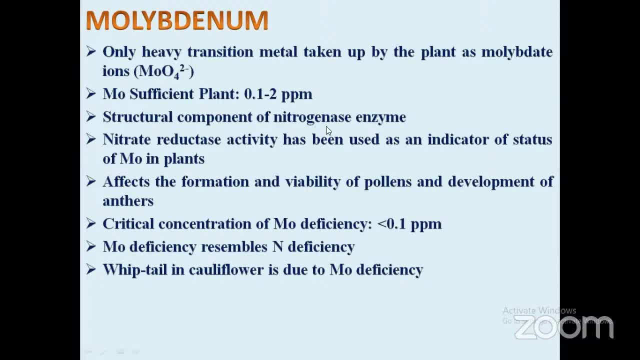 in the plant, then it is sufficient and it is structural component of nitrogenase enzyme. this molybdenum is a structural component of nitrogenase enzyme. before that, you see, i told you that plant take up molybdenum in mo for 2 minus form, this molybdate ion, but in the plant 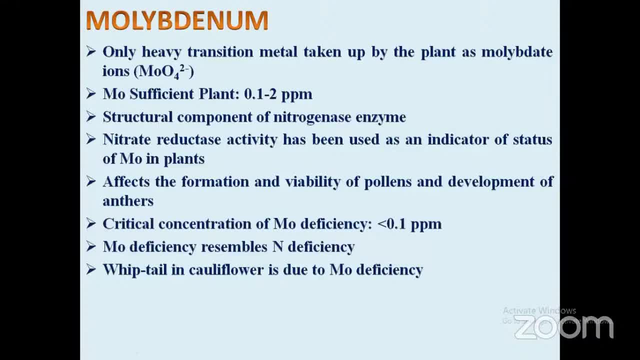 system. under oxidative environment it may exist as molybdenum 6. you write mo 6 plus 6 minus sorry, and also it undergoes reduction to mo 5 also, so valency can take up this minus 2 minus 6 and minus. 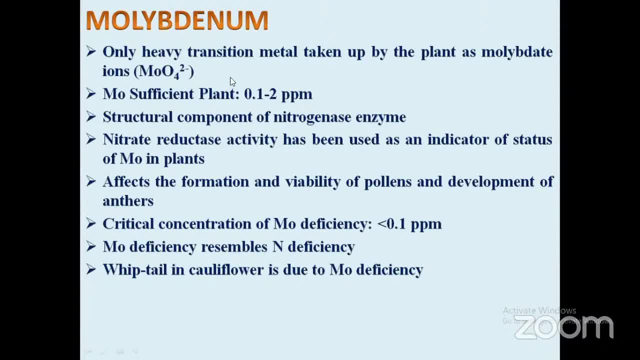 5 minus 4, also 6, 5, 4 and 2 different valencies of molybdenum. you now coming to this nitrogenase enzyme. so molybdenum is a structural component of nitrogenase enzyme and this enzyme has molybdenum iron protein. so if you have studied the biological nitrogen, 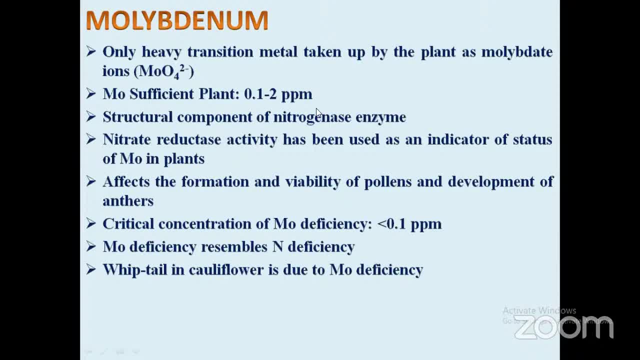 fixation. you must have heard that this nitrogenase enzyme is involved in biological nitrogen fixation and it is having two proteins actually. one is bigger protein, another is smaller one. so the bigger protein that is iron molybdenum protein. we are talking about that only so this molybdenum 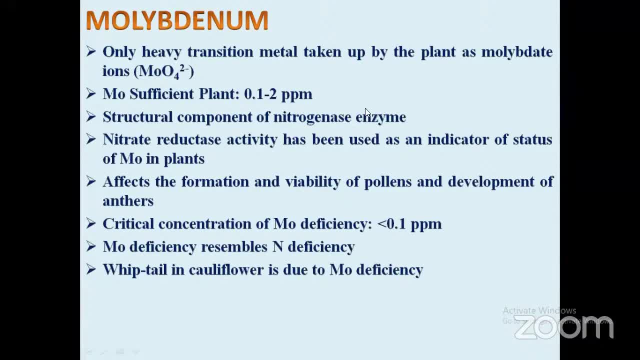 is a structural component of nitrogenase enzyme. this nitrogenase enzyme is having molybdenum, iron protein and catalyzed biological nitrogen fixation. that is why the molybdenum requirement of the nodulated legume is particularly high, because legumes require this nitrogenase enzyme to fix. 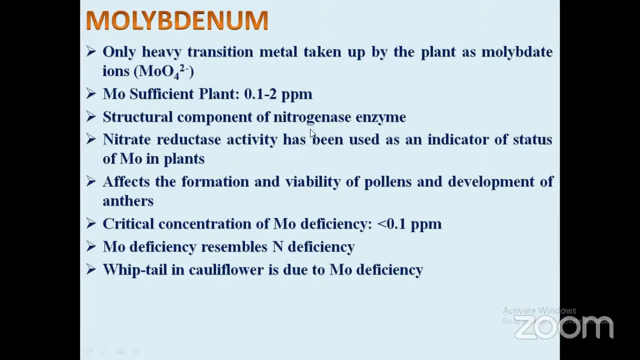 atmospheric nitrogen right. so molybdenum is required for leguminated, this nodulated, legumes. another is: nitrate reductant activity has been used as an indicator of status of molybdenum implant. you see, one is that molybdenum is a component of nitrogenase enzyme, another is that nitrate. 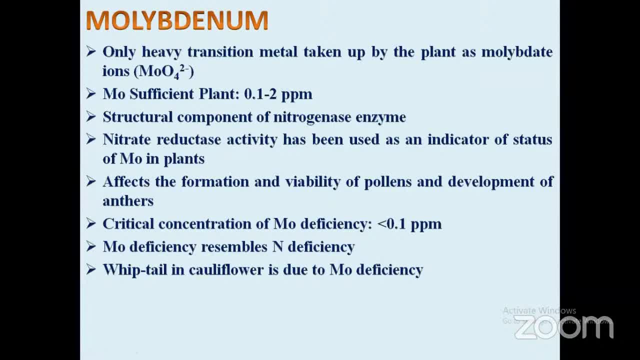 is reduced by nitrate reductase enzyme in the cytoplasm, by the transfer of electron from molybdenum to nitrate nitrate reductase. what does it do? it reduces nitrate to nitrite form right, and for reducing nitrate to nitrate form it requires electron. 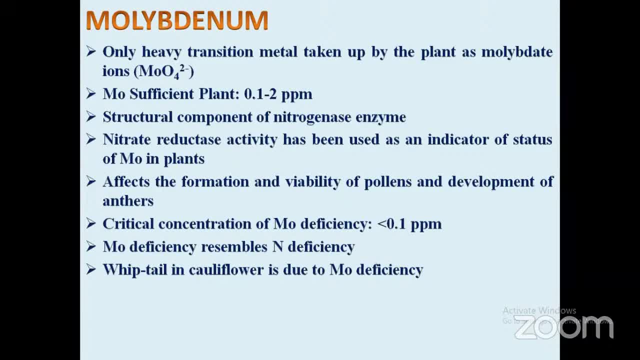 and this is a component of nitrogenase enzyme. so molybdenum is a component of nitrogenase enzyme. this electron is transported from molybdenum. so going to this really relationship between molybdenum supply, nitrate reductase activity and the plant growth, this nitrate reductase. 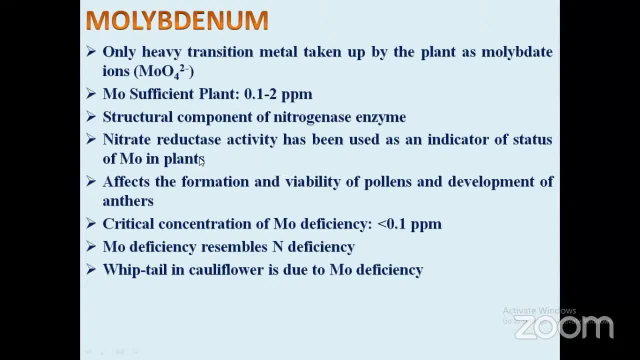 activity has been used as an indicator of status of molybdenum in the plant. what did i say? nitrate reductase is for reducing nitrate to nitrite, and to reduce nitrate to nitrate, electron scrub is required to transfer that electron from molybdenumисm, because molybdenumisel 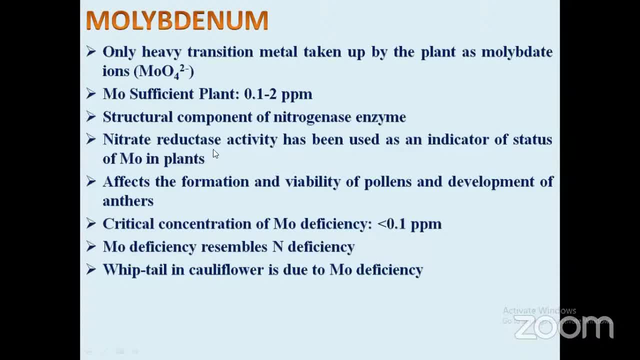 is the powerful substance of nitrate. it is considered a foreign further the origin of Because molybdenum is closely related to nitrate activity, reductase activity. that is why nitrate reductase activity has been used as an indicator of status of molybdenum in the plants. 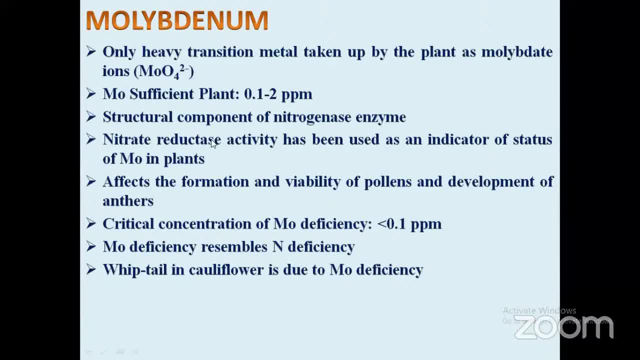 So you remember that molybdenum influences nitrogenous enzyme activity, nitrate reductase activity, And it affects the formation and viability of pollens and development of anthers. Critical concentration of molybdenum deficiency is less than 0.1 ppm. 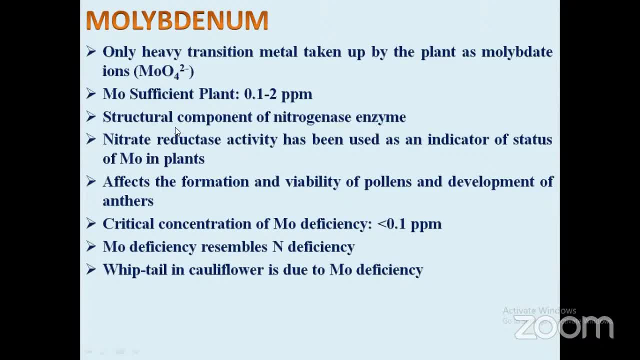 and since this molybdenum is affecting nitrogenous activity, nitrate reductase activity- so all in all it is affecting nitrogen cycle in the soil. So nitrogen availability is influenced by molybdenum. So if molybdenum deficiency is there, there will be deficiency of nitrogen also. 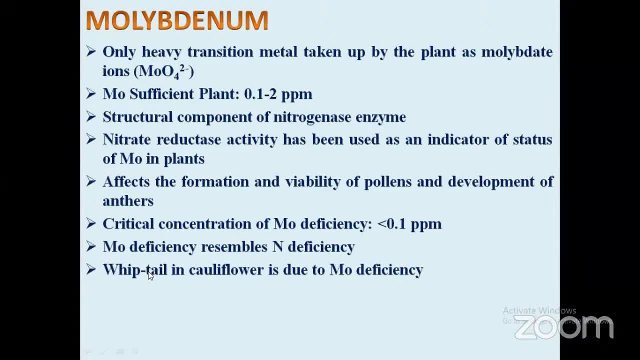 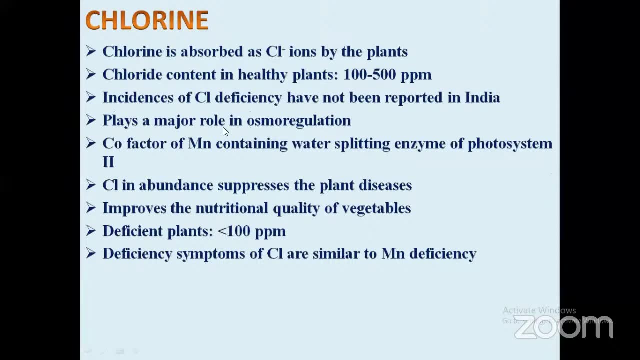 So they resemble each other. The most common symptom disorder of this molybdenum deficiency is whiptail in cauliflower, which is very frequently asked in exam: Whiptail of cauliflower due to molybdenum deficiency. Now, moving ahead to another element, that is, chlorine. 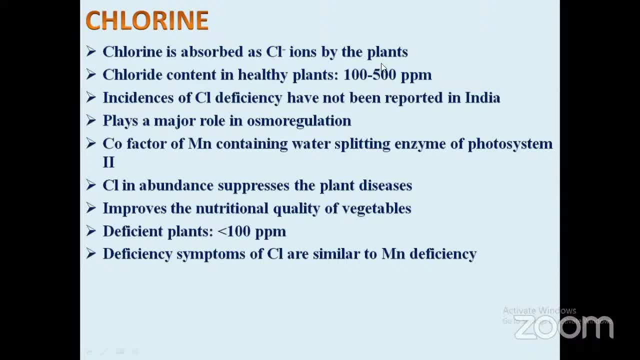 So chlorine is absorbed as chloride ions by the plant, and chloride content in healthy plant is 100 to 500 ppm. You see, the incidences of chloride deficiency have not been reported in India. Why so? Why chlorine deficiency is not reported? Because of its large 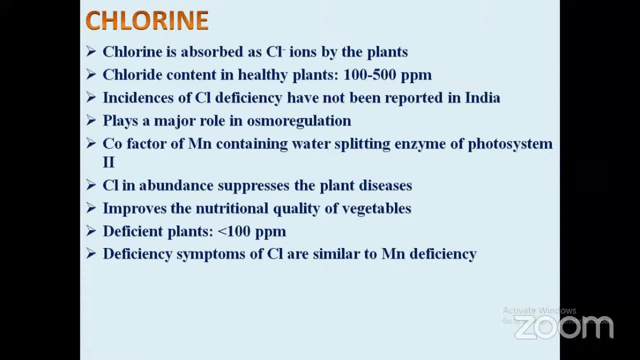 Because it is associated with manganese. Okay, one of the reason is this, only Any other? Okay, you see, you have heard of this murate of potash, no KCL. One reason is this. Another is, you see, because of its large abundance in the air. 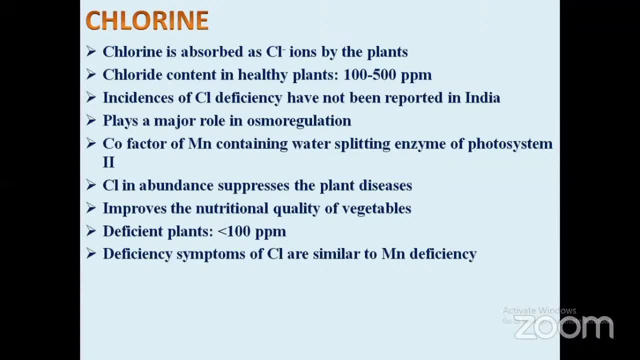 and its accretion through large number of fertilizers like MOP, ammonium chloride. So it is unintentionally being added to the soil. So it is. It is Sufficient for the plant, So deficiency of chloride is not reported in India. 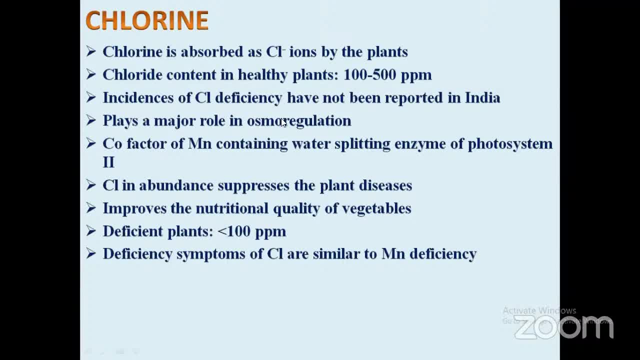 because of its larger abundance in air. Another is because of its presence in the fertilizers, like MOP and ammonium chloride, And it plays a major role in osmoregulation Co-factor. It is a co-factor of manganese containing water-splitting enzyme of photosystem 2.. 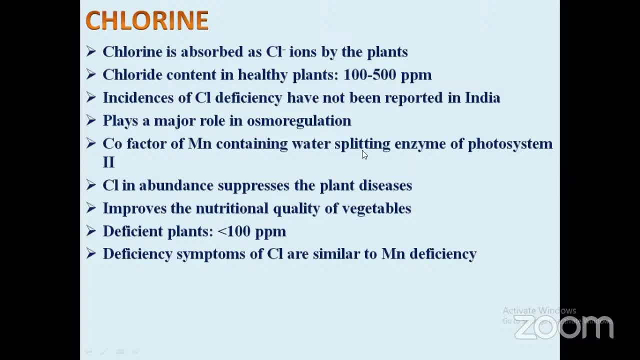 We have seen that manganese is associated with water-splitting enzyme, So this chlorine is co-factor, So it also helps in this water-splitting enzyme. Chloride in abundance suppresses the plant disease, So it also imparts disease resistance to the plant. 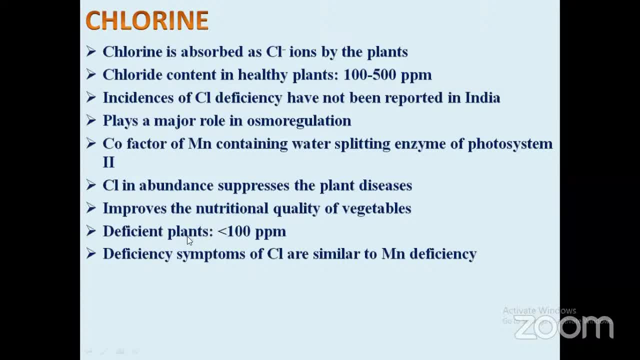 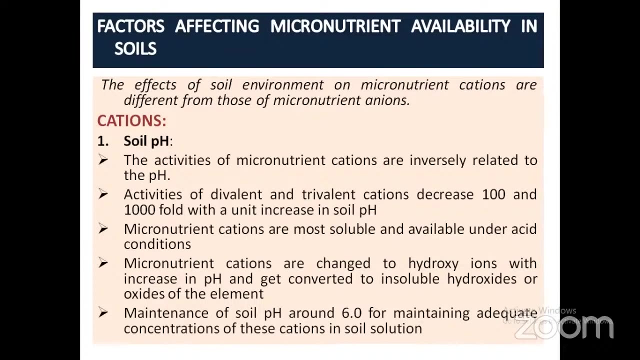 Improves the nutritional quality of the vegetables, And if it is less than 100 ppm there will be deficiency And deficiency symptoms of chlorine. they are similar to manganese deficiency. Now coming to factors affecting the availability of micronutrients in the soil, 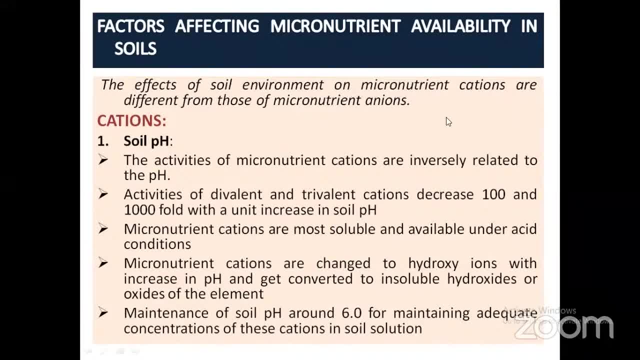 So you see the effect of soil environment on the micronutrient category Cations are different from those of the micronutrient anions. Soil environment effect means soil may concern nutrient presence. Hey present, Hey yeah, Ph. Hey yeah. 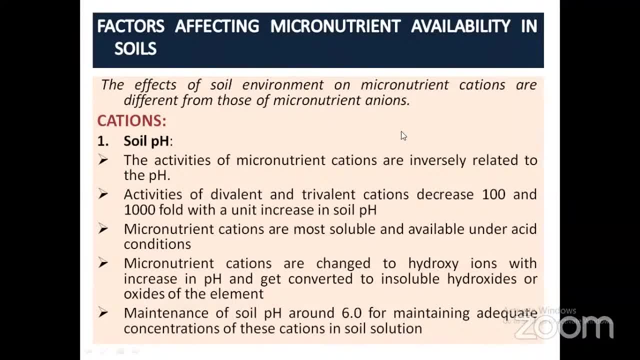 Redox condition. Hey, they'll have different impact on cations and anions, So we'll discuss them separately. Okay, So first we'll discuss what is the effect of soil environment on cations. So cations, micronutrient cations. 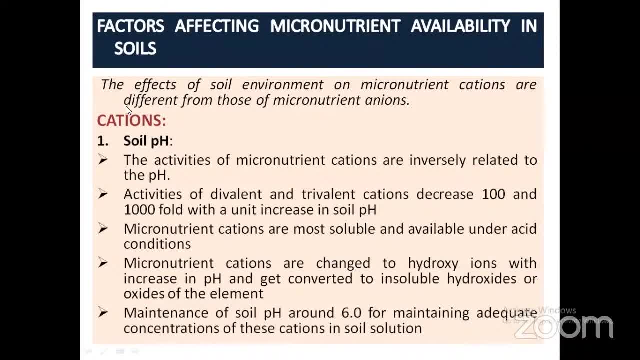 It will go, You both. Oh, I didn't, I don't, manganese. Oh well, go back. Honey, Can Five now? Okay, Now we'll see the effect of soil pH on cations. You see, soil pH predominantly regulates the solubility and availability of micronutrient cations in the soil. 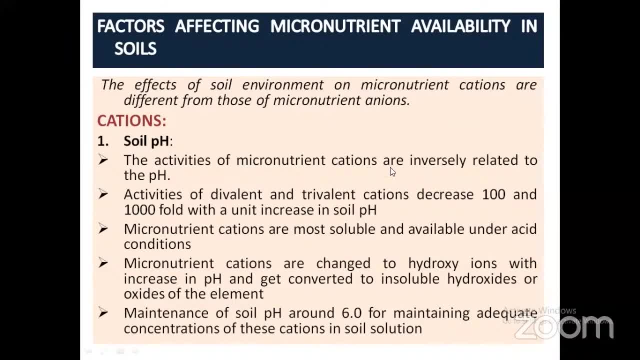 How the activities of micronutrient cations are inversely related to the pH. If the pH will be high, the activity of the micronutrient cation will be less. If pH Is less, the activity will be more, means in less pH range, the availability of the micronutrient cations is more wise. 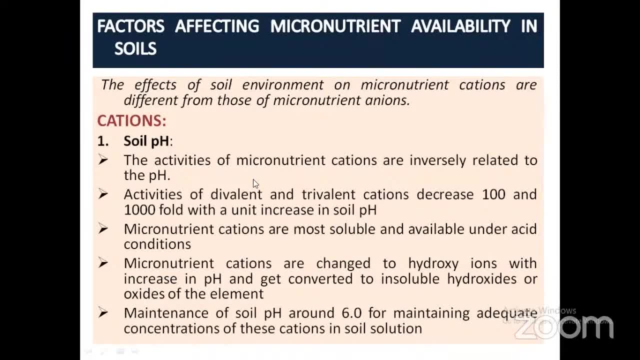 So we'll see that. But yes, this is the information for you, that activity of micronutrient cations is inversely related to pH. activity of divalent and trivalent cations decrease hundred and thousand fold with a unit increase in the soil. 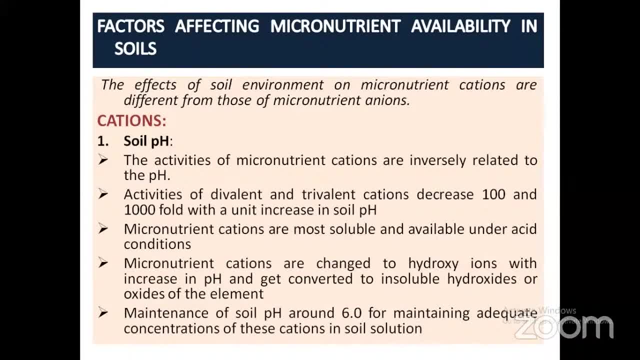 Ph A unit Ph. Keep burning this. It's a very What, Don't I? Yes, I'm listening. I keep asking: Burn this, My This, Yes, Yes, Basically a lot of activity, at least one unit in the. 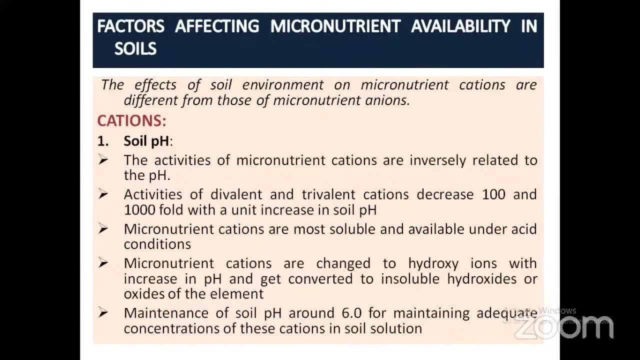 At the activity of the divalent cations. but the activity of the micronutrient cations are being reduced. Now, how much is being reduced? By increasing the pH of a unit, activity of the divalent cations is reduced by 100 times. 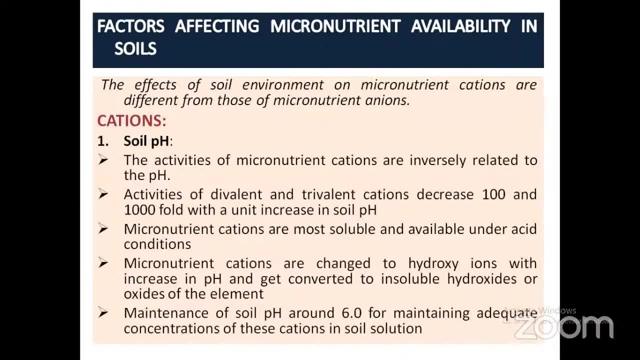 Because pH is log 10 to the log base. 10, right It is, Then it is going at the base, so it will go to 10 to the Power. So one unit increase in the soil pH will lead to decrease of that cation, and thousand fold for trivalent cations. 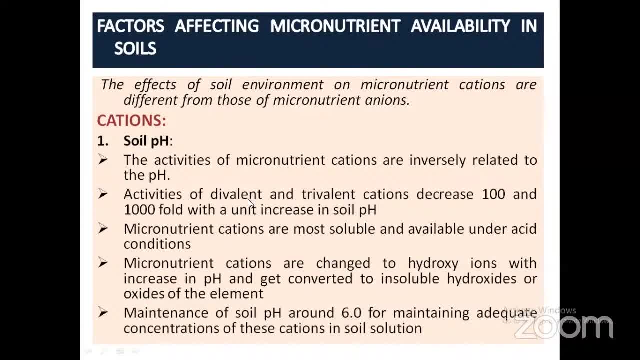 It will automatically decrease and it will decrease in the. It will immediately decrease in the soil pH. It will reduce, It will decrease cations. If it is monovalent, then there will be decrease in 10 fold. Okay, so you remember this. 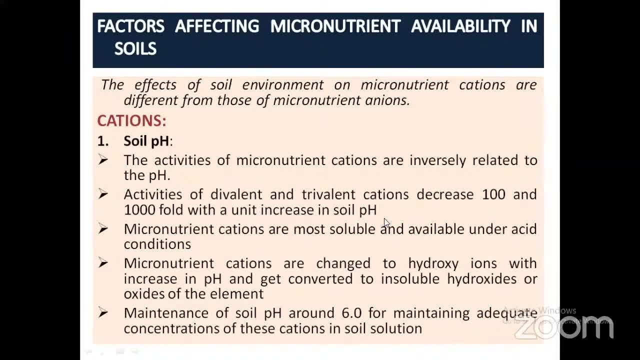 one Directly with each unit increase in the soil pH. what is the effect on activity of Fe2+? so it will decrease 100 fold because it is divalent. If it is asked about trivalent ferric form, Fe3+, then it will decrease around 1000 fold. Microneutrin cations are most soluble. 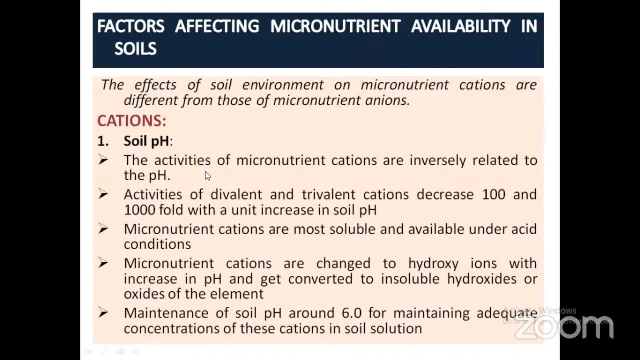 and available under acid conditions. One thing we have seen ki aisa hota hai, lekin kyun hora hai. So micronutrin cations: they are more soluble and available under acid conditions because micronutrin cations are changed to hydroxy ions with increase in the pH. So 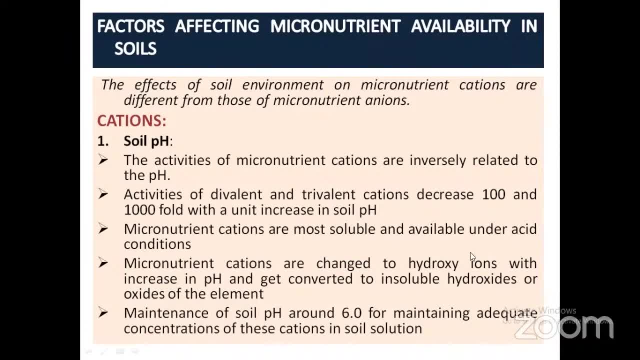 with increase in the pH, these micronutrin cations, they are changed to hydroxy ions and get converted to insoluble hydroxides or oxides of the element. So pH badhne ki wajah se wahan pe hydroxyl ions zyada honge. 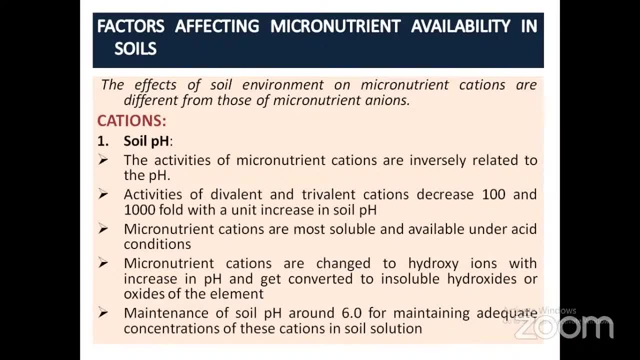 nah. higher pH. pe to micronutrin cations. they are converted to insoluble hydroxides and oxides. That is why their availability is less at higher pH And all the hydroxides of this micronutrin cations. they are sparingly soluble, But the degree of their solubility 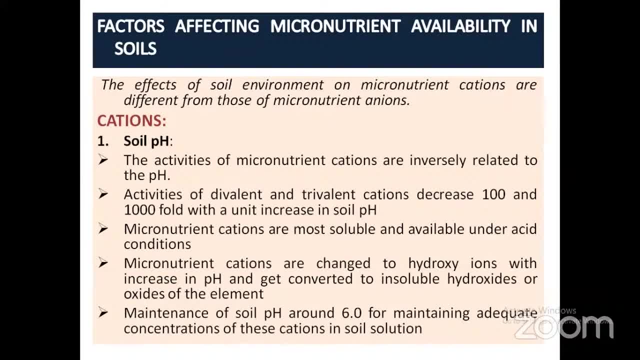 varies. Aisa nahi hai, ki saare micronutrin cations ke hydroxy ions, jo bhi banenge hydroxides or oxides ko kisi ek particular pH mein jaakar li dissolve hongi Their solubility. 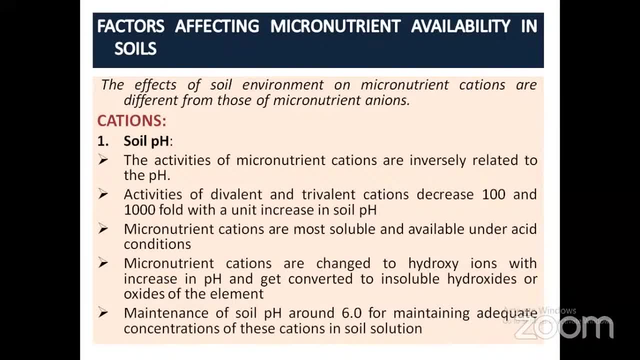 varies. But yes itna sure hai ki inki solubility varies, But yes itna sure hai ki inki solubility kam hoti hai, Jiski wajah se pH badhne, se micronutrin cations ki availability kam hoga. 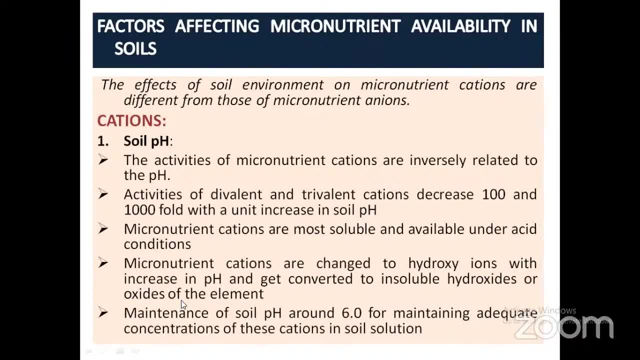 You see, the formation of insoluble hydroxides starts as soon as the pH of the soil solution is raised to 6 and above. Abhi hydroxides, kitne pH ke baad banna shuru hongi jaise hi soil ka pH 6 ya 6 se upar jaega ye hydroxides or oxides, banne lagenge jiski wajah se micronutrin. 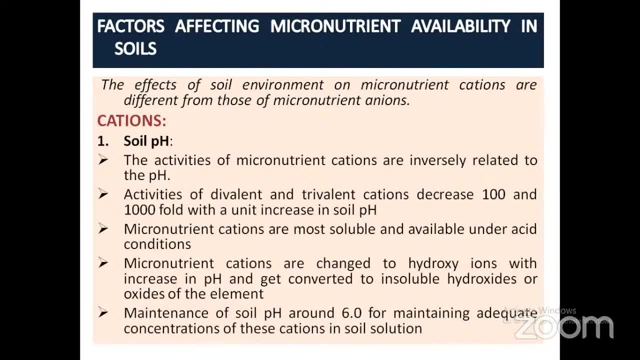 cations ki availability kam ho jayegi. So this is why the solubility is less. So the formation of insoluble hydroxides starts as soon as the pH of the soil solution is raised to 6 and above. So maintenance of soil pH around 6 for maintaining adequate concentration. 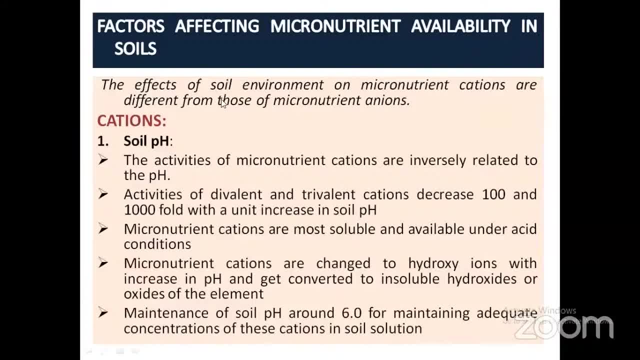 of these cations in the soil, solution is necessary. So agar hume micronutrin cations ki availability plant ko pohchani hai. so the pH has to be less than 6.. Because at pH more than 6, there 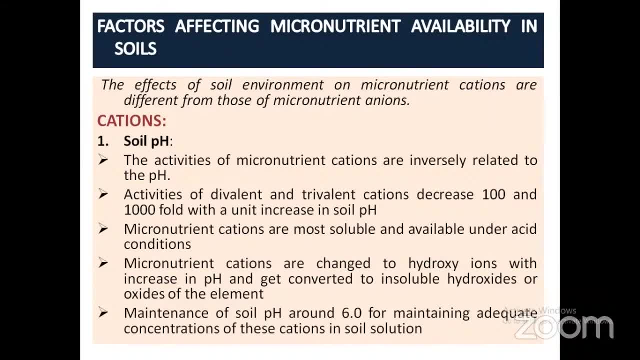 will be formation of insoluble hydroxides and oxides. This is one thing. I'll ask you one question. So the pH of the soil solution is raised to 6 and above. So the pH of the soil solution is increased, So composition is reduced. Population of the soil solution. 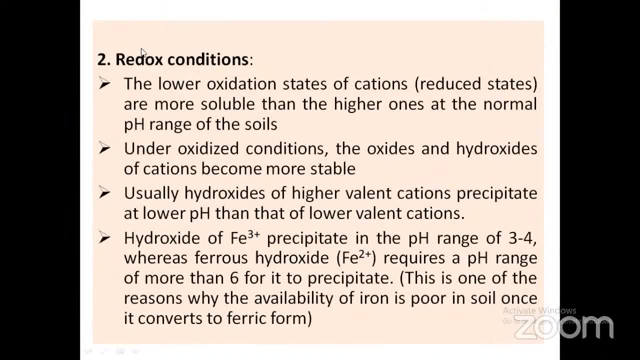 is increased, Filter concentration is reduced, So alkaline off the ground, and now it is. How do I have this list for Dukeifiques usoShall? I give you a quiz about questions after two slides. Okay, now another is: we will see the effect of redox conditions on the availability. 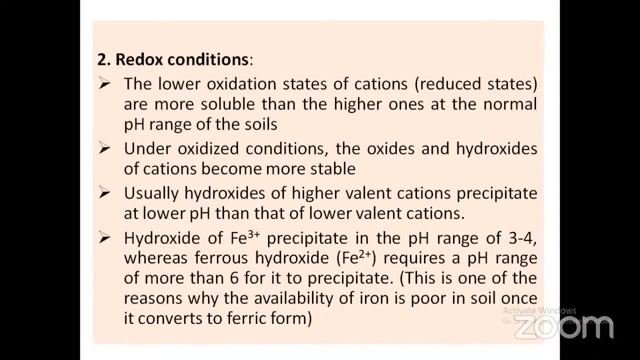 of these micronutrin cations. So the lower oxidation states of cations means the reduced state. they are more soluble than the higher ones at the normal pH range of the soil. If you consider iron, we have Fe2+ and we have Fe3+, ferrous and ferric form. ferrous is 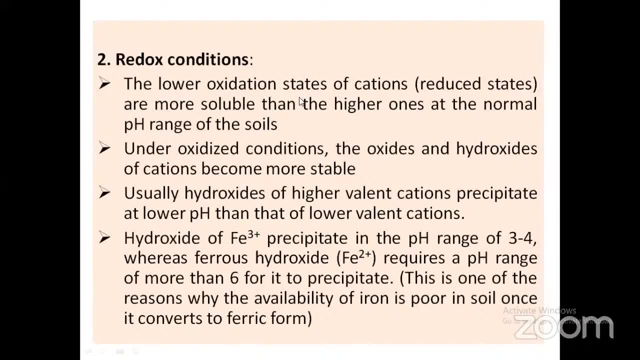 reduced form. ferric is oxidized. form right. So the lower oxidation, first of all this Dialysis- is reduced from. ferric is oxidized. So the lower oxidation state of the cation means Fe2+. They are more soluble than the higher one, that means Fe3+. 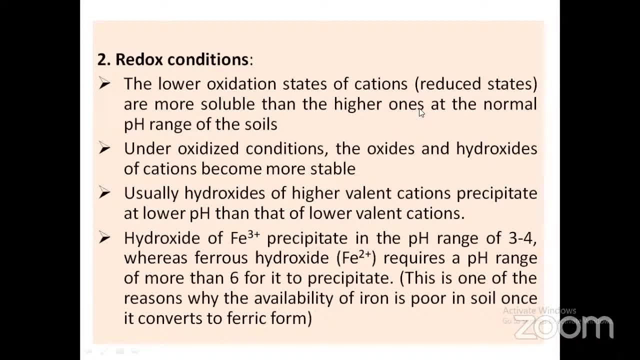 So Fe2+ is more soluble than Fe3+, And under oxidized conditions. why is this happening? Under oxidized conditions, the oxides and hydroxides of the cations become more stable, See, reduced condition is more soluble than the oxidized form. 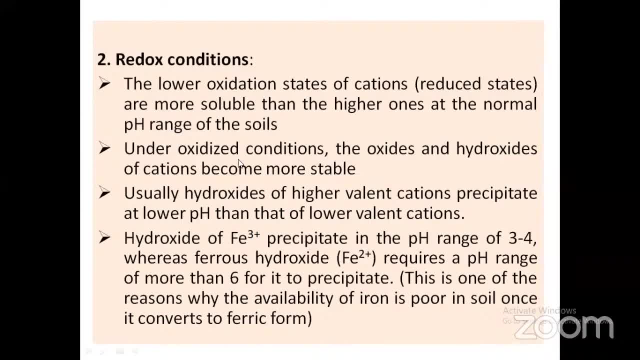 Why? Because under oxidized condition- oxides and hydroxides of the cations- they are formed and they are more stable. Okay, So they are less soluble And usually hydroxides of the higher valent cations precipitate at lower pH than that of the lower valent cations. 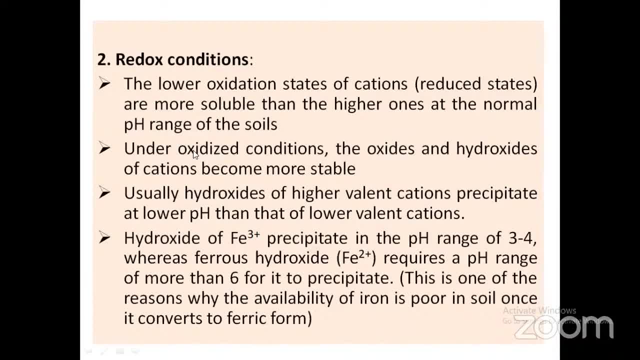 So the first thing that happened was that cations will be more soluble in reduced condition. Why? Because as soon as oxidized condition comes, these cations will make their oxides and hydroxides, And hydroxides and oxides will be more soluble. 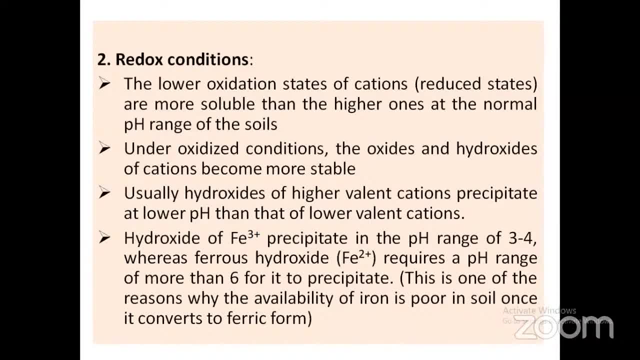 So they are stable, So they will not be soluble. Secondly, usually hydroxides of higher valent cations. Higher valent cations: here you have to take only one cation. You have to consider its higher valency and lower valency. 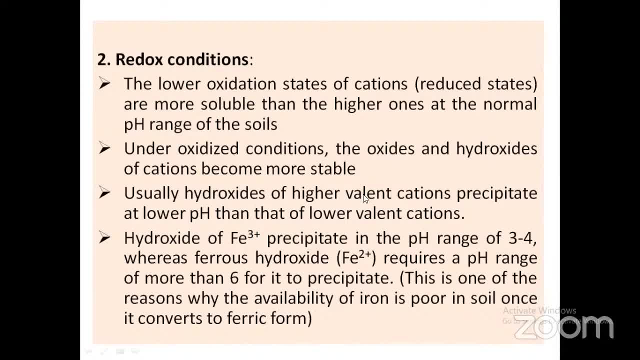 So hydroxides of higher valent cations means hydroxides of Fe3+. it precipitates at lower pH. Fe3+ hydroxide precipitates at lower pH, Whereas if Fe2+ hydroxide is present, it precipitates at lower pH. 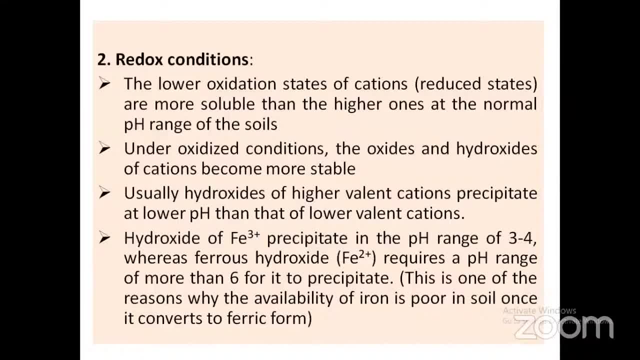 So it precipitates at lower pH. nahi hoga. So it is more soluble. Making sense to all of you? Yes, Hello, Ma'am, ek bah repeat kar do, please. Okay, Pehli baat: humne ye batai ki jo lower oxidation state. 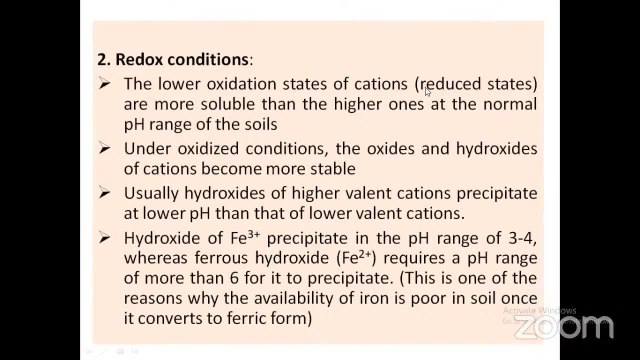 hai ket ion ki. Agar hum iron ki baat karen to, it is Fe2+, So Fe2+ is more soluble than Fe3+. This is one thing. Why is it so Is ka explanation. hai aage Kyun ki oxidized. 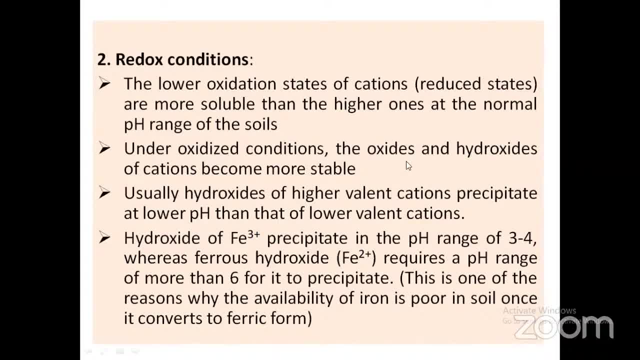 condition me oxides or hydroxides banenge na Reduced condition me to Fe2+ e hai, Lekin agar oxidized condition me hai to wahan pe oxides or hydroxides banenge Ferric oxide or ferric hydroxides Which are more stable To uski availability kam ho jayegi Isle. 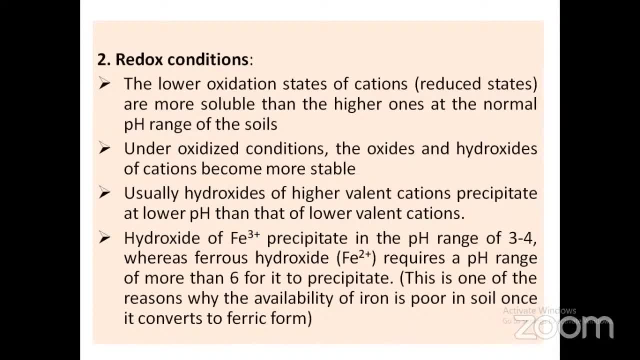 reduced form jo hai, wo zyada available hai plant ko As compared to the oxidized form. Doosri baat: jo bhi amara Fe2+ hai aur Fe3+ hai To Fe3+ ka, jo hydroxide hoga aur ek Fe2+. 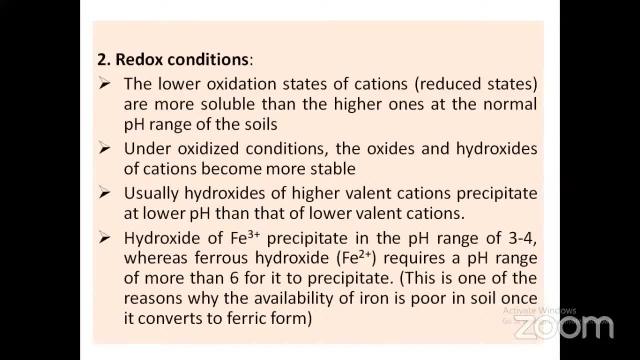 ka hydroxide hoga to Fe3+ ka hydroxide lower pH pe precipitate ho jayega. Ise liye acetic range me Fe3+ ki availability plant ko kam hoti hai. Fe2+ zyada available hai, Kyunki. 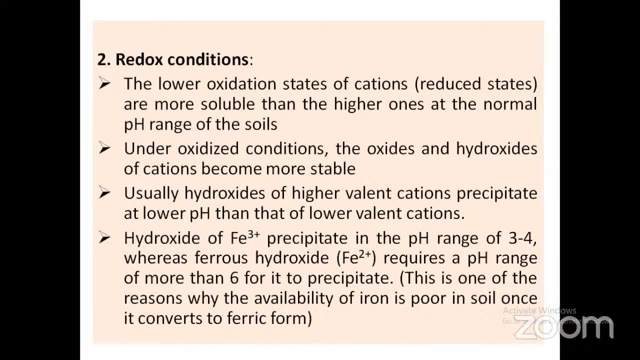 wo precipitate nahi kar raha hai. Jabki Fe3+ jo hai wo precipitate kar raha hai. Making sense, Yes, Yes, ma'am, yes, ma'am Okay. another is, you see, the hydroxide of ferric. 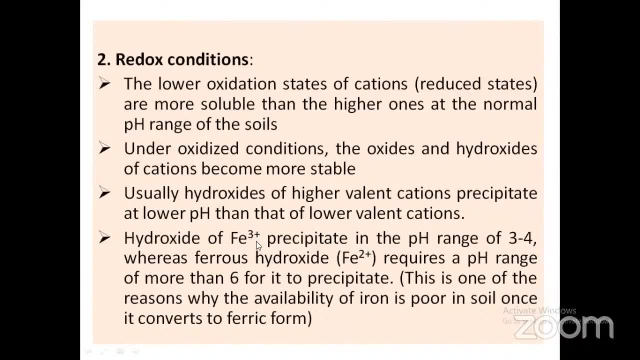 precipitate. as I said, ki jo bhi higher valent hai, uska hydroxide lower pH pe precipitate ho jayega, Lekin kitna lower To value. me bhi dekhte hai. So hydroxide of Fe3+ precipitate. 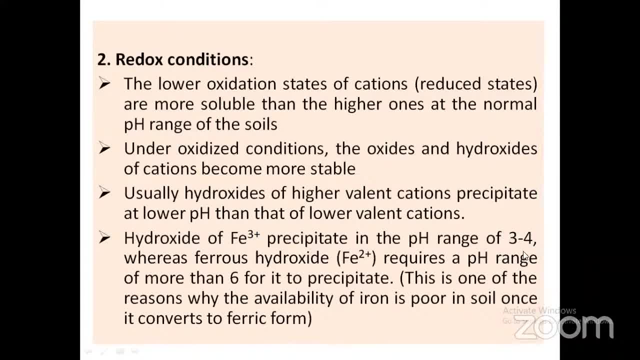 in the pH range of 3 to 4.. So 3 to 4 pH me ferric hydroxide precipitate ho jayega, Whereas this ferrous hydroxide it requires a pH range of more than 6 for it. 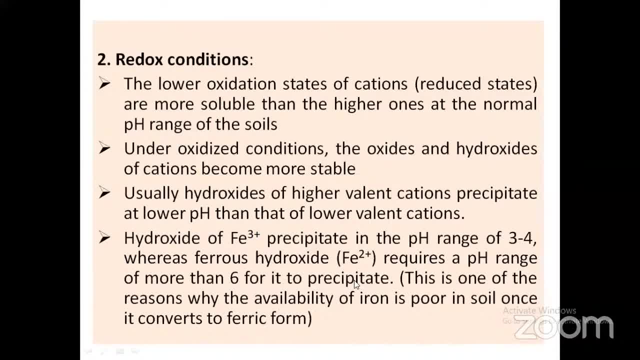 To precipitate. Hume. ye pata hai ki hamare micronutrient acetic range me available hain, Aur acetic range me ferrous form precipitate nahi hota hai. Ise liye plant used to take this ferrous form rather than this ferric form, Because it used to precipitate at pH. 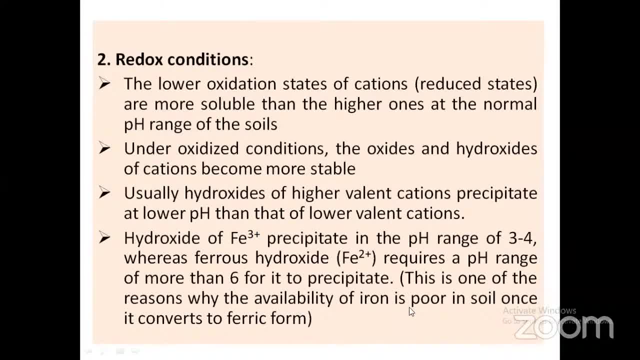 3 to 4.. So this is one of the reason why the availability of iron is poor in soil once it is converted to ferric form. So availability of iron, if you see, this ferrous form is available to the plant rather than this ferric form, Because this ferric form is available. 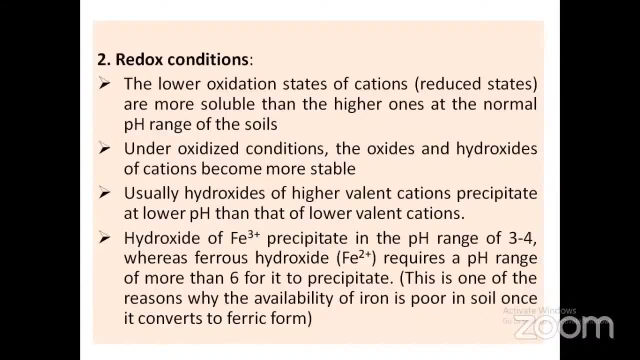 at pH 3 to 4.. Whereas this ferrous form require pH more than 6 to precipitate. So it will not precipitate in the acetic range. Making sense to all of you? Yes, ma'am, So do bate humne padhi Pehla pH ka effect. So acetic pH me. micronutrient cations available. 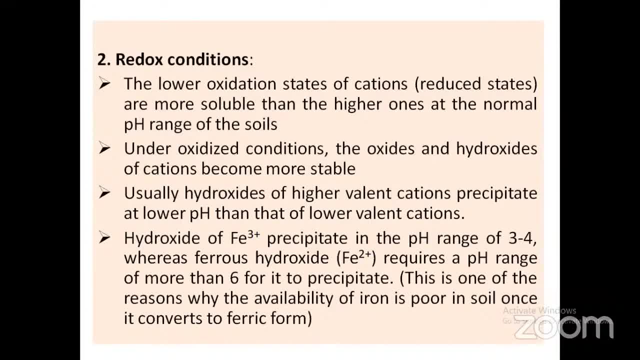 jyada hongi higher pH pe nahi hongi Redox ki baat kari to reduced form plant ko jyada available hoga as compared to the oxidized form. These are the two points that we have discussed. 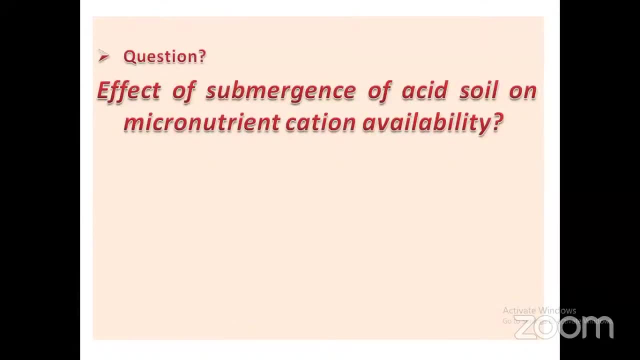 Now comes the question for you. You think and you tell. Question is: what is the effect of submergence of acid soil on the micronutrient cations? availability Kinkin baato pe dhyana hai Pehli baat submergence yaani waterlogged condition hai Isko relate karo redox se. 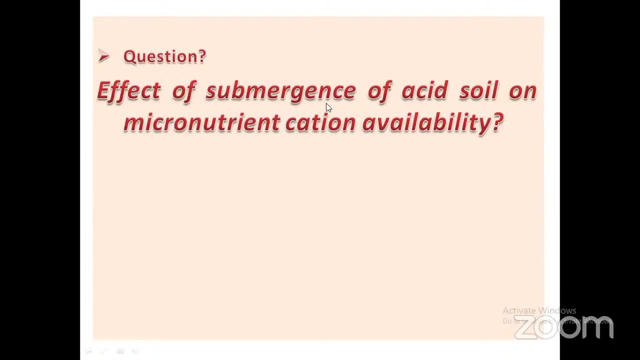 Doosri baat: acetic soil hai, Ye bhi dhyana rakhna hai. Aur teesri baat: hum sirf cations ki baat karte hain. Thik hai Toh thoda socho, aur mujhe batao ki chalo ek, ek tarke isko break. 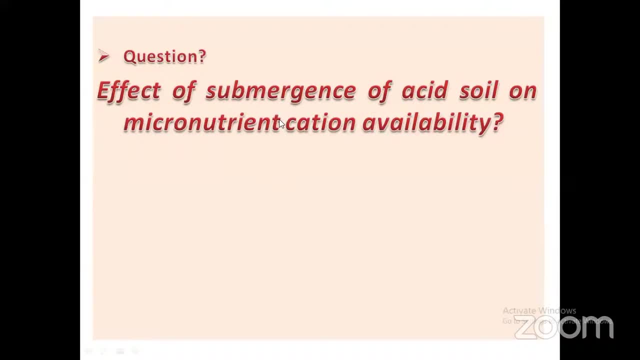 mari ka hai. What is the effect of submergence on cations availability? Soil hamari acidic hai. Tu mujhe yeh batao, ki acidic soil mein submergence ka effect kya hoga? What is the effect of submergence on pH of acidic soil, Whether it will increase or decrease? 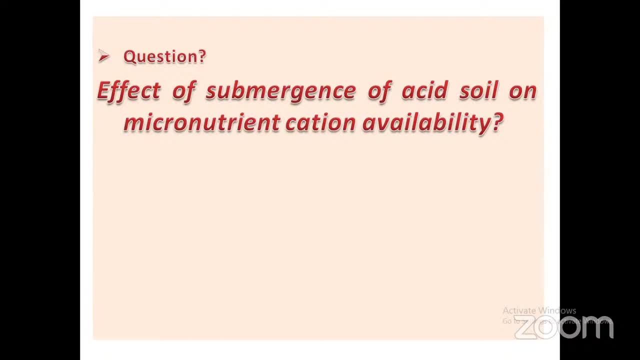 Pambu neutral ek aproji seg raha hai. Increase hoga, ma'am. Increase hoga Toh, agar acidic soil hai, submergence ki wajah se pH increase hoga. Agar pH increase horah mai, toh micronutrient availability kam hoga. 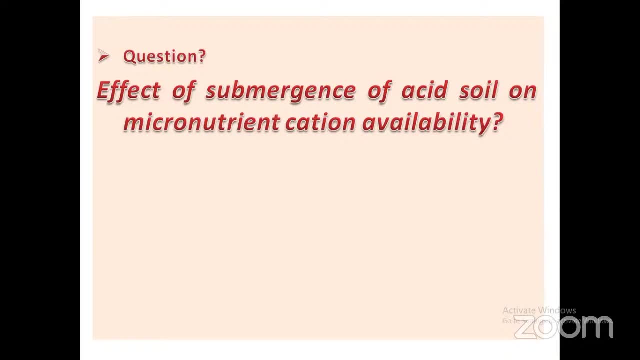 Krishan, availability will be less or more, It will be less, It will be less. Everyone understood this right. The first thing is that if submergence is happening of acidic soil, then micronutrient availability will be less because pH is increasing. 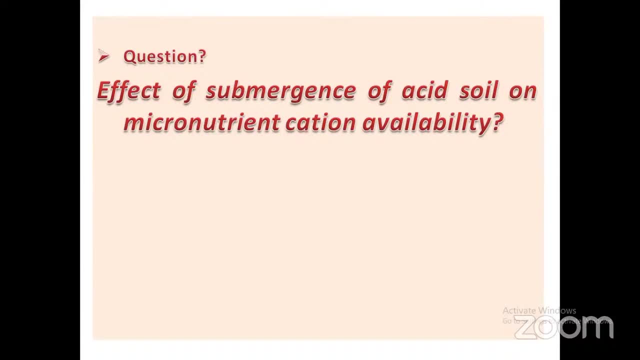 Is everyone understanding this? Yes, ma'am. Next thing: I told you that the reduced form is more available to the plant as compared to the oxidized form. So, due to submergence, reduced form is being created or oxidized. 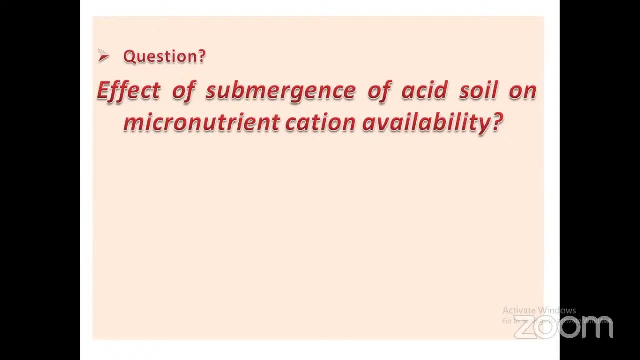 Reduced form. Reduced form, So the availability of the plant should increase. Oxidized. Can you understand what I am trying to say, Ma'am? reduced form, Fe2 plus or Fe3 plus- Yes, talk about any cation. 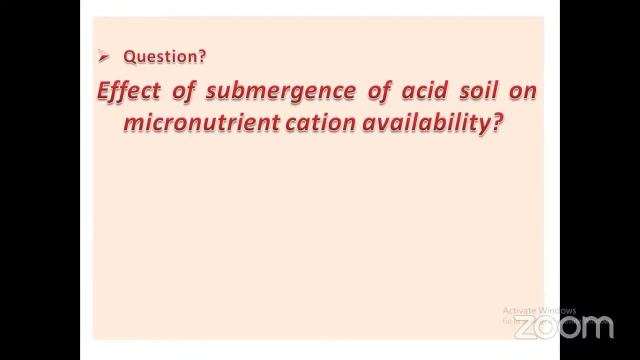 First thing I told you, If we take an example, then Fe2 plus or Fe3 plus, which one will it be? Reduced form is Fe2 plus. Fe2 plus If it is more than Fe2 plus. Yes, you see. 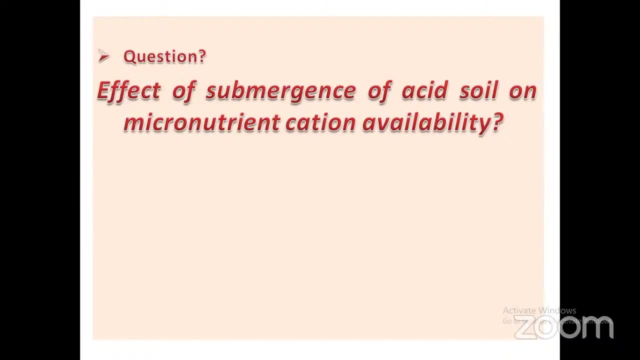 Okay, I will say it again So you will understand my point more carefully. Maybe now you are not understanding my question. The question is that if there is acidic soil and submergence is happening, then will the availability of micronutrient cations increase or decrease? 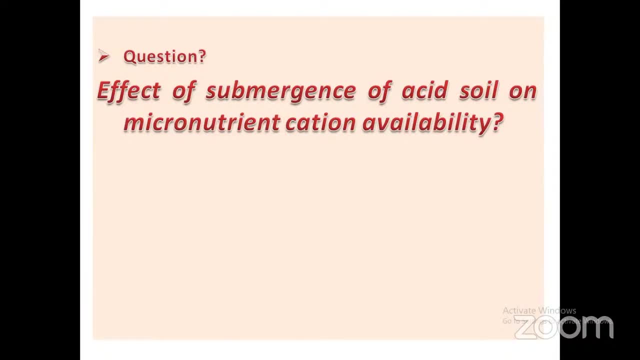 This is the question. Okay Now, due to submergence, the pH of acidic soil will go towards neutral. That means the pH has increased due to acidic rain. Because the pH has increased, the availability of micronutrient cations will increase. 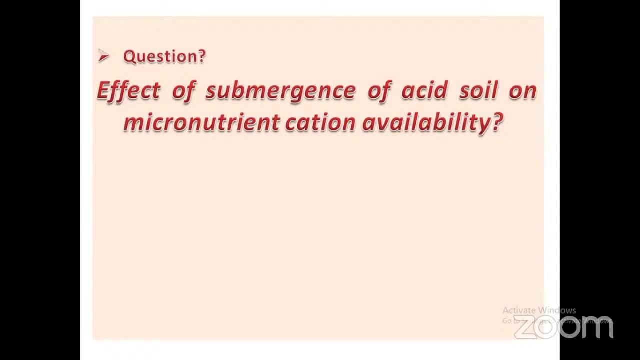 So the availability should decrease. First thing. Second thing: I told you that the reduced form is more available as compared to the oxidized form. So if we are doing submergence, that means we are creating reduced condition. So if reduced condition is being created, then it means micronutrient will also be in reduced form. 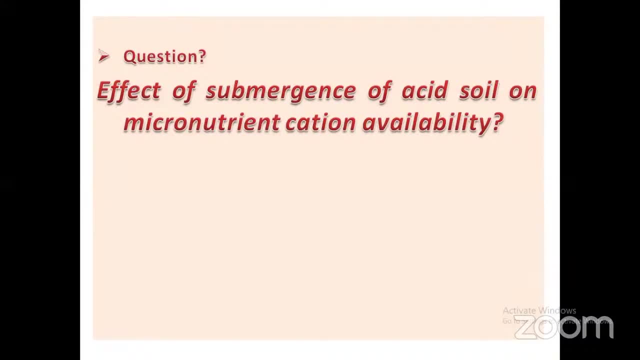 So its availability should increase. In the first statement we are saying that, due to submergence, micronutrient cations are decreasing. Second thing, we are saying that the availability of micronutrient cations is increasing. Third thing, we are saying that, due to submergence, micronutrient cations should increase. 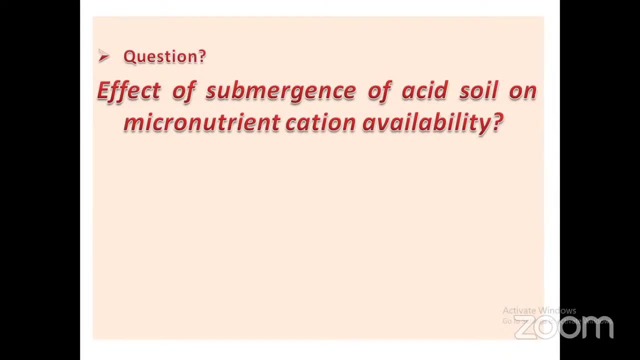 Both are contradictory things. Are you able to understand what I am saying? Yes, ma'am, Because of reduced condition, it should increase. Both are contradictory things. But then what will be the net effect Due to submergence? will micronutrient cations increase or decrease? 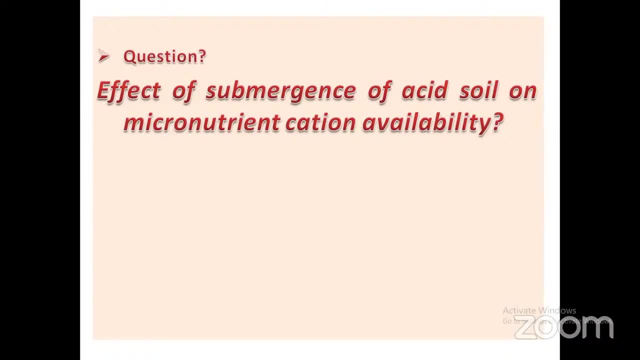 How do we tell this? So now I am speaking. I will speak slowly. Listen to me carefully, Okay, You see, in general, if acid soil is brought under prolonged submergence. You see, in general, if acid soil is brought under prolonged submergence. 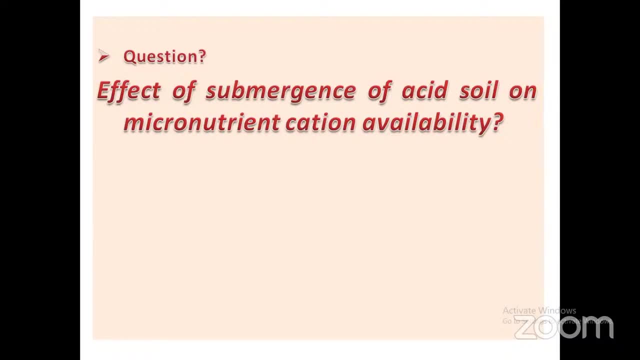 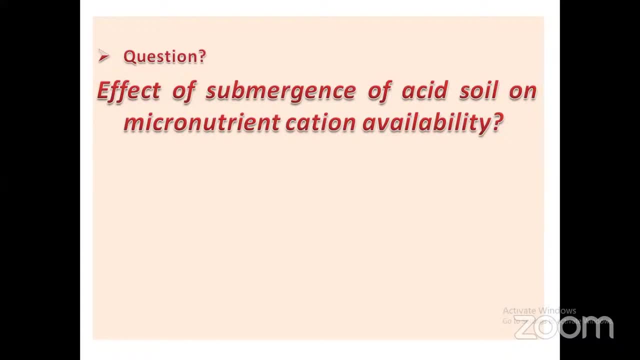 The pH gradually approaches neutrality, leading to the reduction in the solubility of the micronutrient cations. On the other hand, dissolution of iron manganese oxide enhances the solubility and availability of micronutrient cations, with the reduction of redox potential. 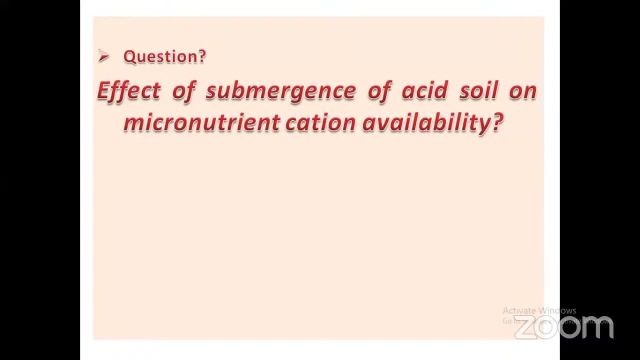 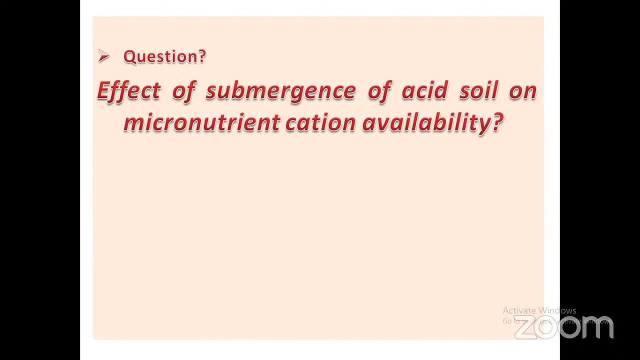 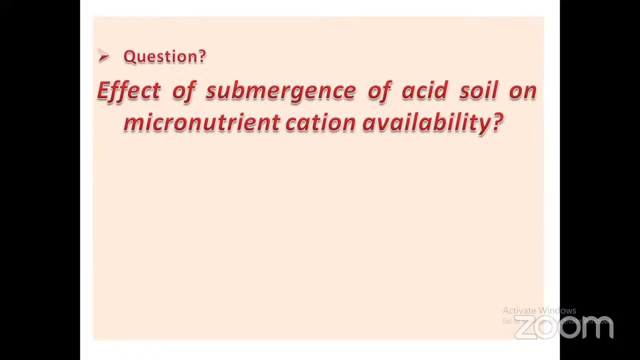 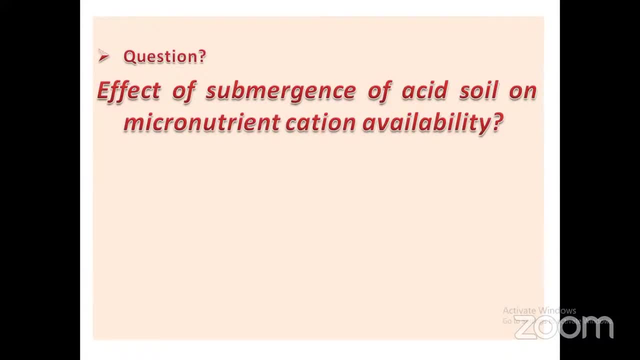 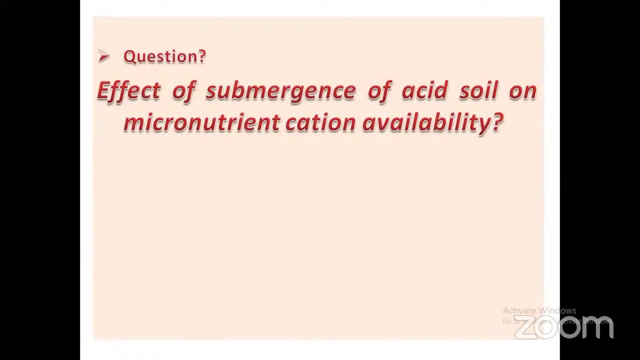 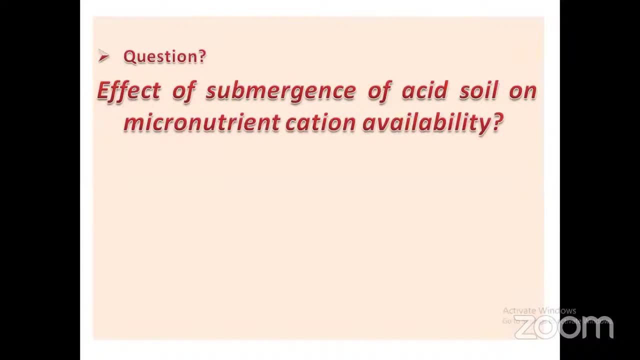 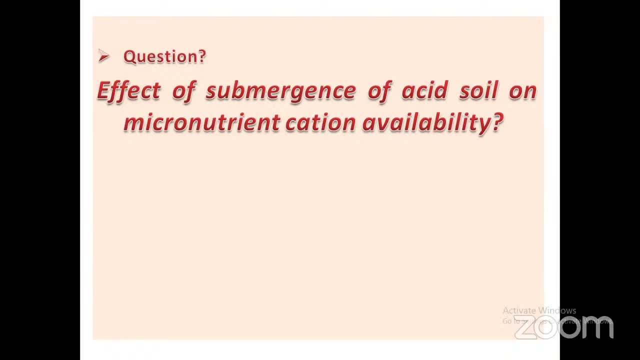 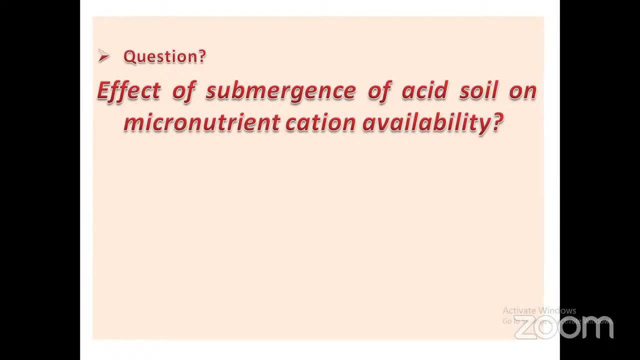 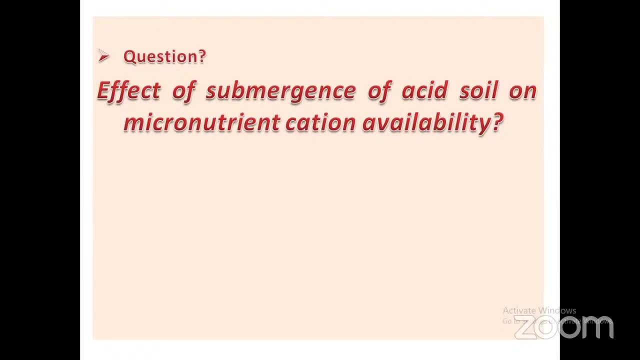 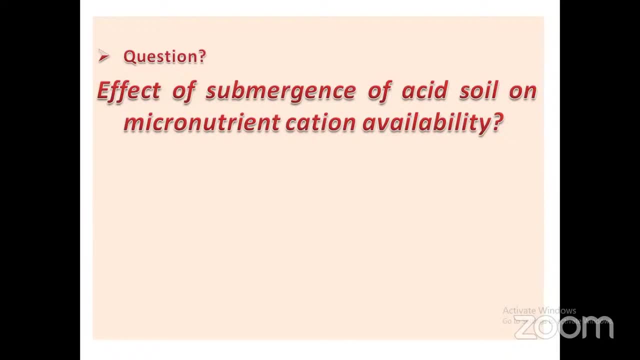 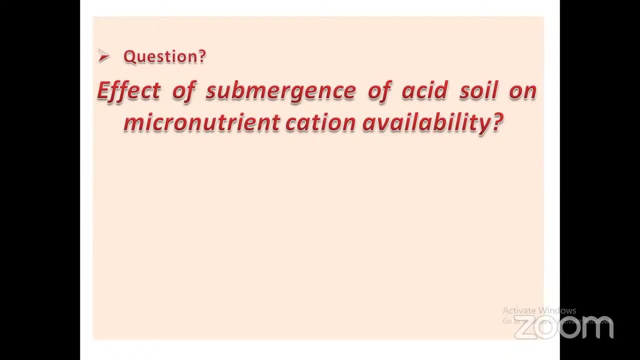 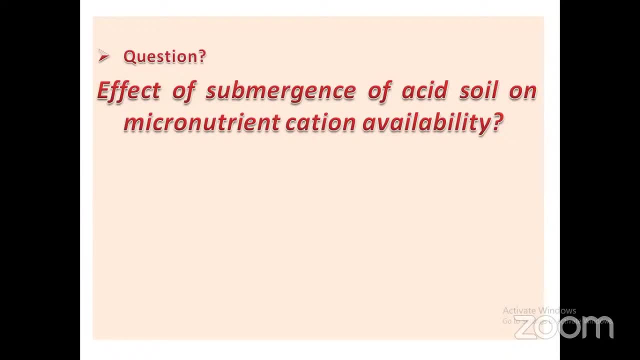 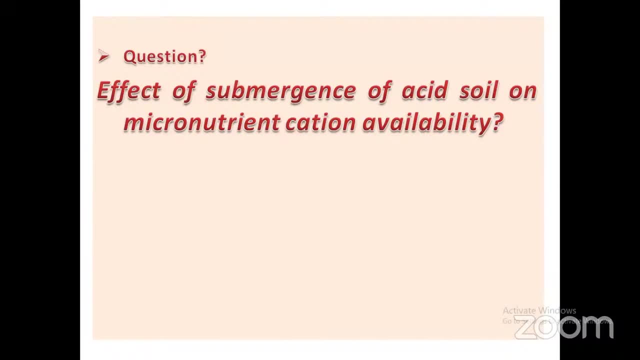 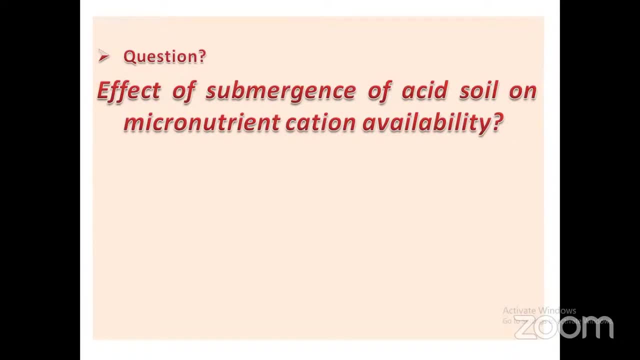 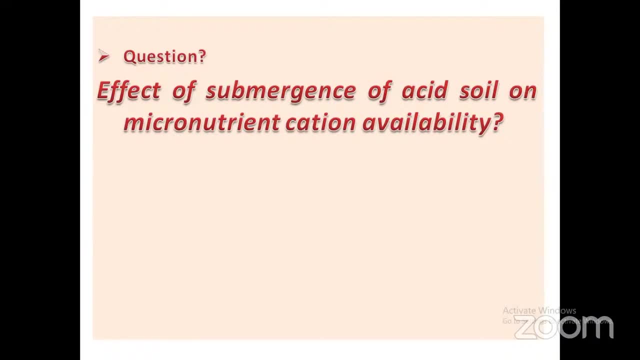 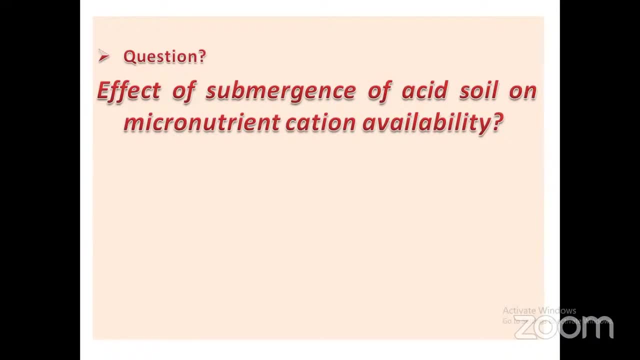 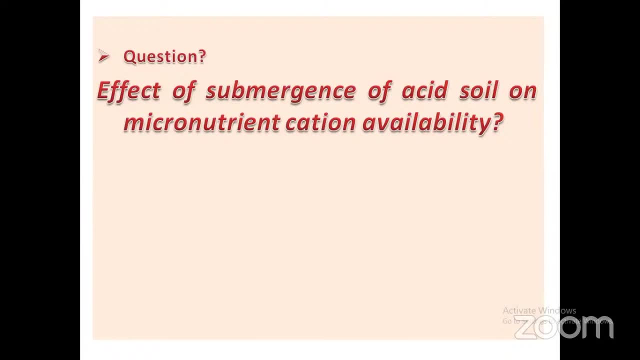 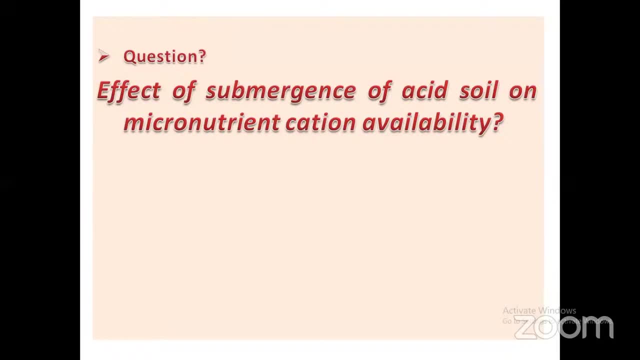 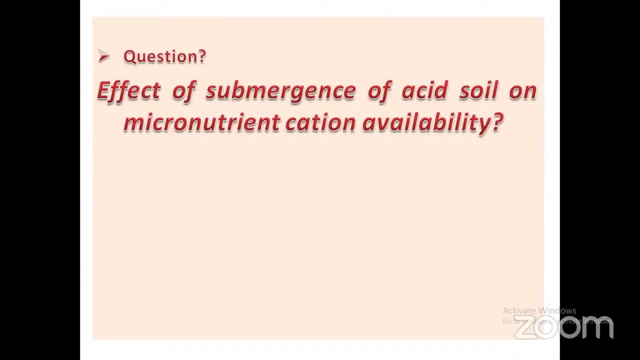 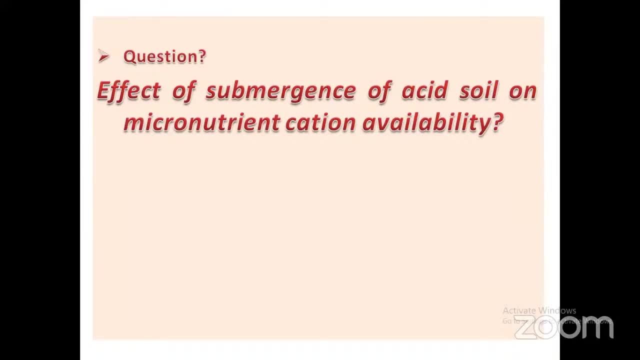 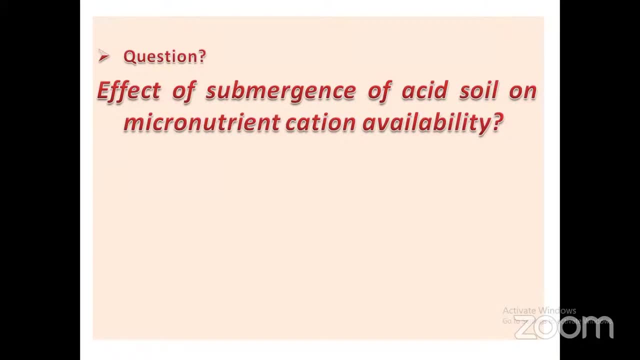 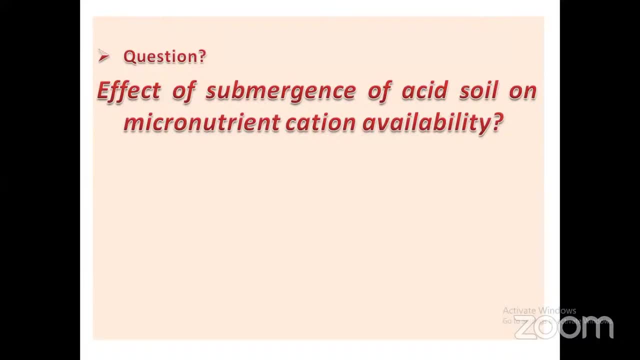 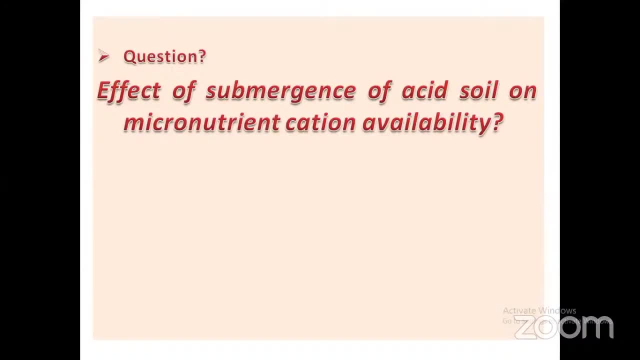 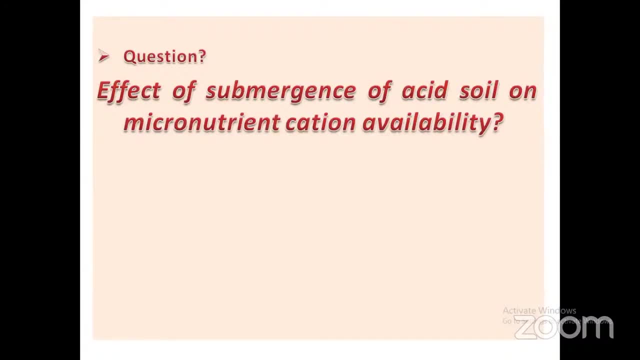 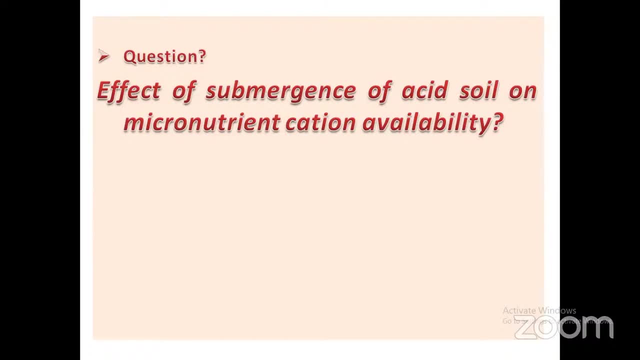 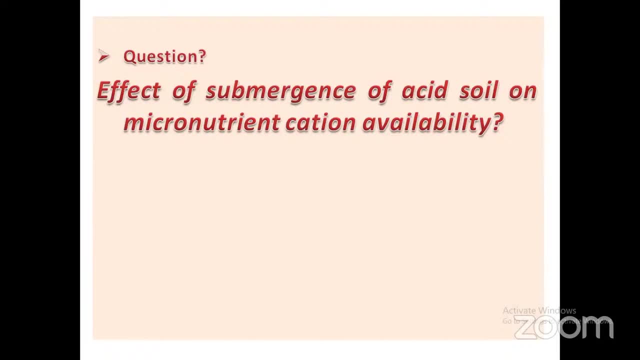 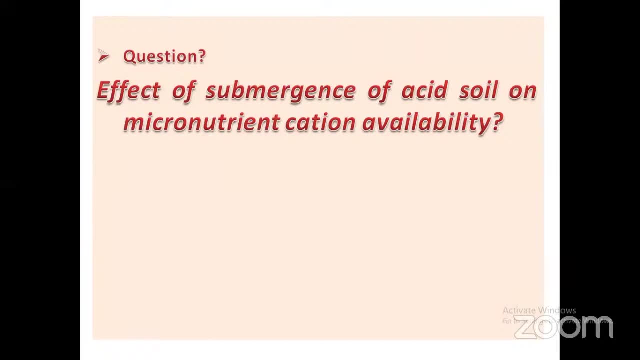 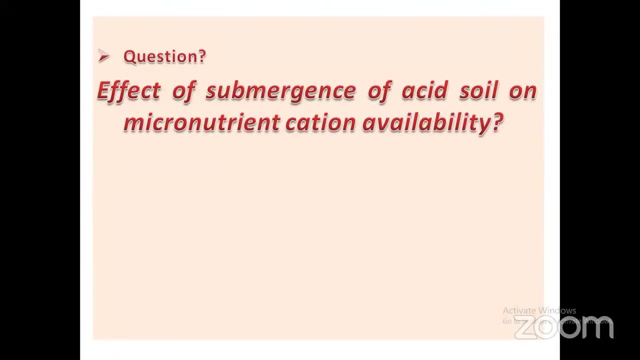 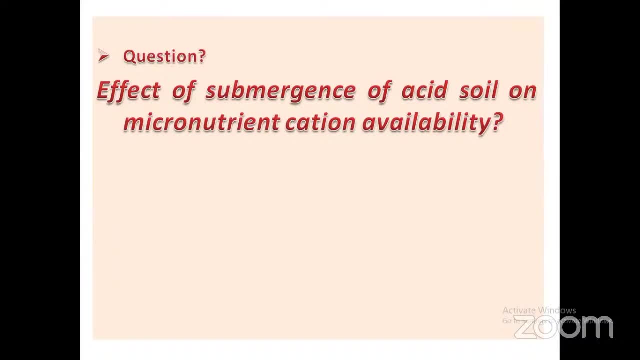 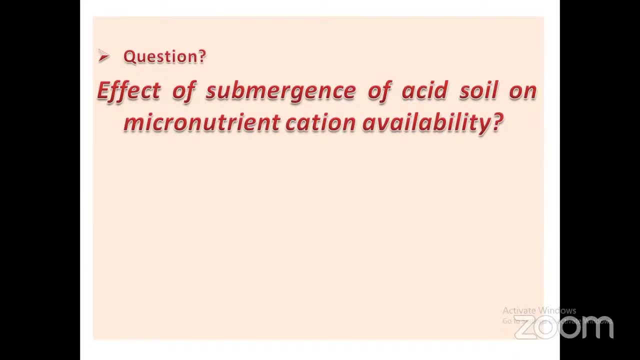 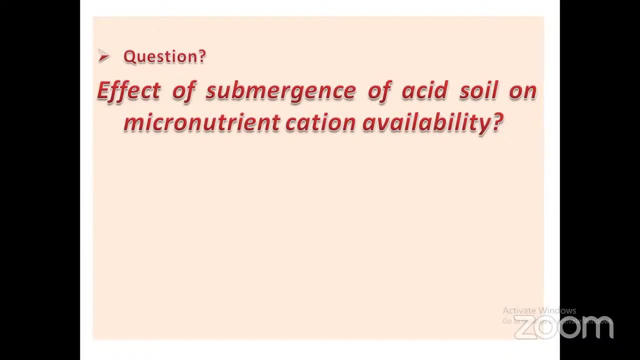 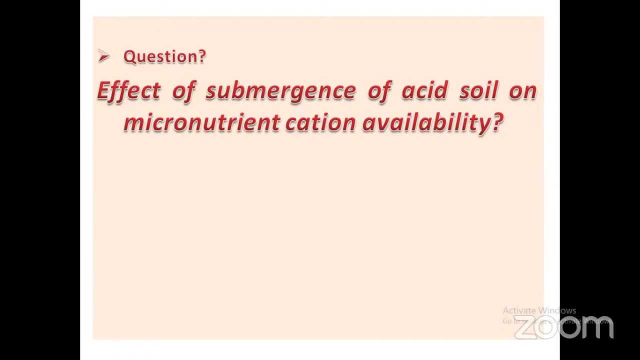 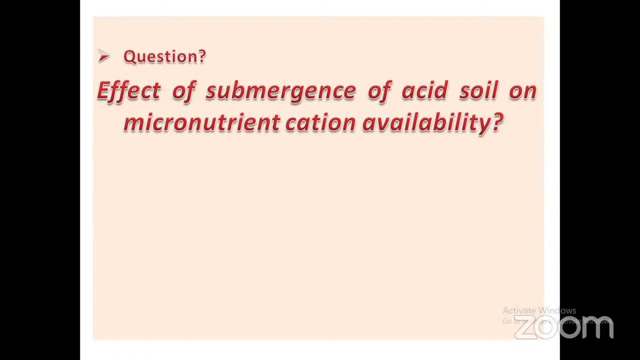 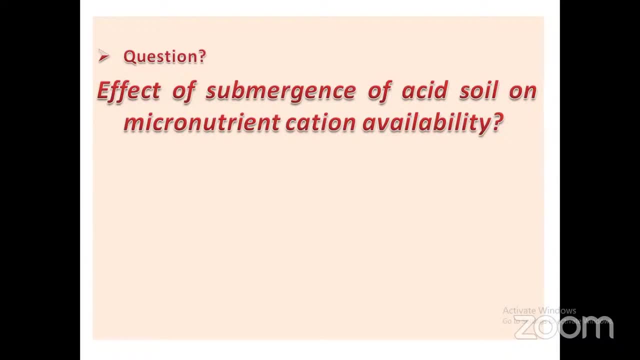 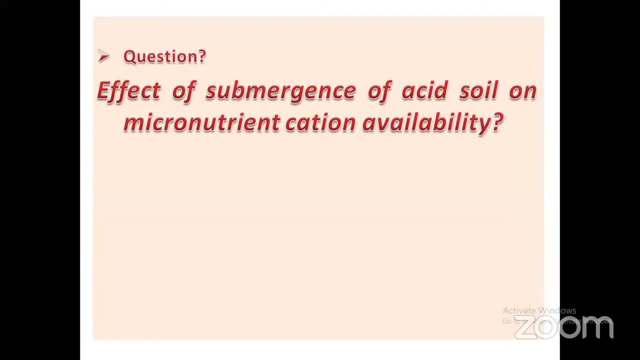 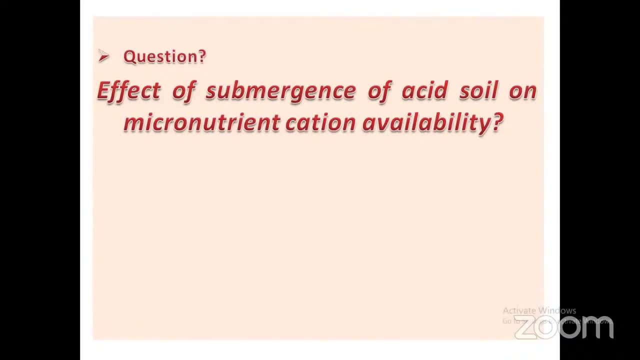 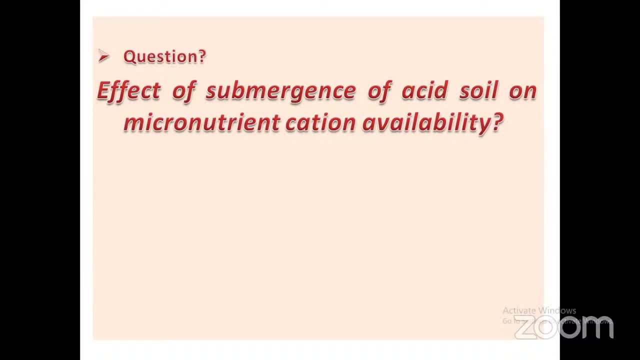 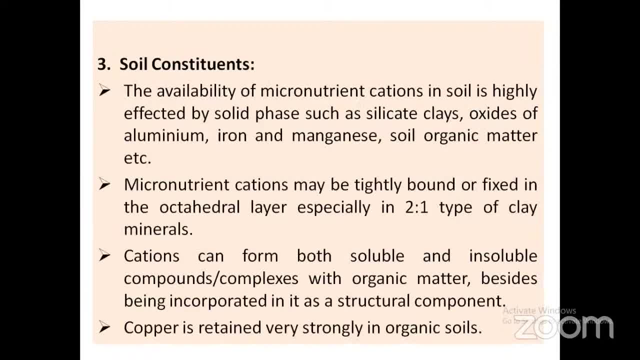 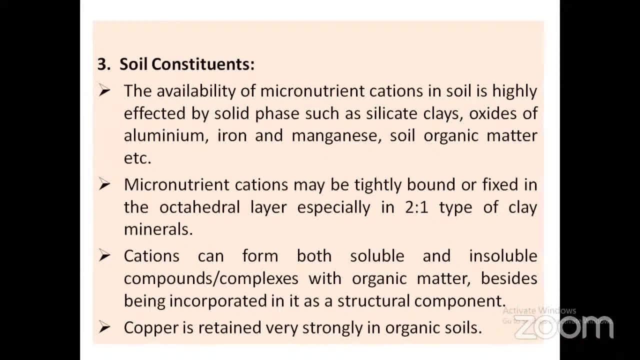 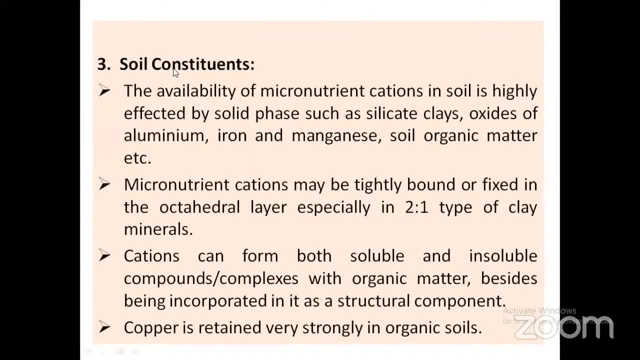 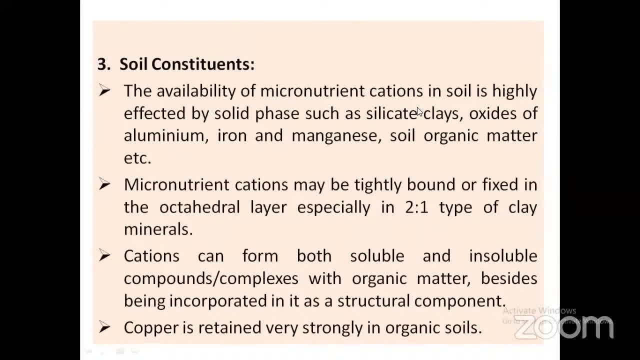 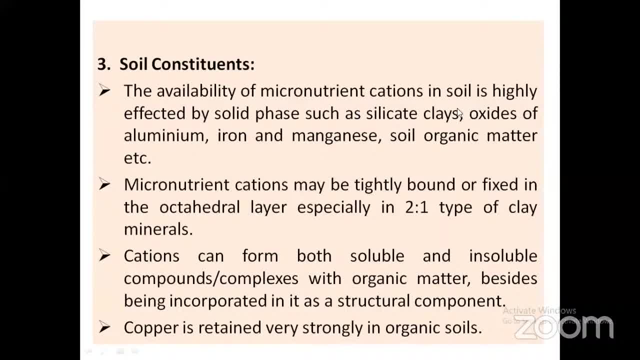 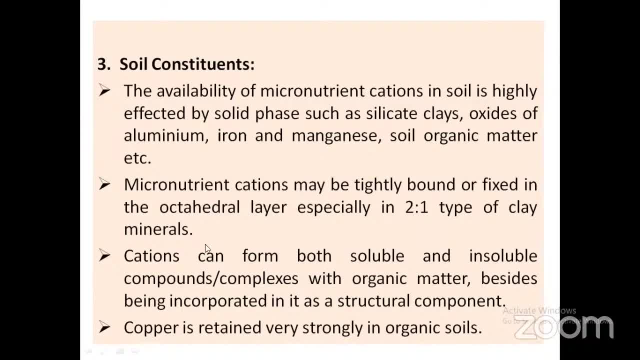 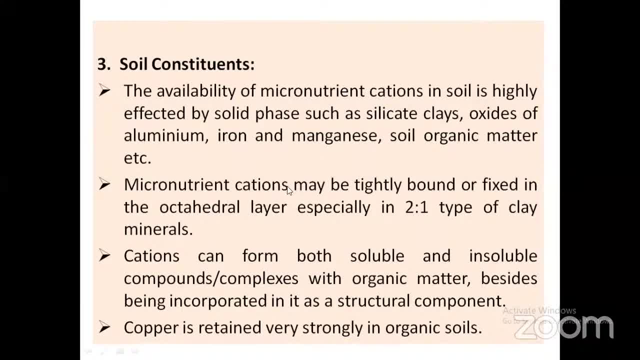 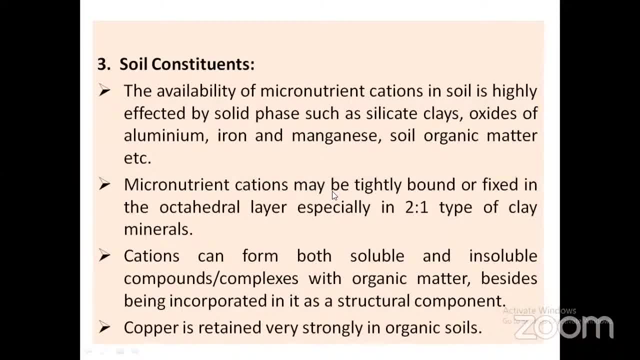 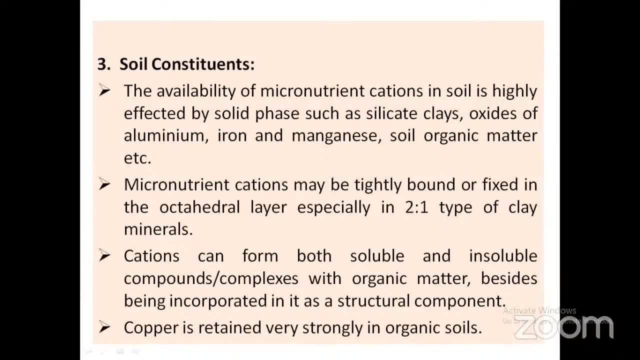 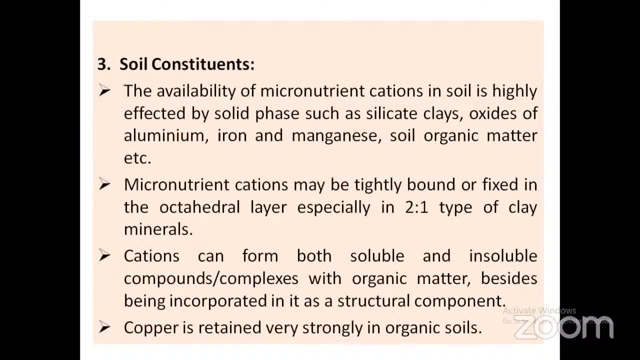 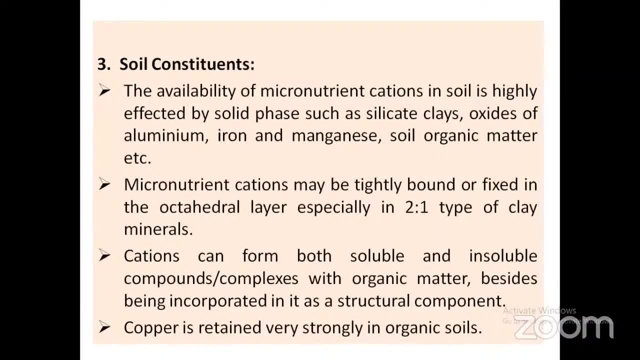 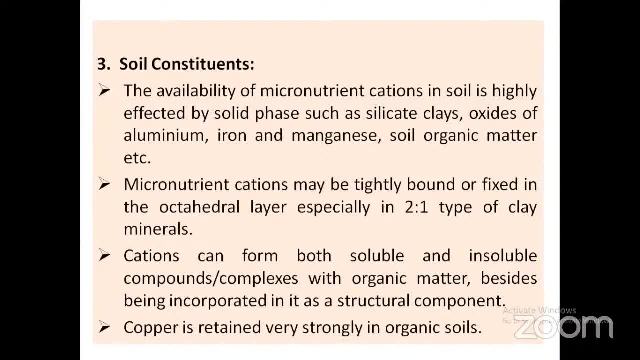 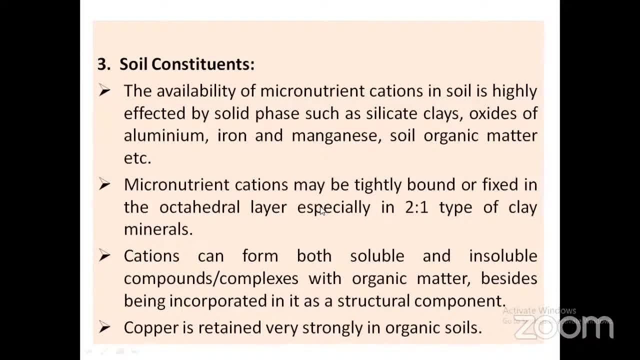 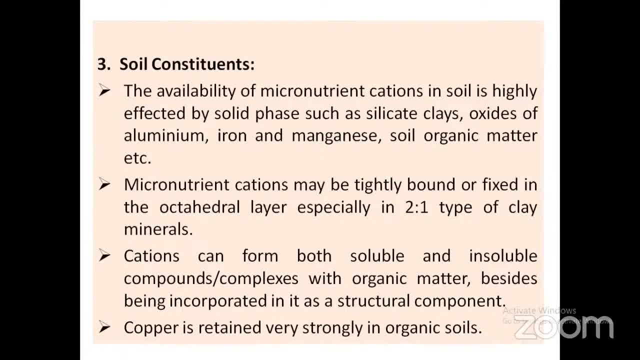 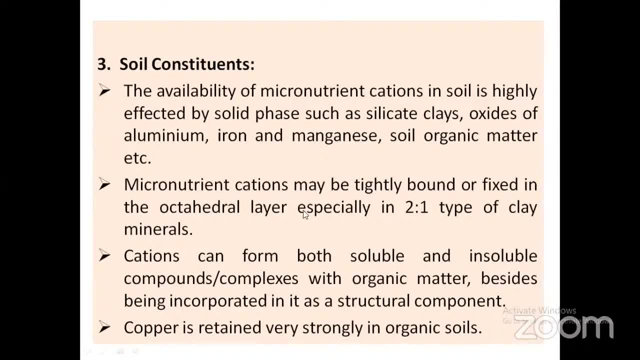 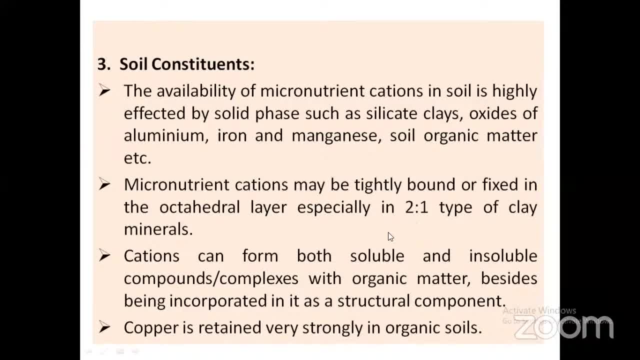 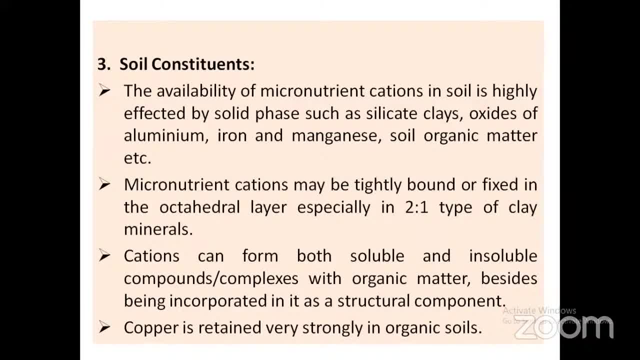 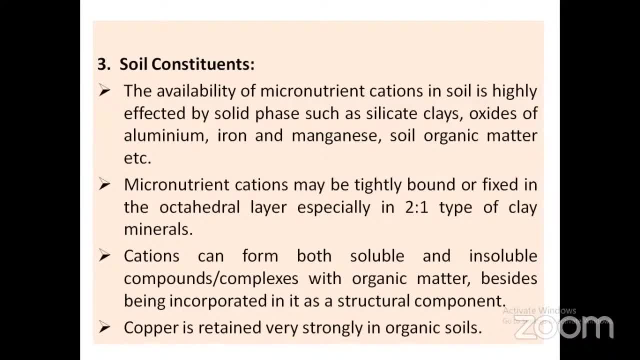 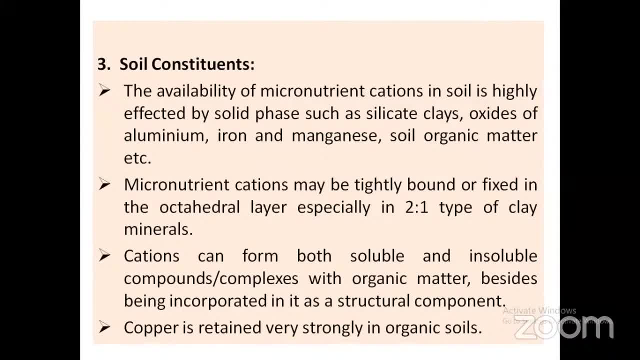 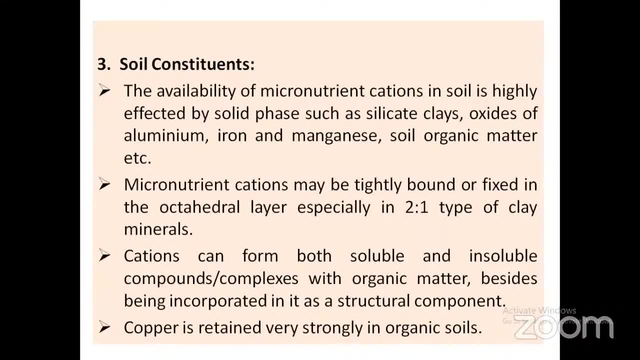 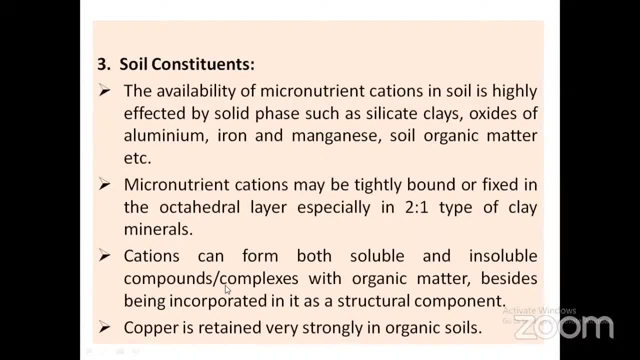 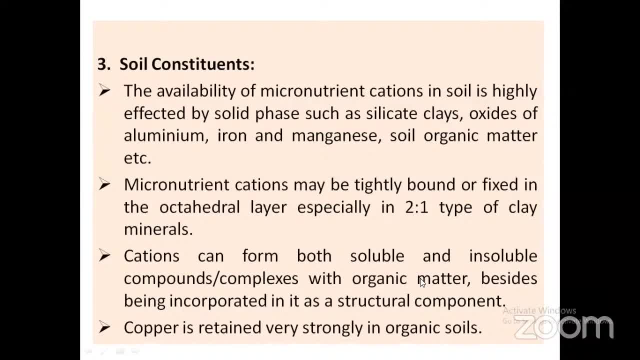 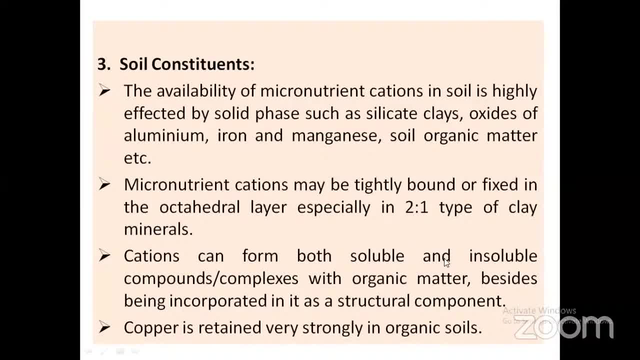 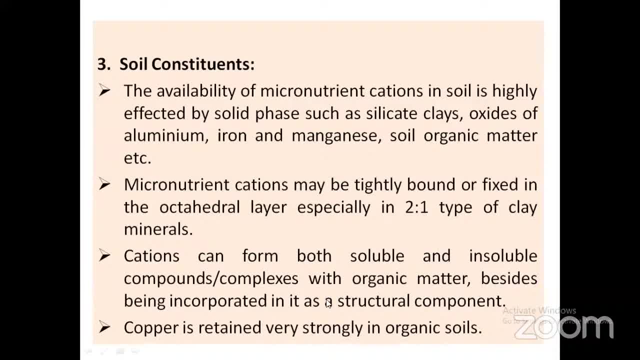 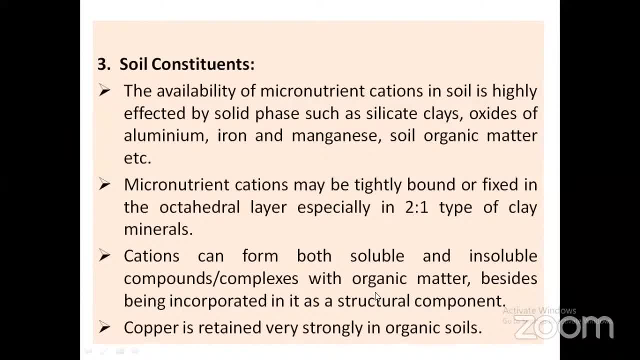 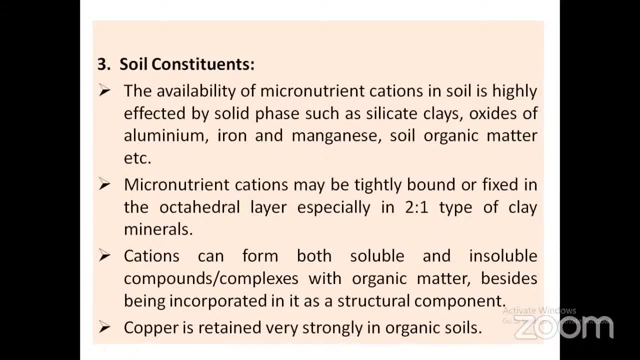 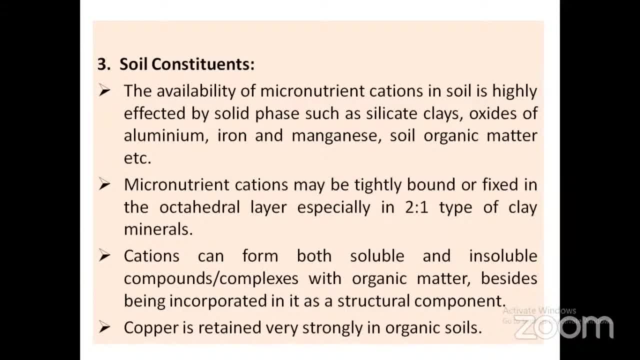 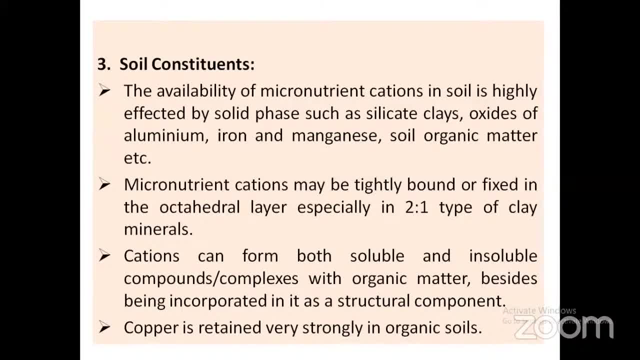 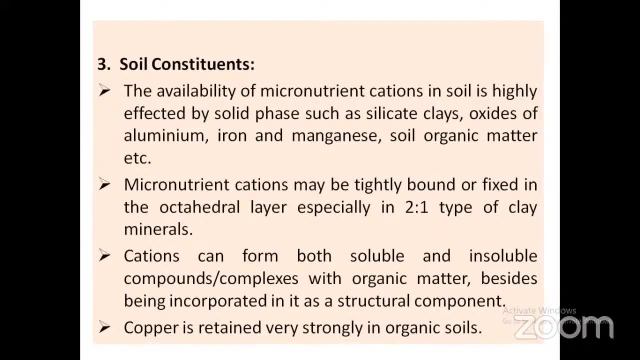 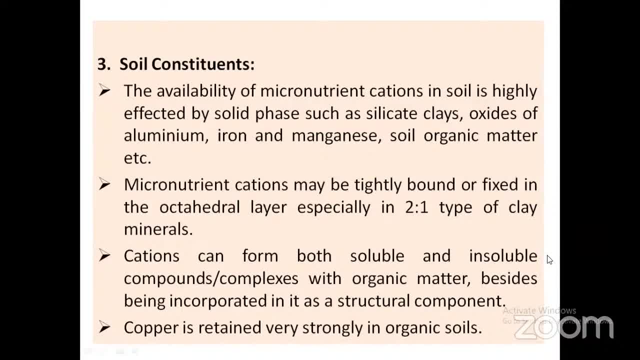 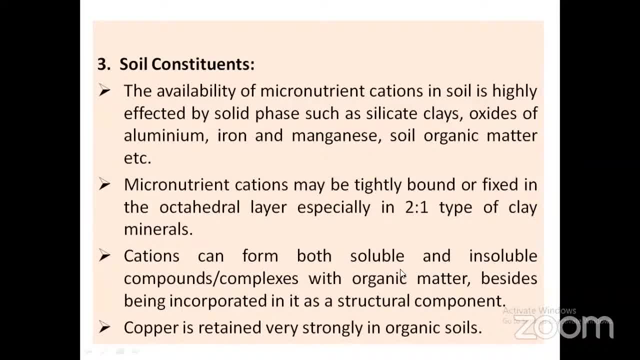 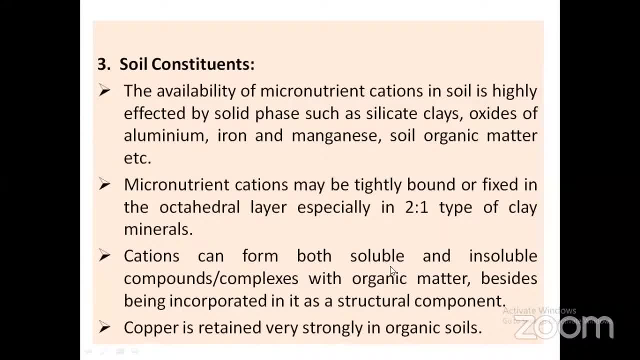 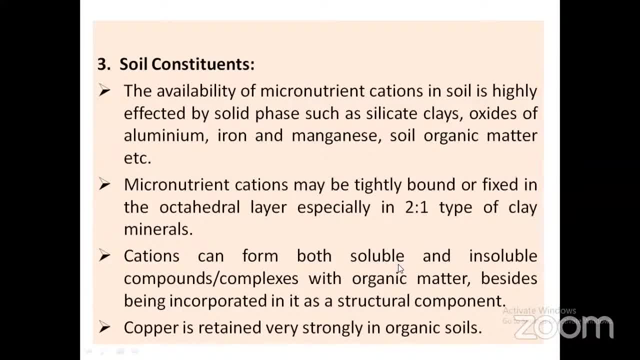 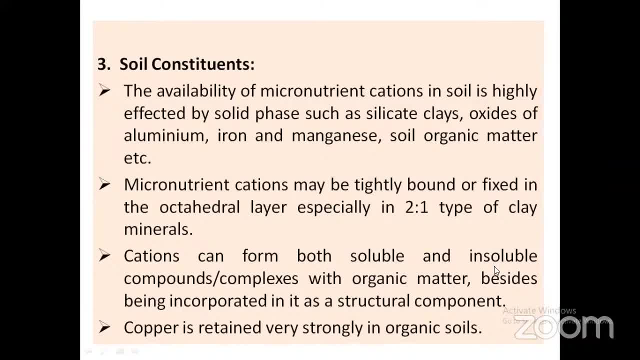 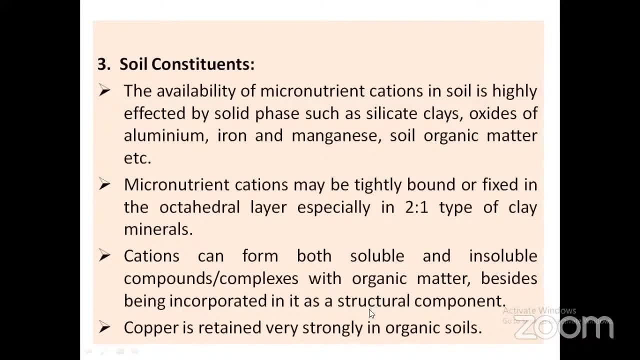 On the other hand, dissolution of iron manganese oxide enhances the solubility and availability of micronutrient cations, with the reduction of redox potential. On the other hand, sodas, natural materials and altre Tele存 Gazib are found in minerals such as copper and magnesium. 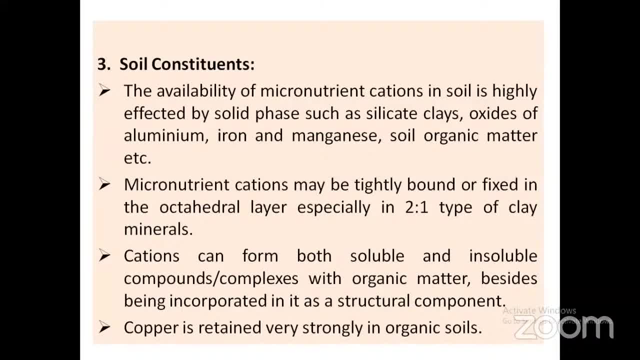 On the other hand, sodas, natural materials and altre Tele存 Gazib are found in minerals such as copper and magnesium. weetened verdice Produced from cement describinged as transcendent. Peter Cching staff, Ken Murtir 2018. Kate. 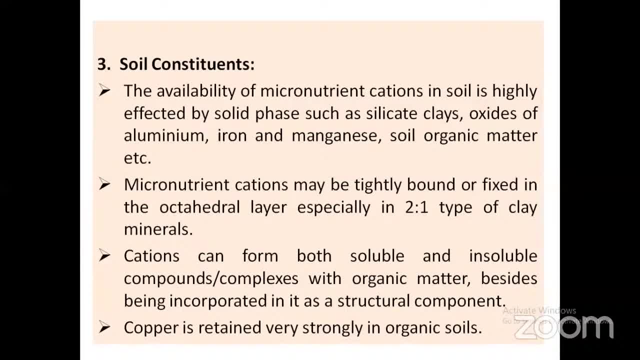 Dangerous Pi Tomorrow, Richard. insoluble compound. that is why reclamation disease we have started. so copper is retained very strongly in the organic soil. so this is how this organic matter influence the availability of cations. now moving ahead to the effect of these factors on the availability of anions. 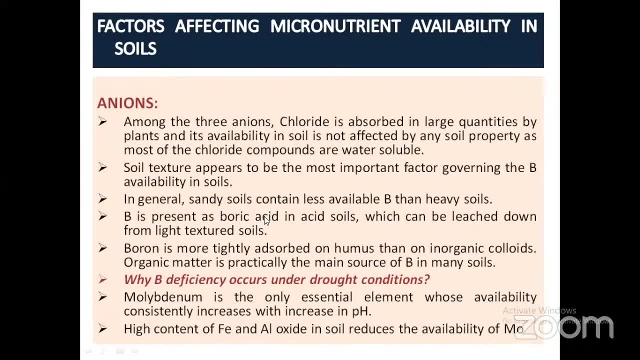 so, among the three anions that we have started, chloride- three anions that we have studied, that is, chloride and molybdenum, and another is which one boron. so, among these three anions, chloride is absorbed in large quantity by the plants and its availability in soil is not affected by any. 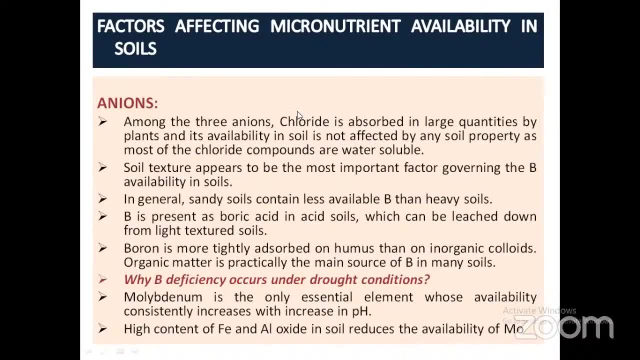 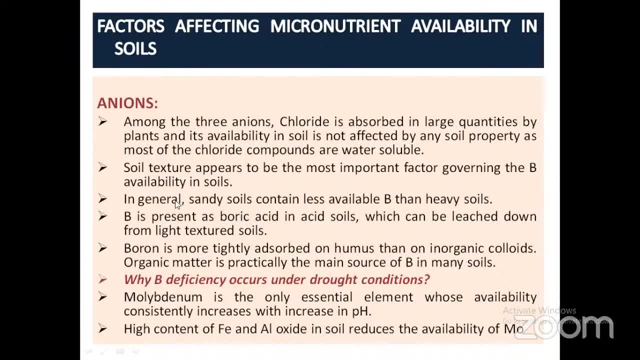 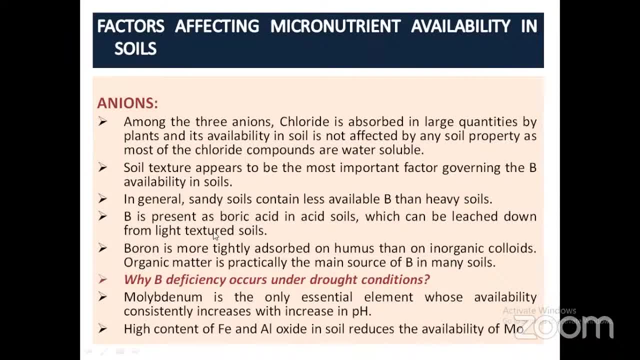 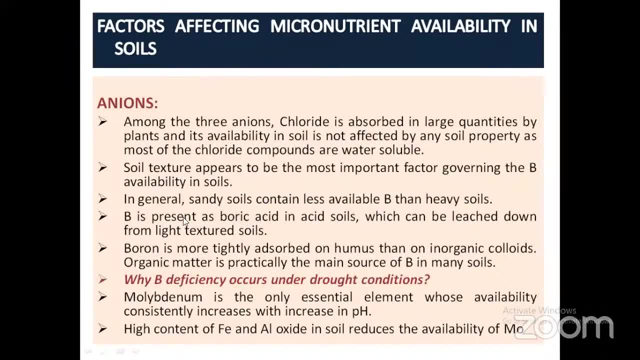 So the loss of boron is more in sandy soil, So it is less available In sandy soil because of its leaching, and boron is more tightly absorbed on humus than on inorganic polyols, So organic matter is practically the main source of boron in many soils. So boron is 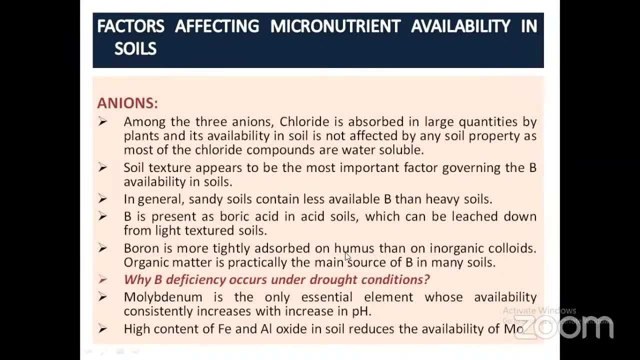 absorbed on the humus and as soon as the decomposition of this organic matter occurs, there is availability of boron. Now why boron deficiency occurs under drought conditions. I am telling you that under drought conditions there is deficiency of boron. Now you tell I 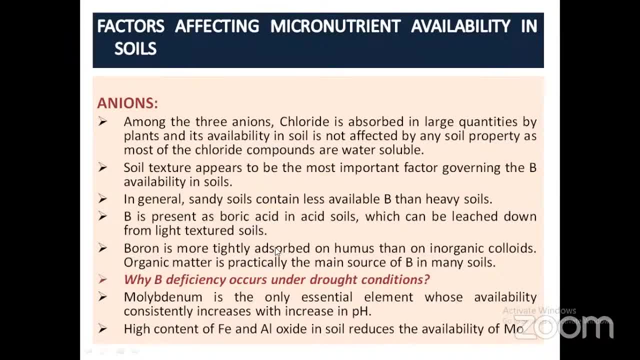 have told you the reason already In saare points mein. iska reason hai Toh koi mujhe batayega Why there is deficiency of boron under drought condition. Ma'am, to reduce mineralization. Yeah, Mineralization of what? 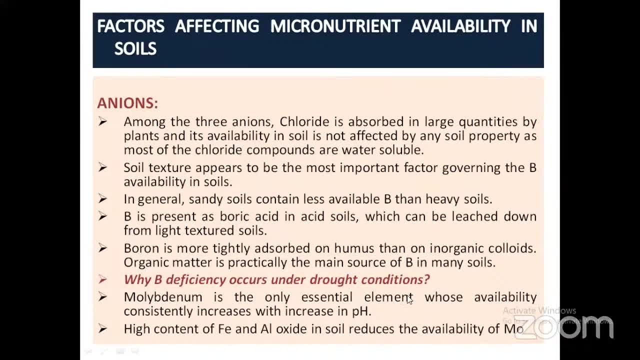 Okay, you see, I told you that organic matter is practically the main source of boron. So in many soils there is deficiency of boron. So in many soils there is deficiency of boron in many soils because boron is more tightly absorbed in the humus right. So 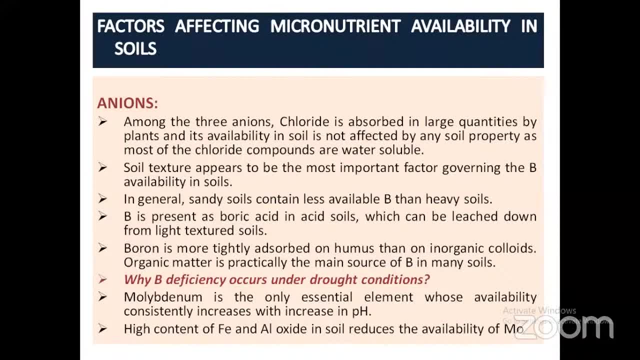 under drought condition, boron deficiency in the plant is observed due to reduction in organic matter mineralization and uptake by the plant. Isse liye drought condition, mein boron ki availability, kam hobi Choki. organic matter ka decomposition nahi ho paega. Another is molybdenum is the only. 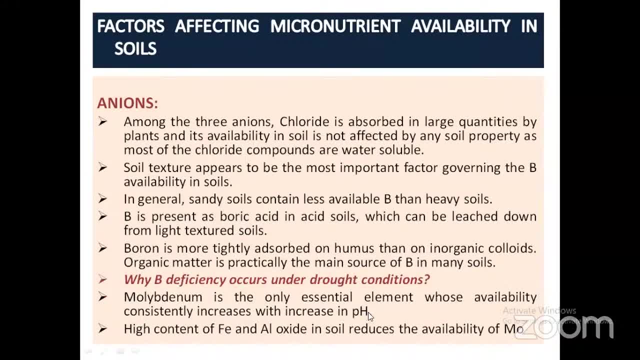 essential element whose availability consistently increase with increase in the pH. pH badne se molybdenum ek akela element hai NekBen gusto kite peshi hai cik hai. high content of iron and aluminum oxide reduces the availability of molybdenum. 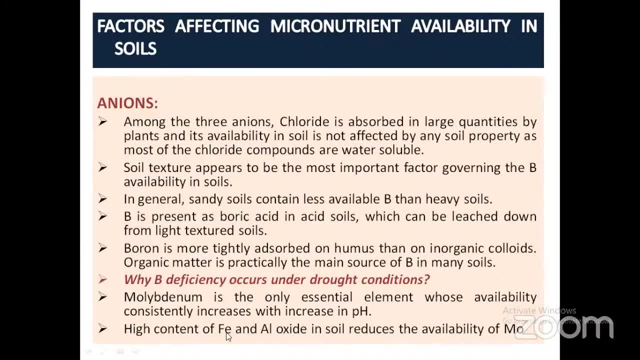 Why molybdenum is less available in acidic range because of iron-aluminum oxide. Molybdenum gets fixed in iron-aluminum oxide as well on silicates at low pH through ligand exchange. That is why this availability of boron is less is less under acidic range and high under at high pH. 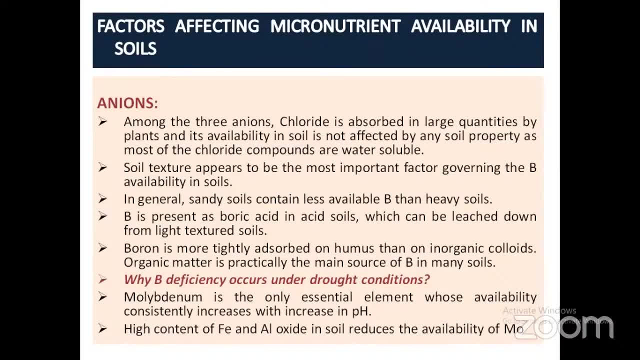 получается verban Gefx. That is why this availability of boron is less in acidic range and it is less under high pH typhians. that is why you can learn坐. changes of highlight rates at train are less- less under acidic range than under. molybdenum is less under acidic range than it is higher than it is higher than iron and aluminium oxide feel better. also very good source of acid. Technical advantages. 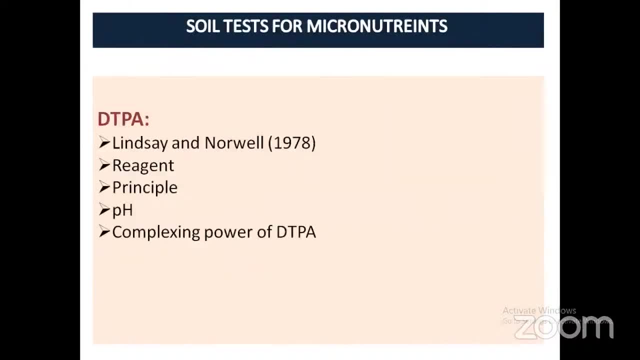 pH. Okay, Now coming to soil testing method for this: micronutrients. So I'll tell you a little bit brief about this DTPA: the process, the functions and the principle on which DTPA actually works. So you tell me what is the full form of DTPA? Yes, So it is diethylene. 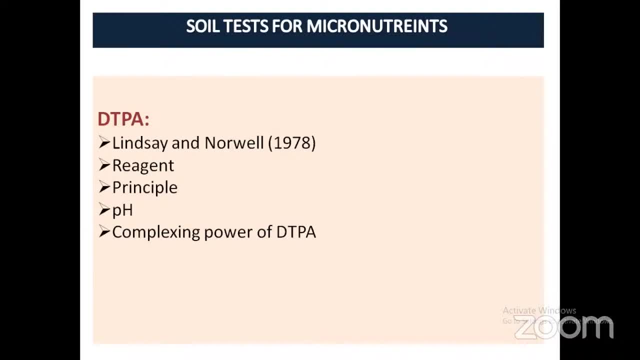 triamine pentacetic acid. This is an extracting reagent for micronutrients, right? So DTPA is an extracting agent, reagent given by Lindsay and Norville in 1978.. So DTPA is given by Lindsay and Norville, very frequently asked 1978, and the reagent it is not only DTPA. 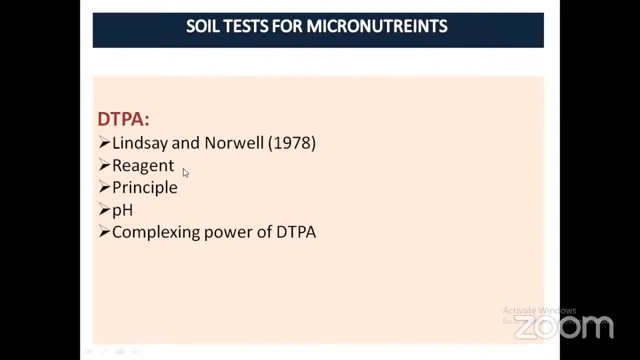 there are two other reagent along with DTPA. So reagent: you write. this is frequently asked in exam. You write 0.005.. molar DTPA: 0.005 molar DTPA plus 0.01 molar calcium chloride dihydride: 0.01 molar calcium. 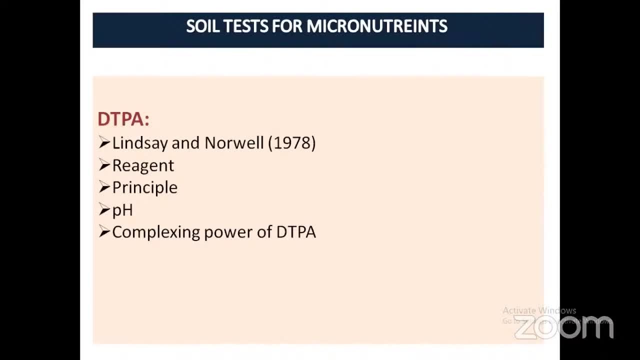 chloride dihydride plus 0.1 molar T triethanol amine, So I'm repeating 0.005 molar DTPA plus 0.01 molar calcium chloride dihydride, So I'm repeating 0.01 molar calcium chloride dihydride plus 0.01 molar T triethanol amine. 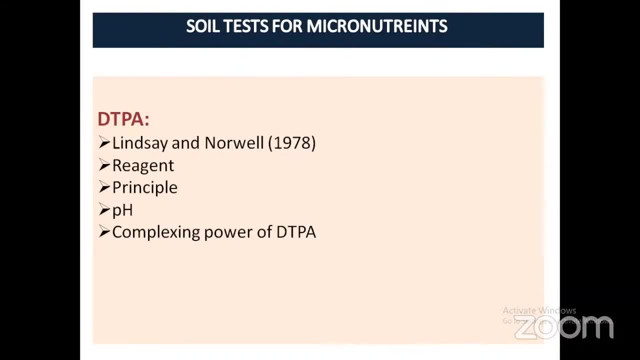 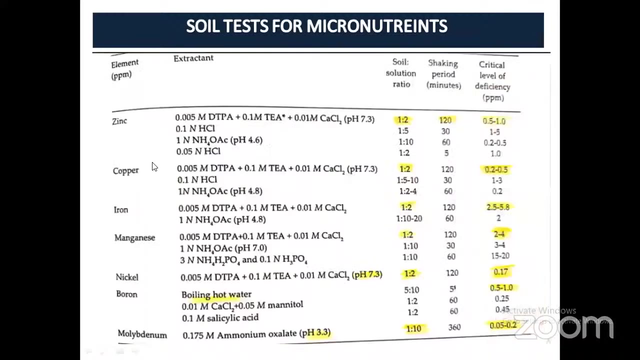 Written, all of you. If there is one, I can write it down and tell you: Yes, Okay, Now the pH, pH at which this DTPA works. it is 7.3.. Okay, So Lindsay and Norville has. 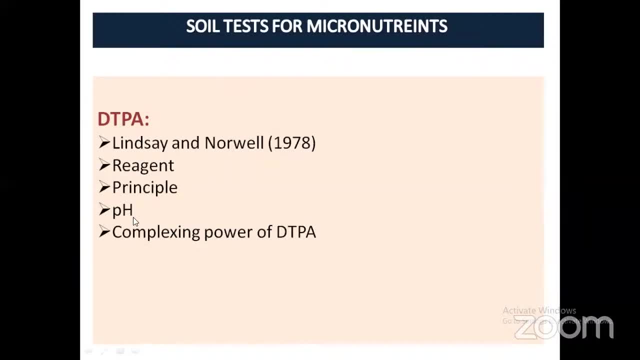 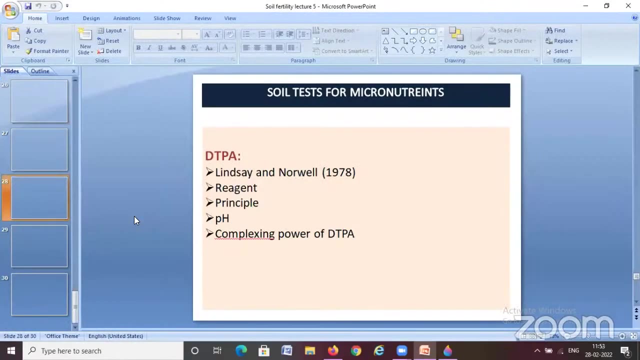 given this reagent. I told you it is DTPA, calcium chloride. pH is 7.3.. Okay, Very frequently asked question. Now we'll see the principle on which this DTPA works. Okay, For that, there is an option of whiteboard. Where is it? 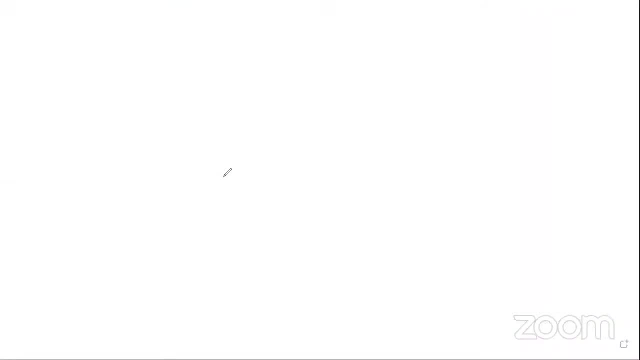 Ma'am, you take some blank page, then you take the pencil. ma'am, Yes, Okay. So I'll tell you the principle on which DTPA works. Okay, So you see, we know that there is solid phase. There is solid phase in soil right, And there is solution phase. 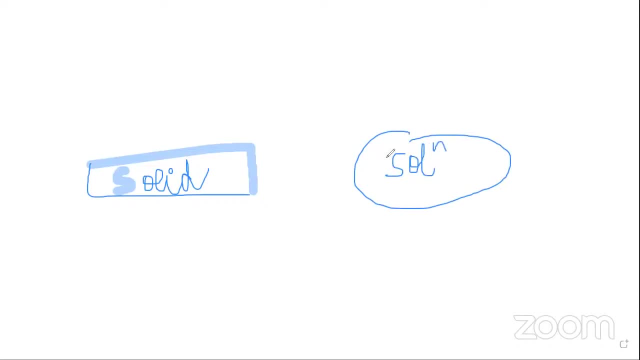 So plant takes nutrients from which phase? Directly From solution, Solution. So plant takes nutrients. This is our plant, So this is our plant. It takes nutrient from solution. And if from solution- soil solution- particular nutrient is taken up by the plant, then it is replenished from solid phase. 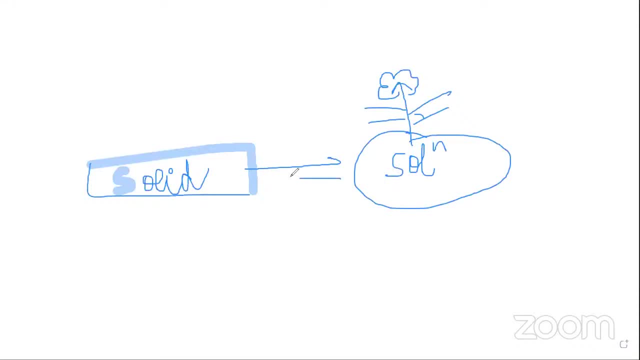 So where it will come from? From solid phase, From solid phase. And if we put any fertilizer in the solution phase, if it is more, then it will go to the solid phase. Do you understand this much? Yes, ma'am. 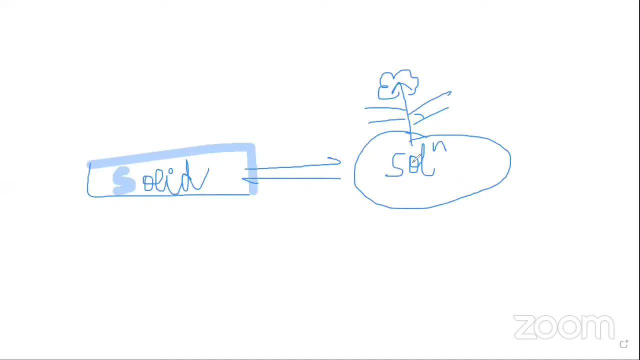 So this solid phase is actually replenishing whatever nutrient is taken up by the plant from the solution phase. This is one thing. Now you see, if we are adding DTPA in soil solution, we are putting DTPA. What is this DTPA? 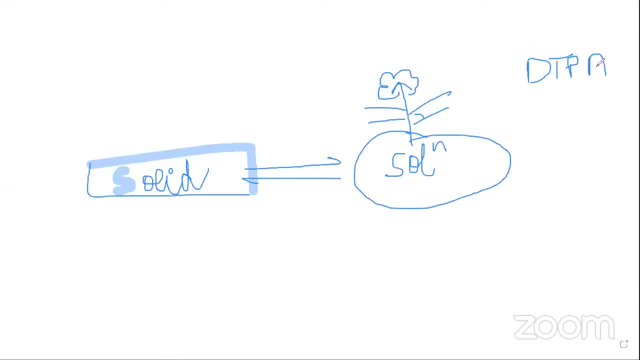 DTPA is a chelating agent. Chelating agent means which can bind any nutrient Like a bird's claw. Chelate term comes from the claw word, which means just bind it, Make it complex, Chelate it. 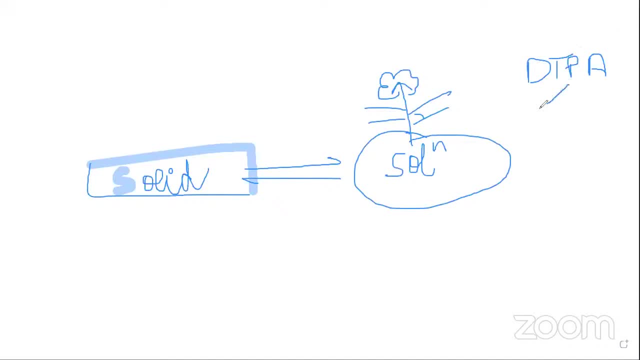 So this DTPA is a chelating agent. If we add this DTPA in the soil solution, what this DTPA will do? This will bind the micronutrient. This DTPA will chelate the micronutrient. 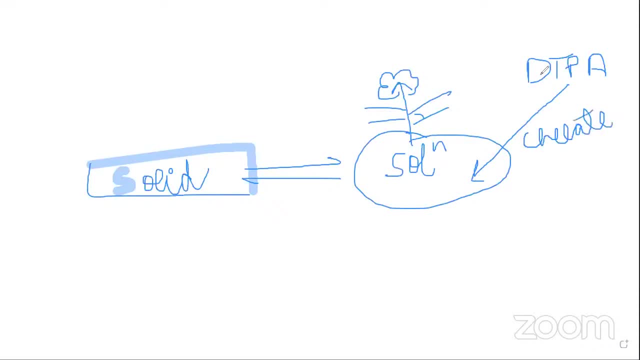 And if this DTPA will chelate this micronutrient, then the concentration of micronutrient in solution will be less. So where will it come from? If there is less in the solution, then where will the nutrient come from? 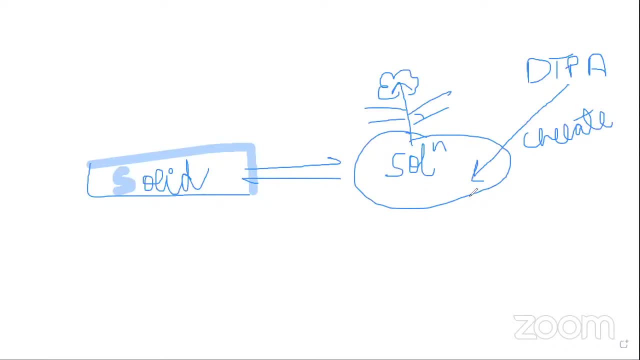 From the solid phase, From the solid phase. So one thing is, if plant take up this micronutrient from the soil solution, it will replenish by the solid phase. This is one Another is if we are adding DTPA, DTPA will bind the micronutrient. 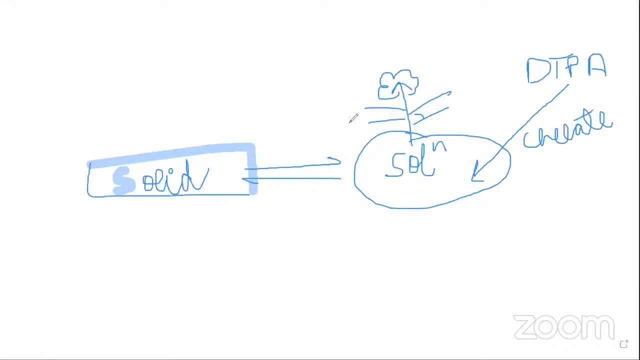 And the evaluation. The variability of particular micronutrient to plant will not be there and it will be replenished by the solid phase. Okay, So the principle on which DTPA works. it says that the chelated micronutrient 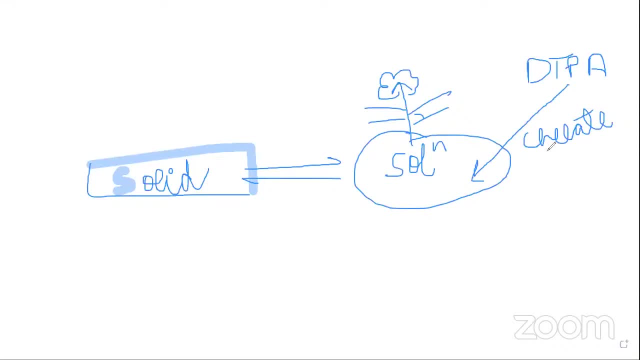 the micronutrient that DTPA has chelated. it will lose its ionic form, as if absorbed by the plant roots. The micronutrient that DTPA has chelated will behave like the plant has uptaked it. The solid phase does not know whether the plant has taken it or the DTPA has binded it. 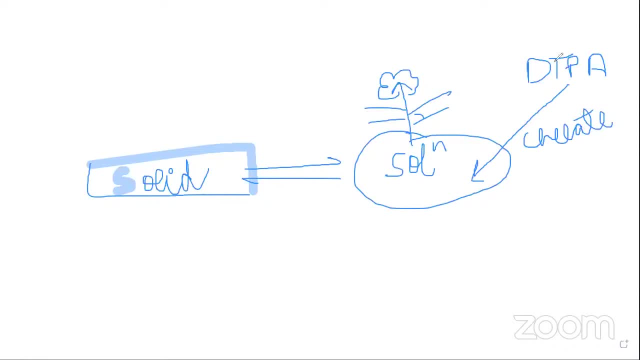 It just means that it is less than the solution. So DTPA works on the principle that whatever the nutrient is chelated by the DTPA, it will mimic as if it is taken up by the plant. And if the plant is mimicking this, then the solid phase also releases micronutrients in the solution. 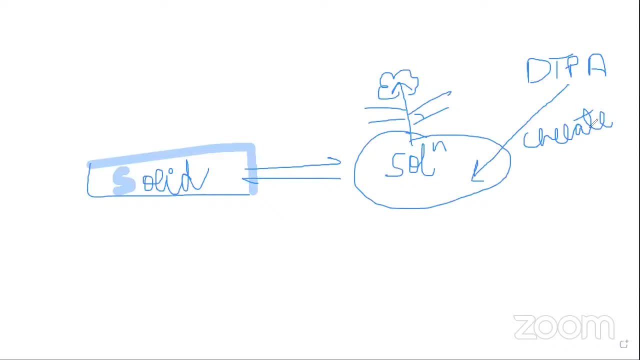 Now, whatever micronutrient is in the solution, DTPA has chelated it and we can find it out. So what is the principle? If the nutrient is less in the solution, then it will come from the solid phase. And how will it be less in the solution When the plant will uptake it? 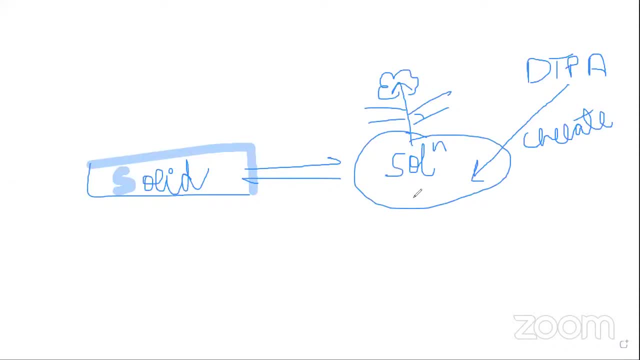 So if the plant is taking nutrient from the soil solution, it will be replenished by the solid phase And, because of DTPA, it chelates that particular micronutrient, binds it and behaves as if the nutrient is taken by the plant. 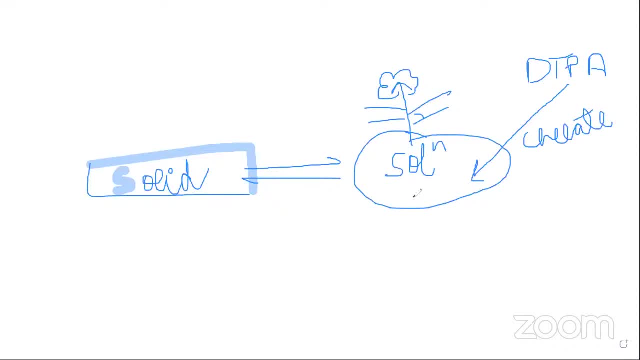 And if the solid phase feels that the nutrient is less in the solution, then it will give it back to the solution and DTPA will bind it again And DTPA will tell us how much nutrient is in the soil. Is it making sense to all of you? 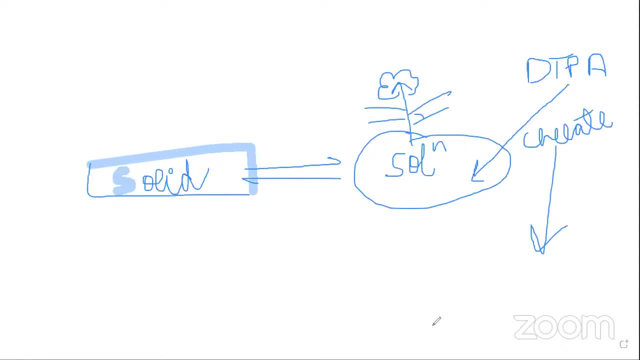 Yes, ma'am, Ma'am. ultimately, how will we measure it? DTPA will take reading from double layers. DTPA has to bind whatever nutrient is there And whatever DTPA has bind, it will take reading from double layers. 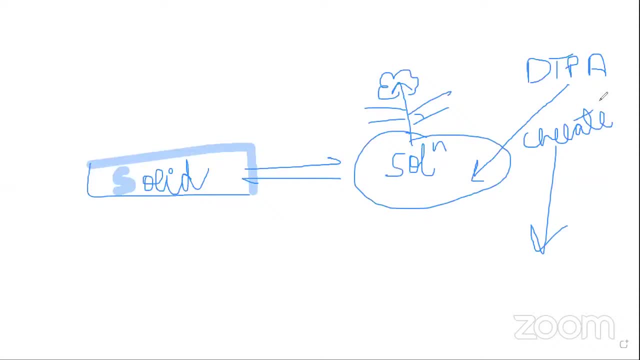 DTPA is only an extracting agent. Whatever is there in the solution, it will take out the micronutrient from it, And the rest of the reading has to be taken from double layers in atomic absorption. Is it making sense? So, ma'am, actually we are trying to find out which micronutrient is there in the soil. 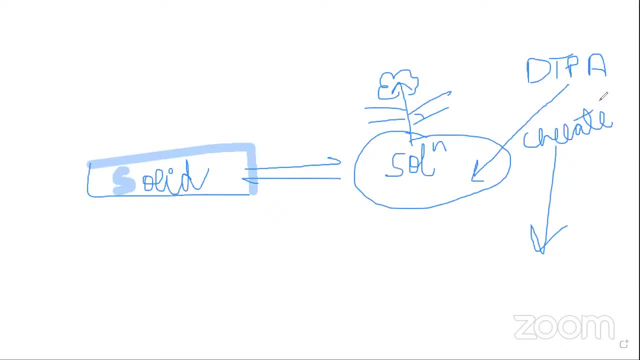 How much is there? Who is there and how much is there? We are also trying to find out the amount. And one more thing: The purpose of this experiment was that you understand two things: Intensity factor and quantity factor. Yes, ma'am. 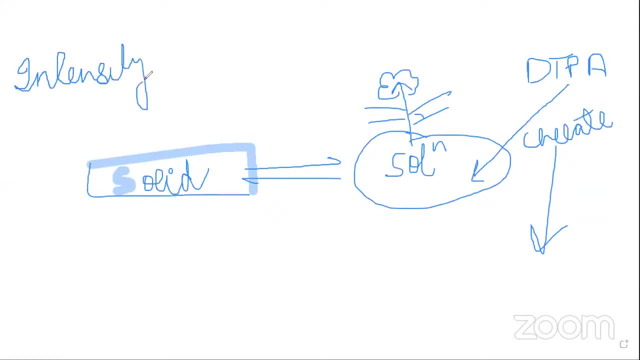 What happens? Tell me, Intensity is the concentration of a particular nutrient in the soil solution And there is the ability of the soil to maintain that concentration. How to replenish that So we can say that quantity factor is whatever is there in the solid phase is quantity. 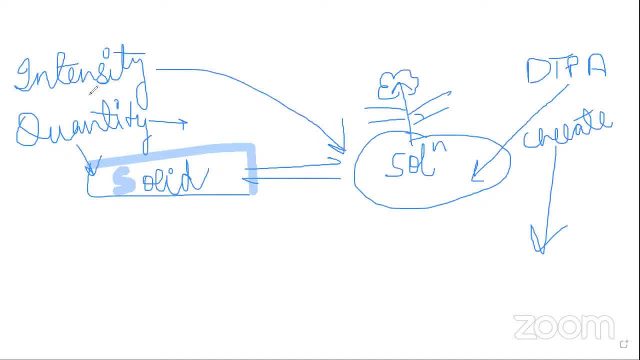 Intensity factor. is this solution? Please mute your mic. Just say what you want to say and then mute it. So this quantity factor is whatever there is in solid phase and intensity is there in solution phase. And I said that DTPA has already binded the solution. 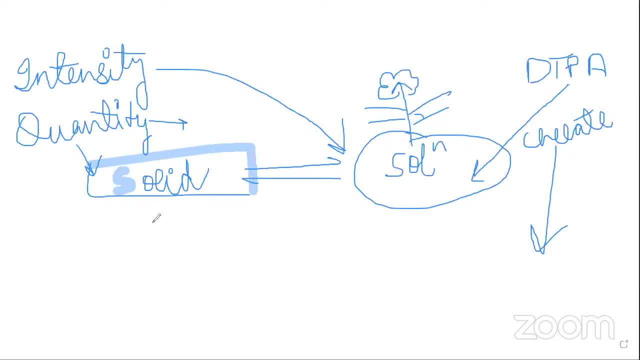 Then mimicked that the plant has taken it and then the solid phase has also given it here. So DTPA is actually estimating both intensity and quantity. It gives not only initial concentration but also quantity factor related to labile pool. It takes into account both intensity and quantity factor. 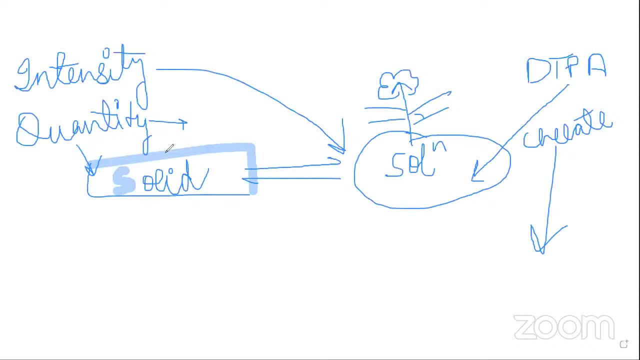 Is it making sense to all of you? Yes, Ma'am. repeat once again the last line. Okay, Tell me what you have understood in the principle till now. Ma'am, What's your good point? Ma'am, What's your good name? 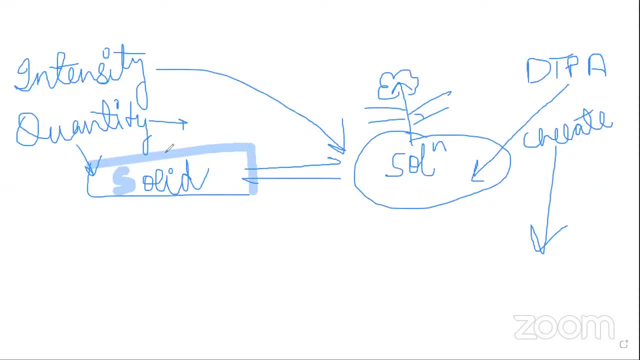 Ma'am, Hrithik Kumar. Hrithik, You say, Ma'am, As DTPA is a chelating agent, We put it in soil solution, So from there it absorbs the micro-nutrients It chelates. 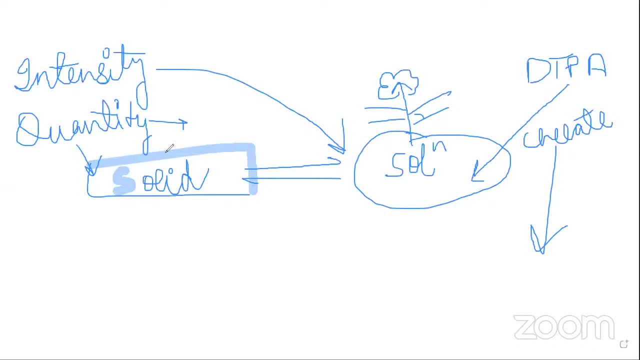 So it chelates in the soil solution. So to replenish the micro-nutrient in the soil solution, the micro-nutrient comes back And then we can absorb it. So this shows how much micro-nutrient is absorbed in the soil. 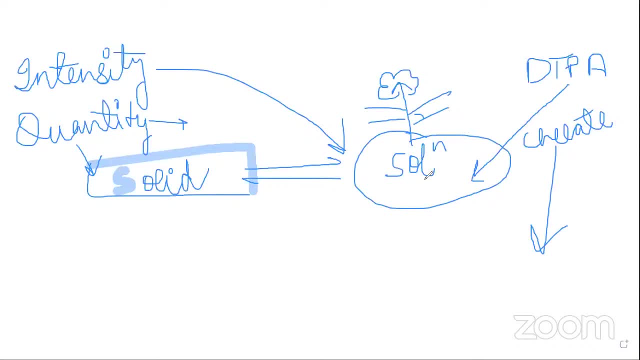 DTPA is absorbed. Okay, You are absolutely right, Just once. when you say this principle, you have to say this too: That DTPA is chelating micro-nutrient and behaving as if it is taken up by the plant. 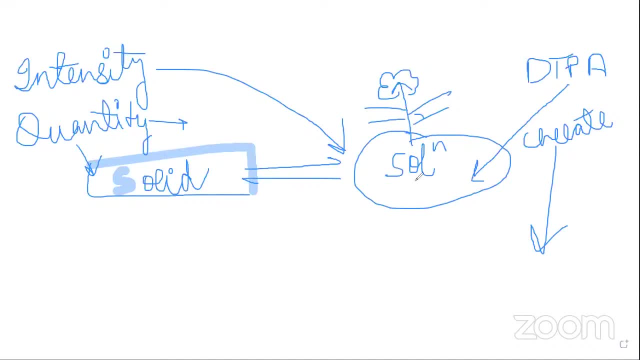 That's why it is replenishing from the solid phase, Because it is mimicking that. the plant has taken it. Okay, Now you said it yourself That DTPA has taken the solution And, because of that, whatever came from the solid phase, we also measured that. 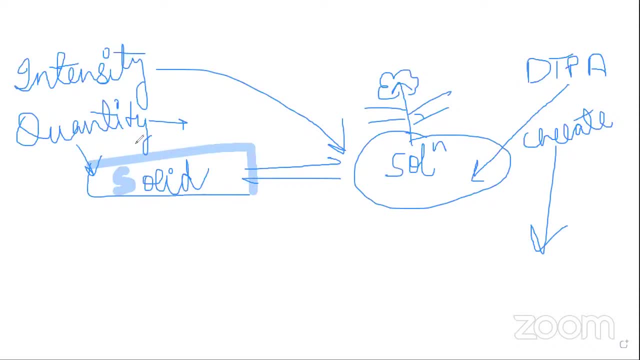 So DTPA method is actually estimating. It is actually estimating both intensity and quantity factor. This is what my last line was Making sense now, And quantity is on solid. Quantity is called solid phase, Which can replenish, Which is the labile pool. 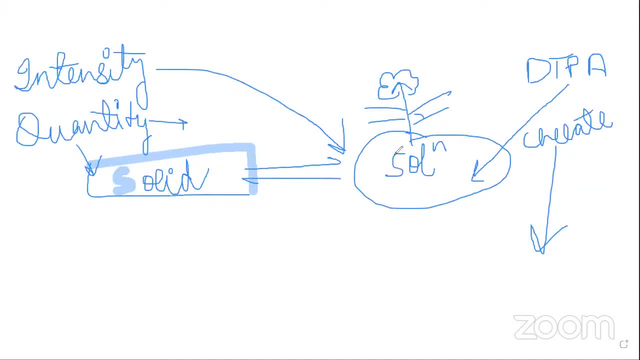 Which will replenish and come in the solution. So the solid phase also came in the solution. That's why we measured it too. Okay, Yes, ma'am. So DTPA measures both intensity and quantity factor. Any confusion, Any one of you? 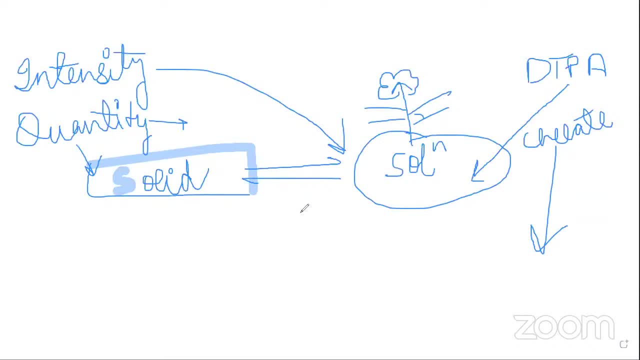 Yes Or no, Tell me, I won't know. if you stay quiet, Can I move ahead, All of you? Yes, ma'am. Okay, So we have seen. Yes, tell me. Does anyone want to say anything? I will delete this. 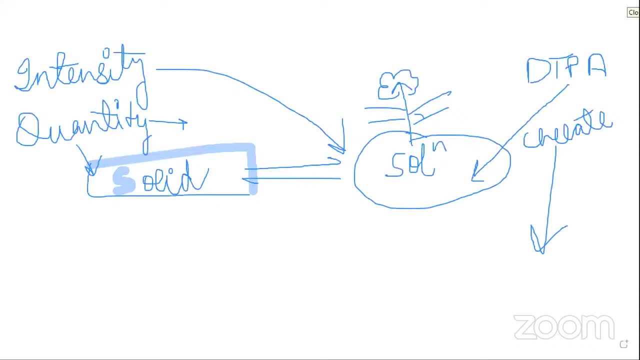 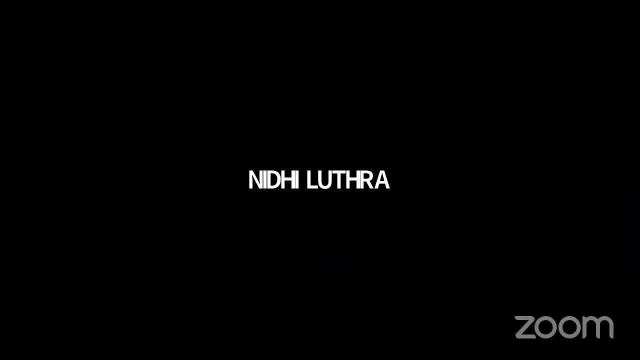 Then you can say it before this: Okay, I will delete it. No, no, no, Please go ahead, ma'am. Okay, fine, So we have seen that it is given by Lindzen Orwell. We have seen the reagent. 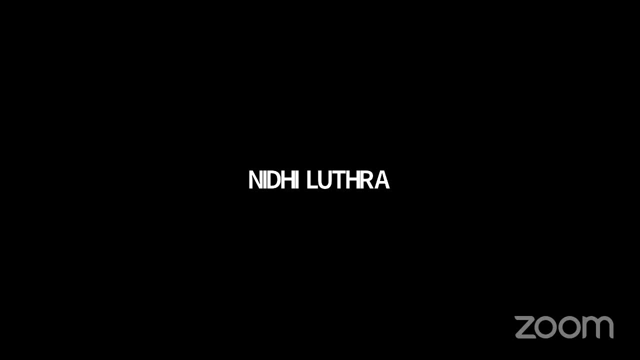 We have seen the principle, We have seen the pH, That is 7.3.. Now another is complexing power of DTPA, as this DTPA is the extractant for all the micronutrients. No, So how much micronutrient. 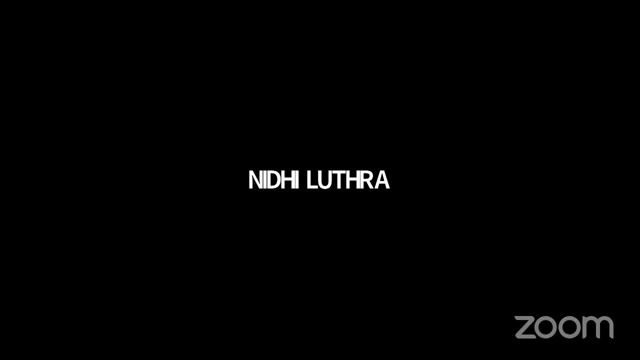 This particular Micronutrient, This particular DTPA, is able to complex. right, So you write: the complexing power of DTPA is 10 times, 10 times its atomic mass. So whatever micronutrient we are taking into account, suppose, if it is iron, 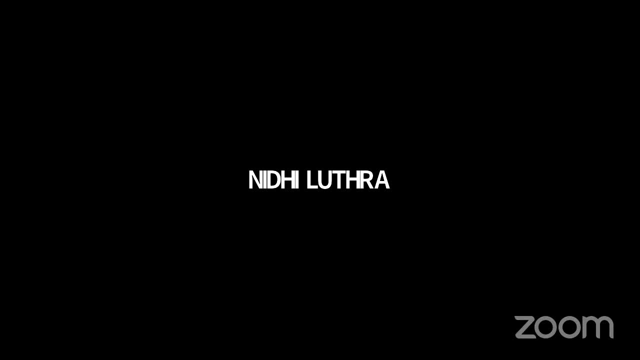 So iron is having atomic mass 55.. So 550 ppm of iron can be complexed with DTPA. Okay, So the complexing power of DTPA is 10 times its atomic mass, So iron atomic mass is 55.. 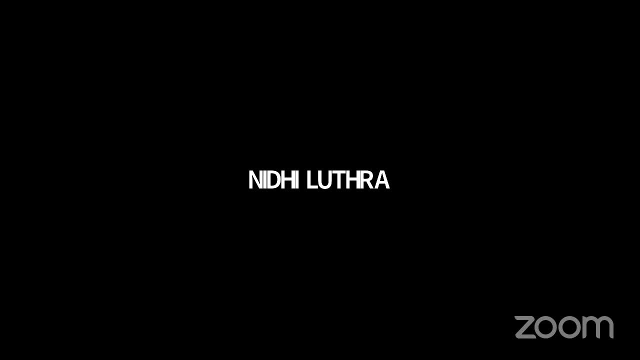 So 550 ppm iron can be complexed with DTPA. Manganese atomic mass is 56.. So 560 ppm of manganese can be complexed. Zinc atomic mass is 66.. So 660 ppm of zinc can be complexed with DTPA. 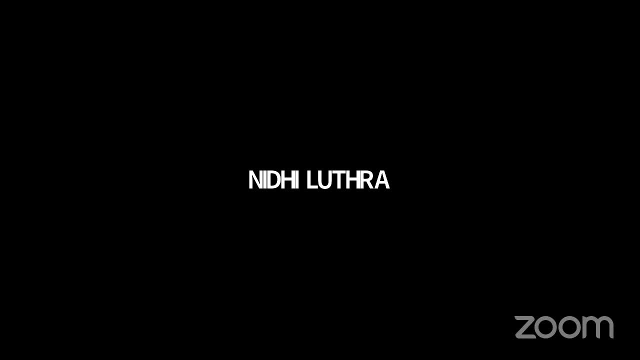 Copper atomic mass is 63. So 630 ppm of copper can be complexed. So DTPA is able to complex 10 times the atomic mass. Okay, Now moving ahead. Soil test for micronutrient. One of the extractant is DTPA that we have seen. 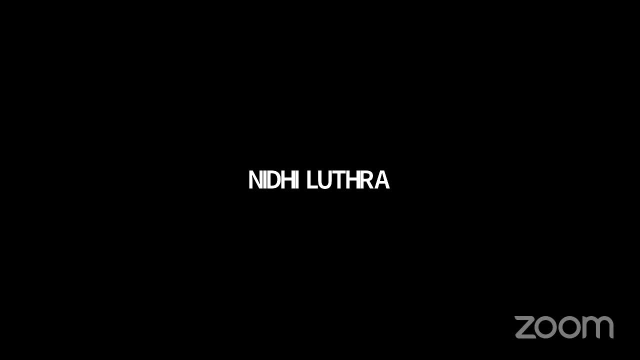 There are other extractants also. DTPA is common for all, But yes, there are other extractants also, Like for zinc, HCL, Bolo Slide start now. Okay, Wait, Okay, Okay, Okay Okay. 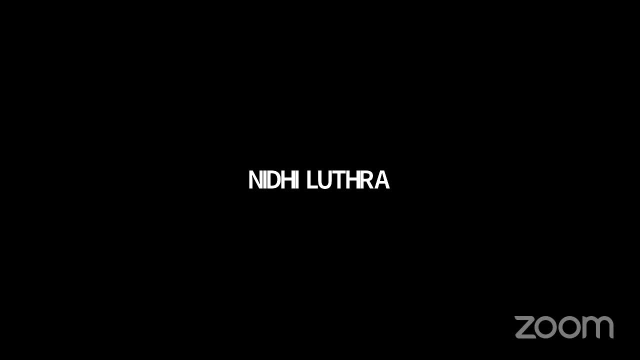 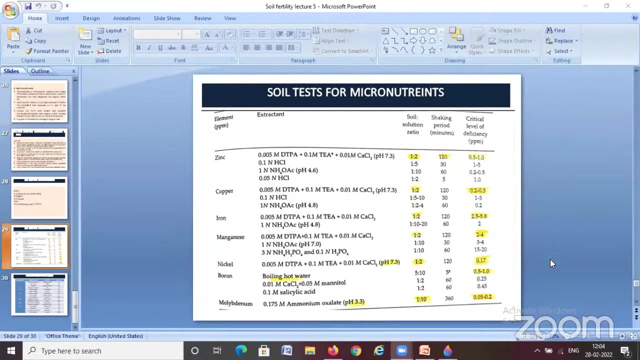 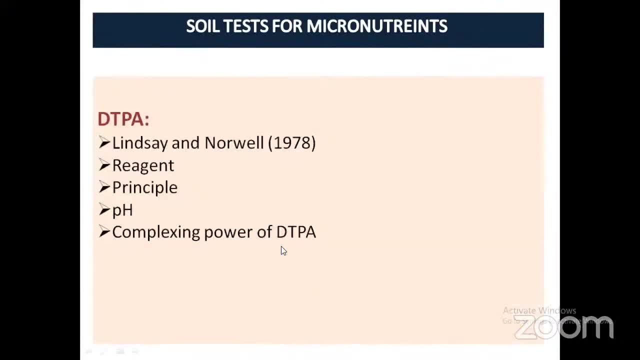 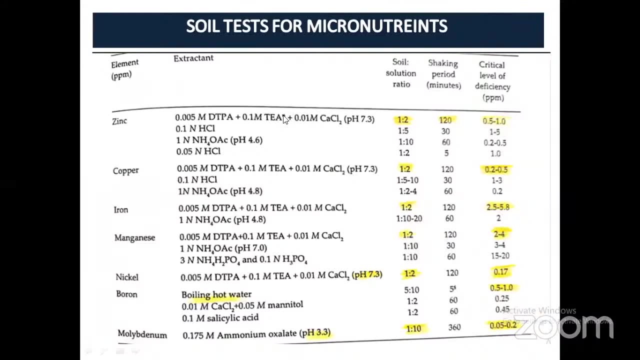 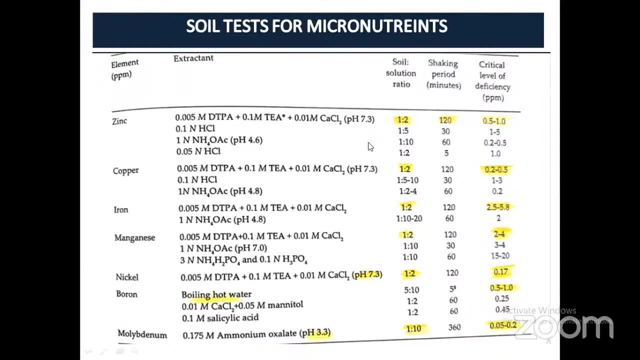 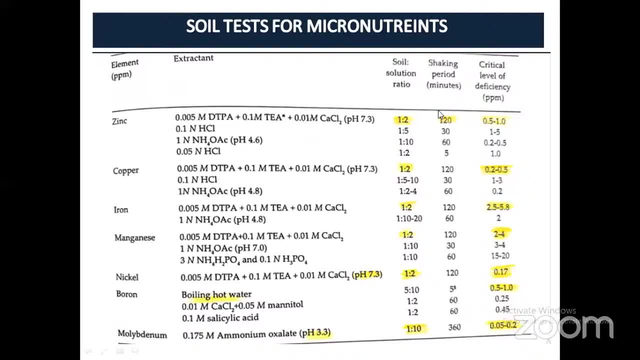 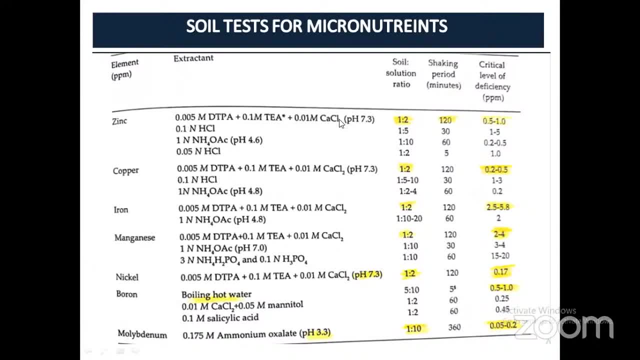 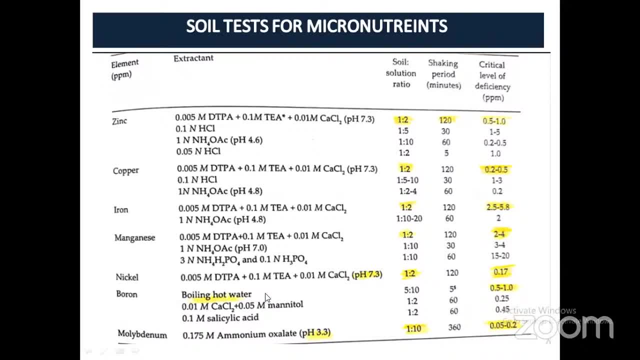 water method of boron, Berger and Trong. So it is by Berger and Trong this boiling hot water method of boron that is usually asked. Another is molybdenum. This molybdenum is extracted with ammonium acetate. What is this reagent known as Ammonium oxalate? 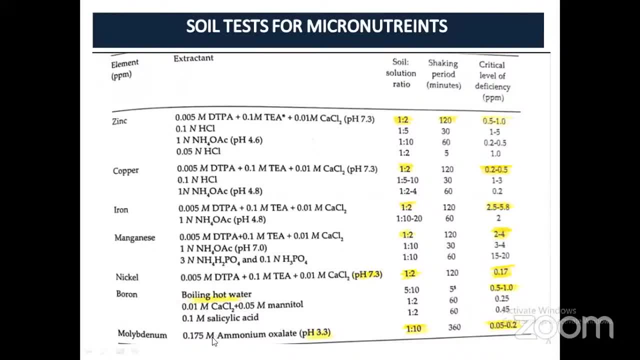 Any one of you? Hint for you. it starts from G Griggs reagent. Yeah, wonderful. So molybdenum is estimated by ammonium oxalate, which is Griggs reagent and the pH. you remember, it is frequently asked. 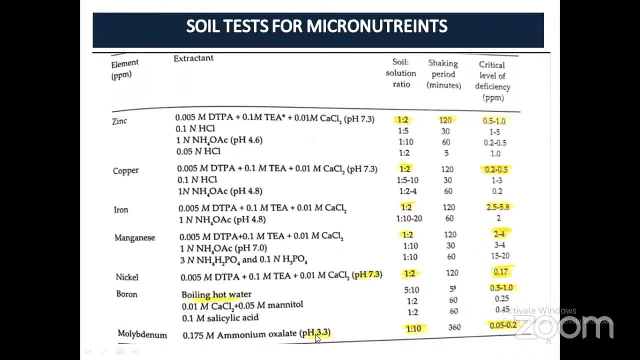 It is 3.3. So Griggs reagent is having pH 3.3 and molybdenum is extracted with ammonium oxalate. Griggs reagent Boron- you remember boiling hot water, Berger, and Trong nickel. 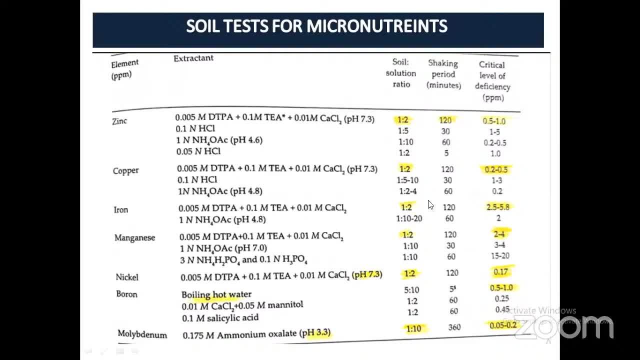 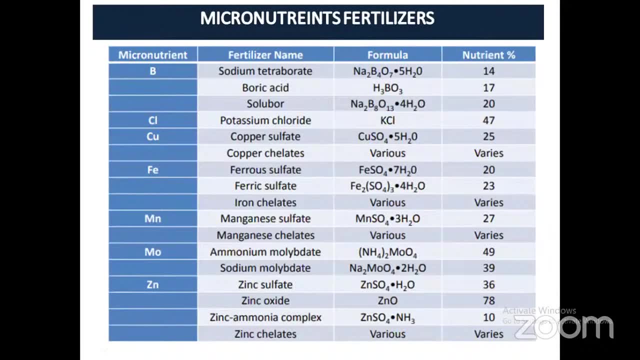 DTPA only. manganese, iron, copper, zinc. DTPA only. Okay, now let us move ahead. There are different fertilizers, Ma'am, yes, Ma'am, just like we use TEA with DTPA. what is the? 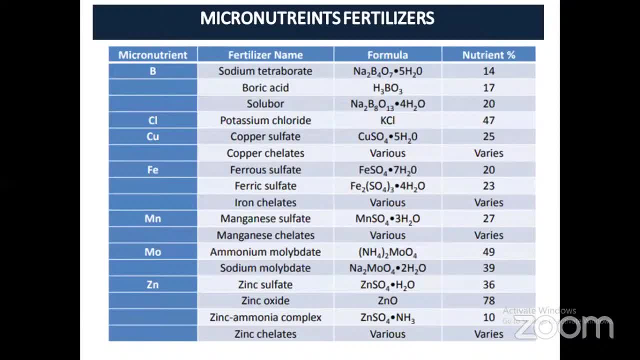 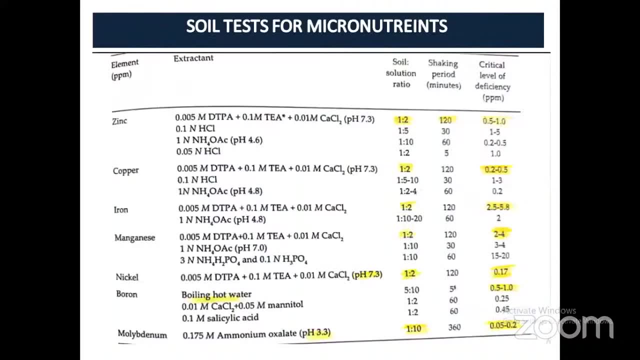 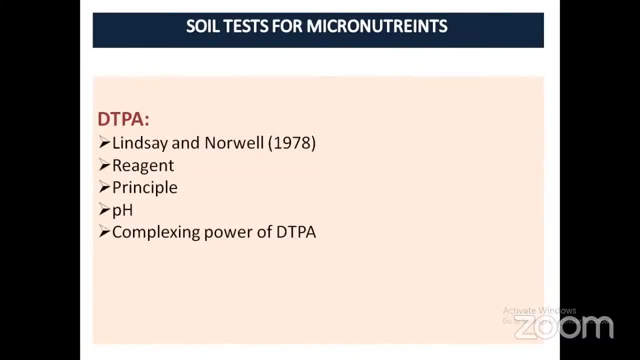 Okay, Okay, Okay, Okay, несanta, yes, No, no, we did not talk about calcium chloride. also, May I tell you why calcium chloride is added and why TEA is added. You see, this TEA is tri ethanol. I mean right. So the purpose of adding T is that it clearly burnt. 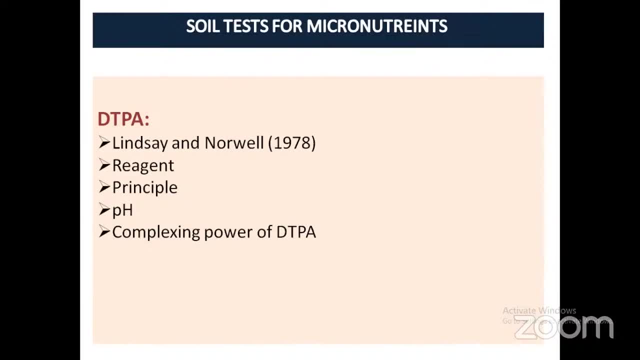 in the flame of double AS when we are cleaning, and then it burned. clearly. This is one of the reasons of adding T. Another is if flame wea is not disturb, Flame is not disturbed When TEA is added, so it fantastic. so if we are adding our instead of 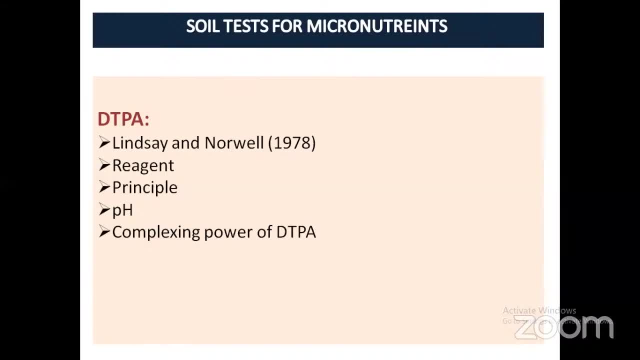 If we are adding our in our cocktail- and this is the explanation of that- is T called terrorism, etc. That is whyít keep putting the in our cocktail as signs of destruction, because this is what the residue is produced. it will not add t? na, so there will be production of residues, so there will be. 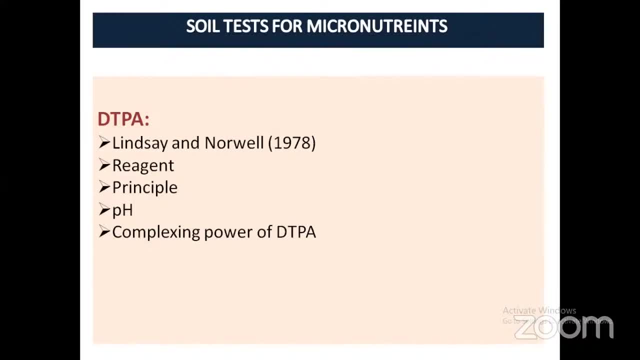 some choking in the flame of double. as for that very matter, we add t. this is one making sense to you. okay, right now, coming to calcium chloride, now why we are adding calcium chloride in it. so initially, when lindsay and norwell gave this method, gave this dtpa method, they gave it for. 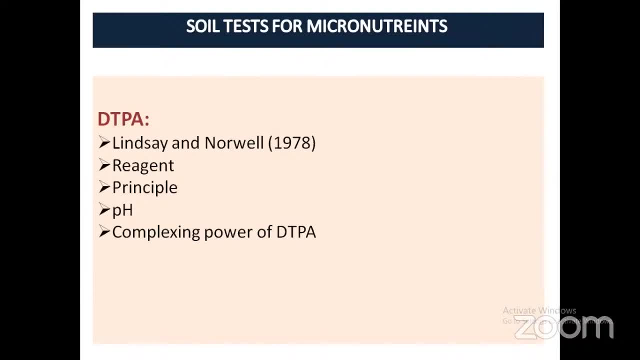 calcareous soil. initially they gave it for calcareous soil, and in calcareous soil calcium carbonate is there, so the challenge was to check the excess dissolution of calcium carbonate. so calcareous soil, initially dtpa method. so that is why this was added, making sense to all of you. 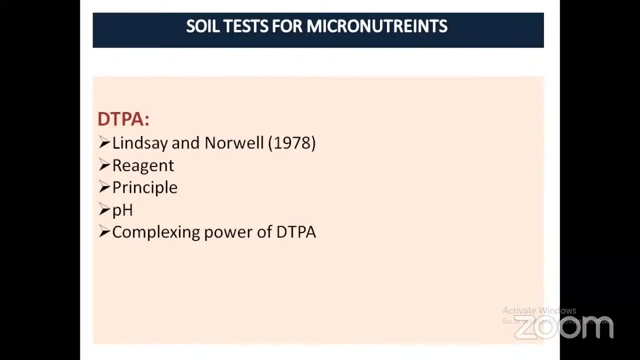 yes, ma'am, due to concentration. yeah, it was making. actually it was to check the excess dissolution of calcium carbonate. this was one of the reason of adding calcium chloride. another is we know that calcium helps in coagulation. it is a flocculating agent, so calcium helps in coagulation. so to precipitate the filtration, for getting clear extract. 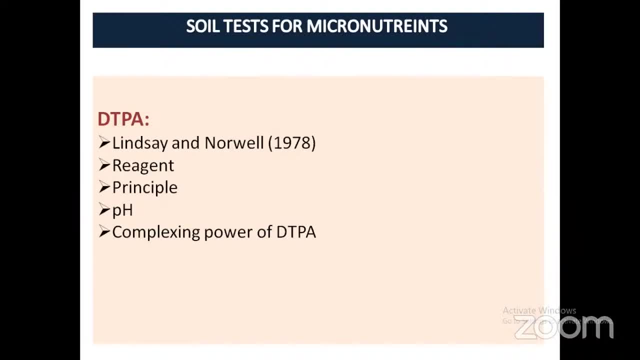 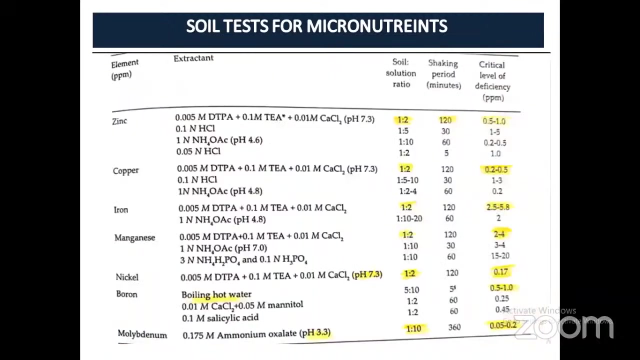 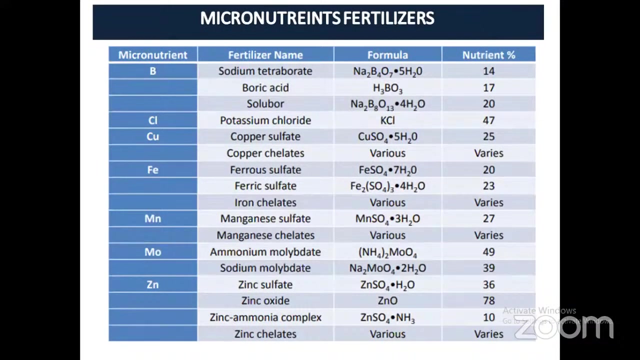 in a. okay, can i move ahead now? yes, yes, so we were on fertilizers, different fertilizers of micronutrients. their percentage is can be asked in exam. okay, boron: we used to add boric acid, usually 17, this soluble sodium tetraborate. potassium chloride- 47 percent chloride is there for copper, copper. 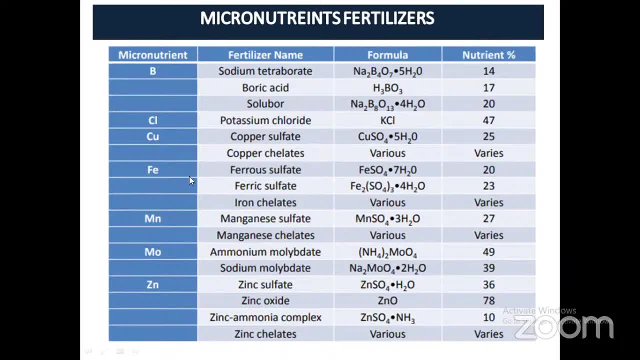 sulfate. copper chelates means copper. edta is added for iron, ferrous sulfate, ferric sulfate is added. manganese sulfate form is usually added of all the fertilizers. okay, uh, commonly asked question: is that zinc deficiency, since they are very much concerned with zinc deficiency, so they used to ask: what is the nutrient content in zinc sulfate, tetrahydrate and monohydrate? 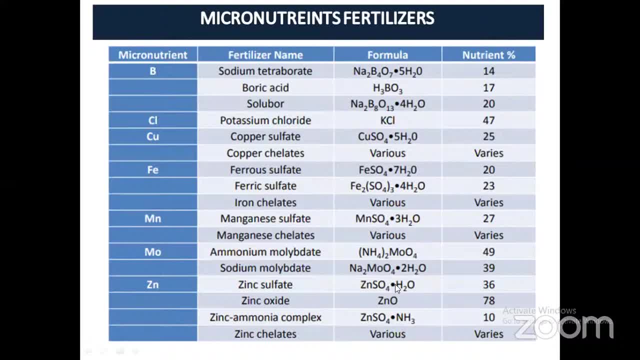 this zinc sulfate? it comes in two form. this one is monohydrate, another is zinc sulfate heptahydrate. sorry, i said tetra, that was my mistake. it is 7 h2o, so znso4 monohydrate and. 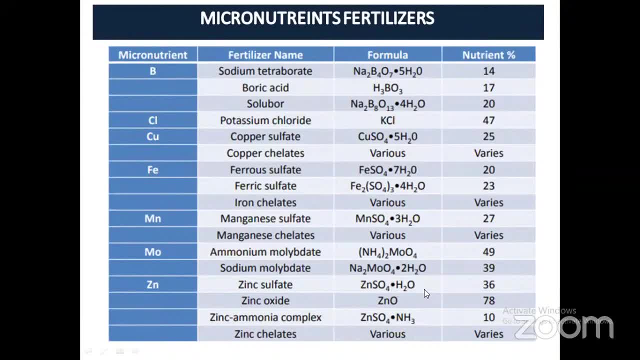 heptahydrate, okay. so they used to ask what is the content of zinc sulfate in monohydrate and heptahydrate? so you should know both okay. so in monohydrate it is 36, in heptahydrate how much? you tell 21 somewhere. it is written 21 somewhere, 27 also. so it is. 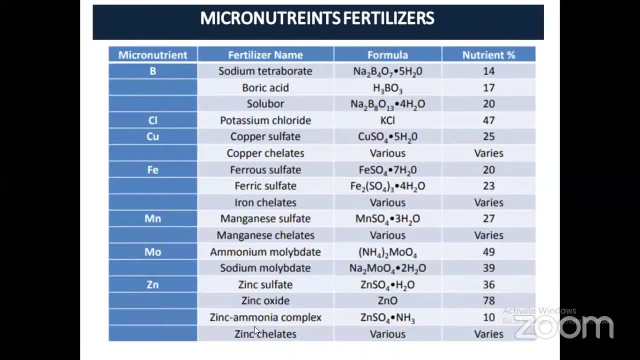 in the range of 22, 25 or something okay. another thing: if we can remember the nutrient percentage of all the fertilizers, well and good, we can't- then if we are asked that we are given a portion- We have given four options- which particular fertilizer has the highest content of that nutrient? 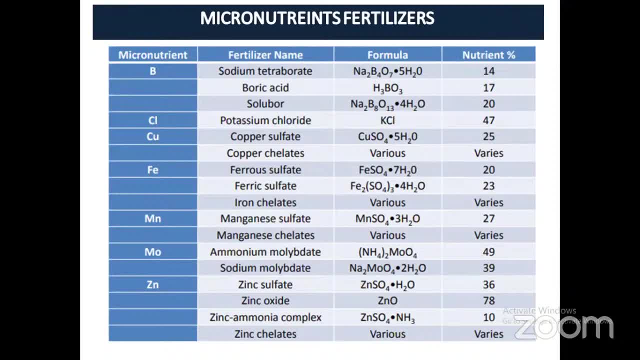 Suppose we are asking about iron and we have options like iron sulphate, iron oxide, ferric sulphate, ferrous sulphate, EDTA, etc. So if we observe, the oxide form has the highest content. If you want to answer directly, you can do so. 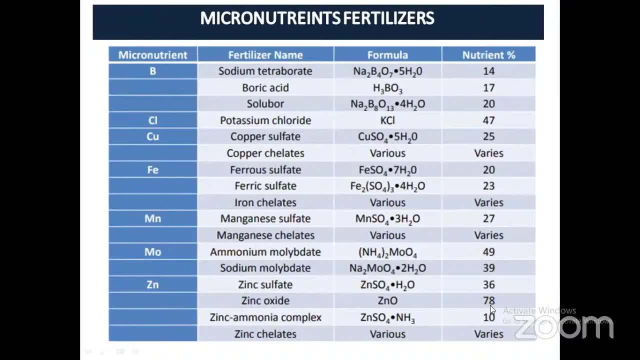 In the oxide form. if you see the zinc, the zinc oxide is having highest nutrient content. Any other oxide form It is not given here. but if you see this in book you will find that oxide form is having highest nutrient content. 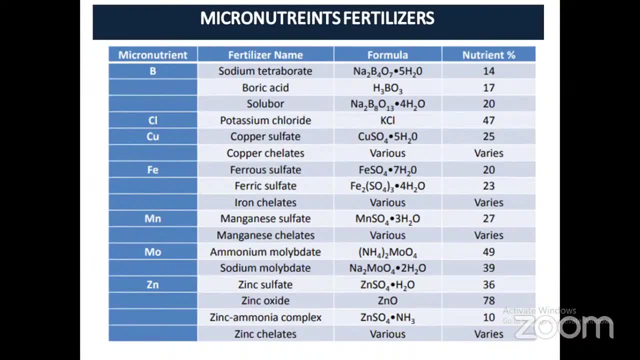 Okay, so that's all from my side. If you have anything to ask, if you want me to repeat anything, you can ask, Can you please provide this recorded class? Previous recorded class. I will provide this PPT to you. I don't know about the recording. 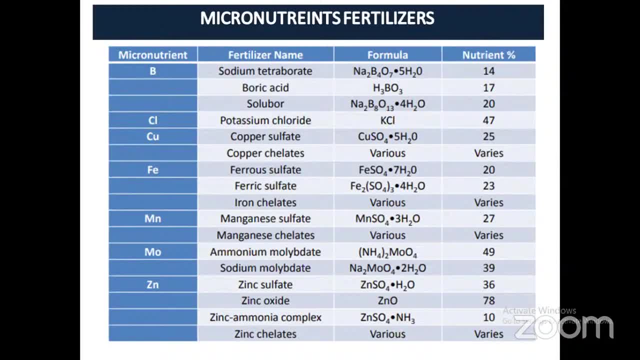 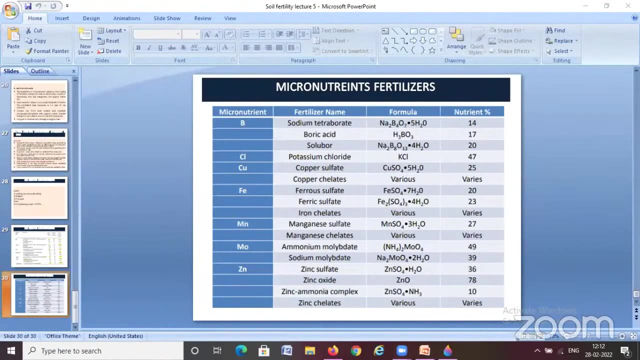 PPT. I will provide. Recording they will also provide. I am not in group, ma'am. Okay, whosoever is in group, who will take charge of all this? Sir, are you there? Suman says Yes. yes, I am here, ma'am. 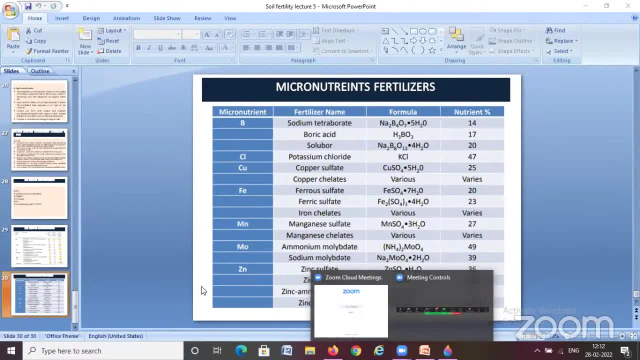 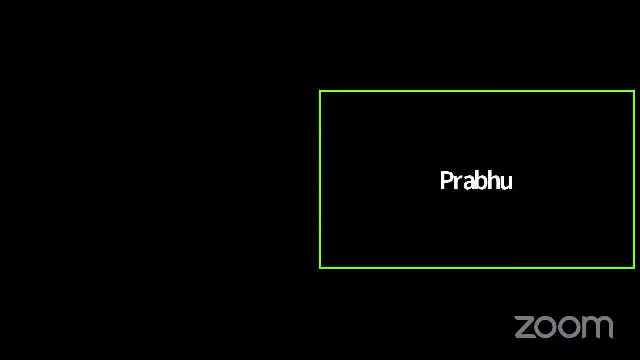 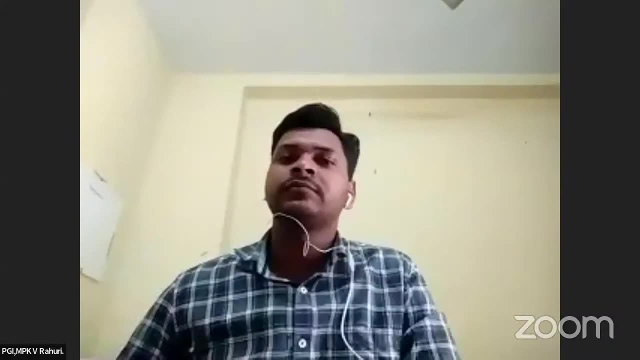 Yes, yes, yes, I will aid these boys in the group. That's good, Fine, Okay, don't worry, You take the class, Okay, Anything else? anyone want to ask or any confusion? any clarification required? Please ask another question. 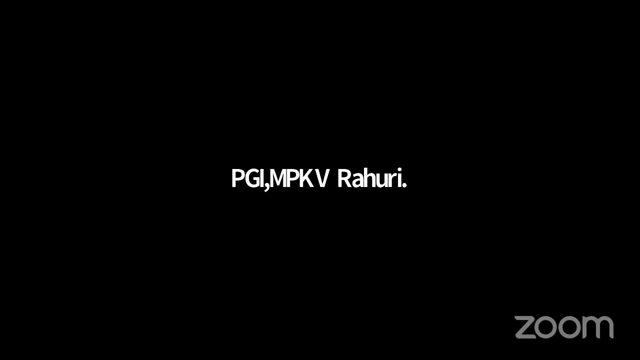 Please ask Any question you have regarding to micronutrients. Yeah, one more thing. This micronutrient chapter you read from both ISSS book. That would be sufficient. This new ISSS book, Soil Science and Introduction and Fundamental of Soil Science, very wonderfully written in both the books. 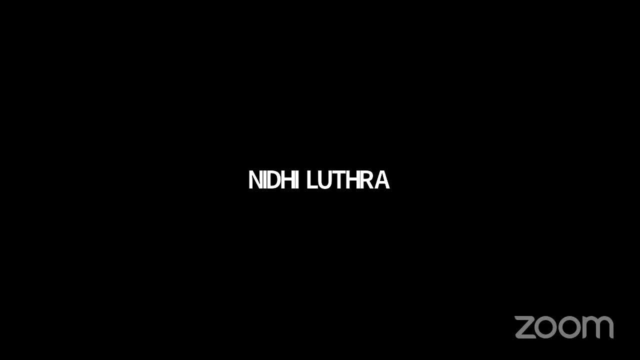 So that will be sufficient for you. But there is a specific query after that, So you can prefer Tested and Nielsen. Otherwise, both the books of ISSS are sufficient. If someone wants to read only one book, then he should prefer Soil Science and Introduction, which is new ISSS this chapter. 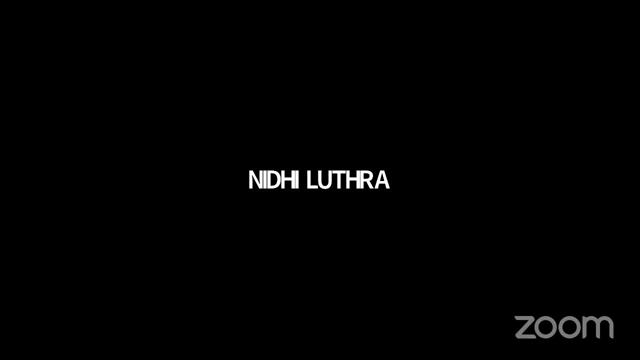 Anything else? Anything else, Hello, ma'am. My one question to you, ma'am, What's your good name? Myself Suman. Yes, sir, Yes, yes, Your question. This is the question that is asked in the nitrogen chapter by the one student. 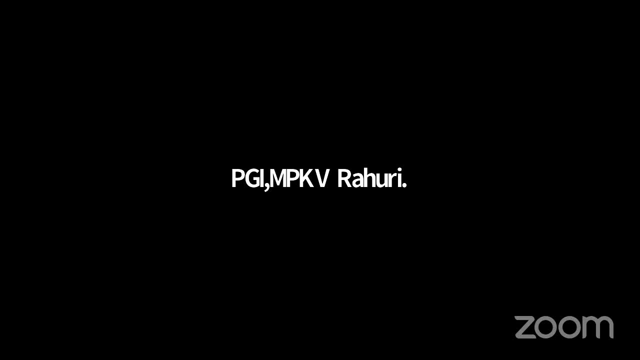 I hope there is not percent in that class. Yes, I tried to explain him, but I also request to you: you also explain these things to the students. Tamanna Sharma, I hope they asked a question personally to my call. Yes, 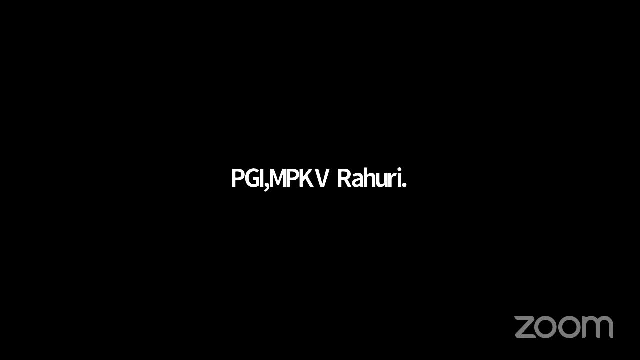 What is the question? Question ma'am: What is the dilution effect of the zinc? Zinc Dilution effect of zinc? Okay, And what was the another question? Tell something about what is the transportation of macronutrient to the plant root? 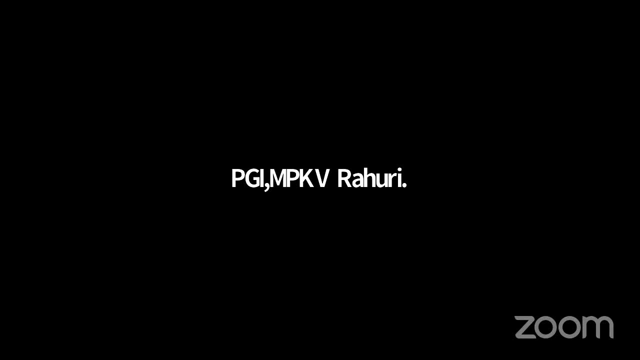 Okay, A brief idea about the transportation of the macronutrient in the plant roots. Two questions, Okay, fine. So one is: you are asking about dilution effect. You are specifically asking about zinc? Okay, But I will tell you in general what dilution effect is. 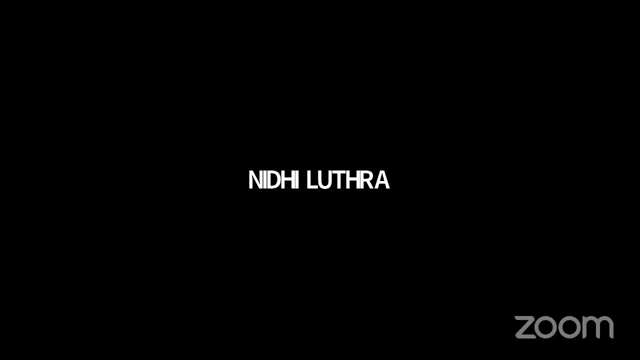 It is mainly because you know we are talking about zinc, right? Yes, Yes, Yes, It is mainly because of this micronutrient. only, Like in starting, if we talk about the plant, the biomass of our plant is less. 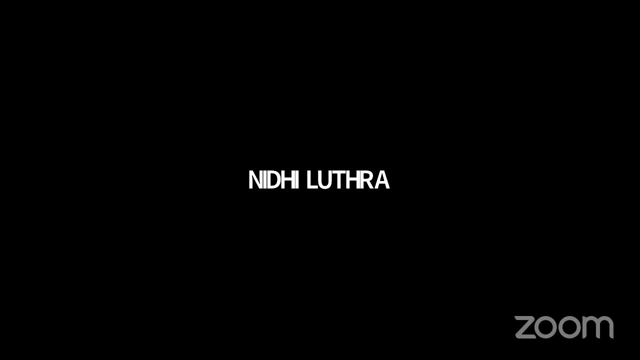 And in that the amount of micronutrient is already less. Okay. So if we look at the ratio of micronutrient and biomass of the plant, or if we look at how much micronutrient is there per unit biomass, Okay, 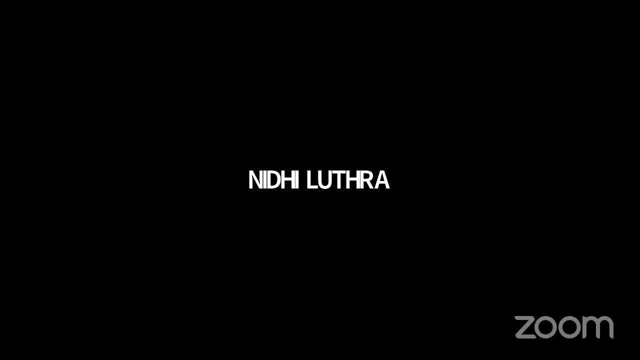 One thing. Secondly, when the plant is growing, its biomass is increasing a lot, But the concentration of micronutrient is less. So in that case, per unit of biomass, the amount of micronutrient is less. This is what we call dilution effect. 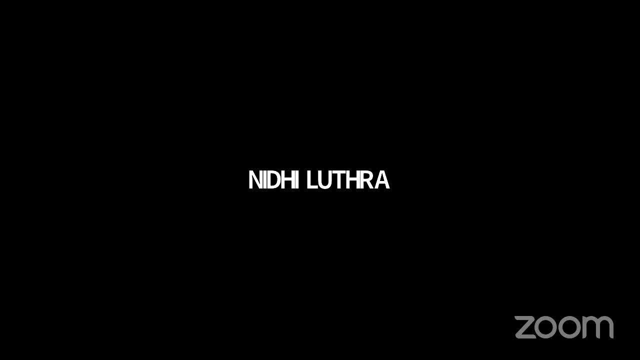 That per unit biomass. the biomass has increased, but the amount is the same, So that particular nutrient has been diluted there. This is what is dilution effect Making sense, Ma'am. is it for micronutrient or for sub-nutrient? 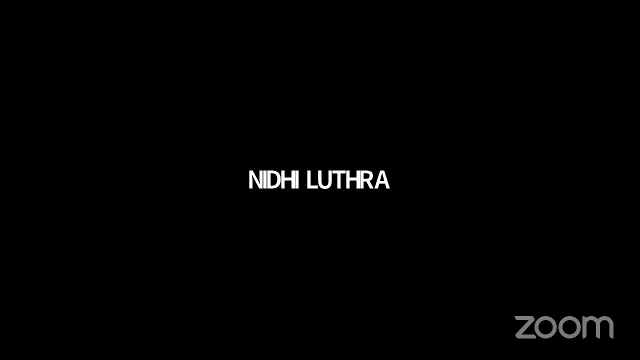 It is mainly for micronutrient, because if our biomass is increasing then micronutrient is still available to the plant, So it does not get diluted that much. But it is mainly for micronutrient, because micronutrient is in a small amount and biomass 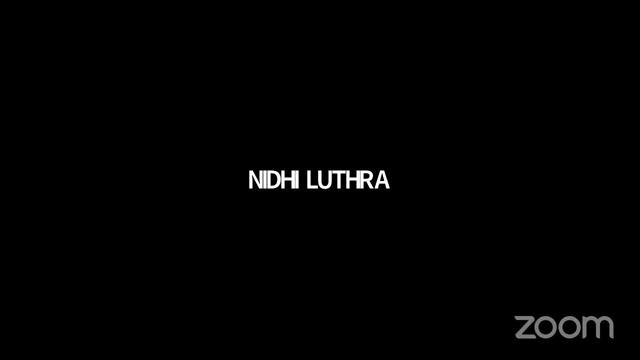 has increased, so that particular nutrient has been diluted. Okay, What is the second question? Ma'am, as you said about dilution, Give us a brief idea about Plant uptake. no, You were asking Yes, Yes, Yes. 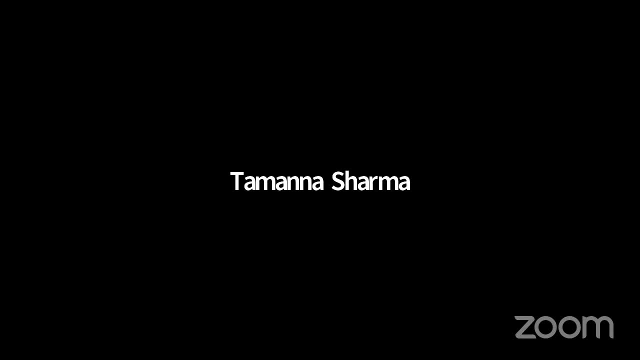 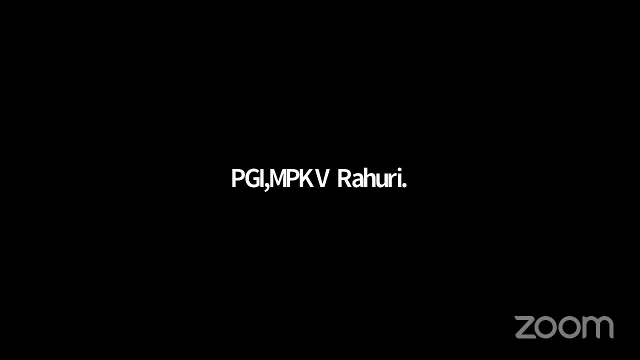 Yes, I hope there is. Tamanna Sharma want to ask some clarification of the dilution effect. I hope the question is. this question is asked by. he is in the section of the nitrogen, So I ask the question to you, Ma'am. 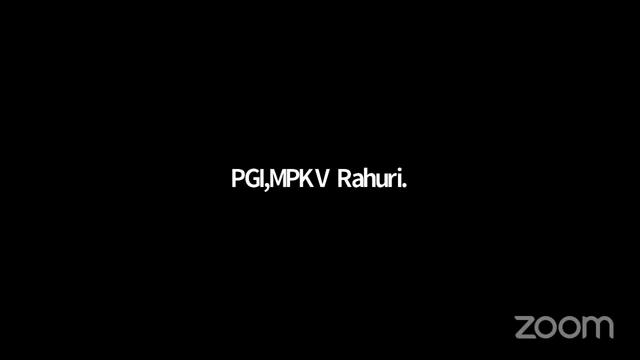 this question to you, ma'am. actually there is just something problem you need, okay, uh, if i will send you, okay, ma'am, please go ahead, ma'am, please go ahead. okay, okay, ma'am. i said. and then i you send me, sir ma'am. and i said to him: yes, i sent you. 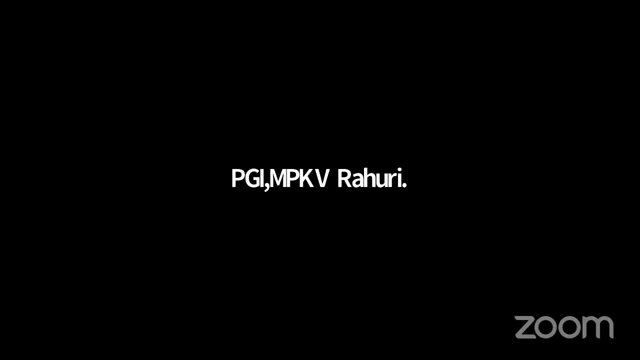 so there are basically three mechanism by which nutrients are taken up, as if not: either dilution, mass flow or another one is root interception. so generally we cannot say which micronutrients- general term, i cannot say that all the micronutrients- are taken up in diffusion form. 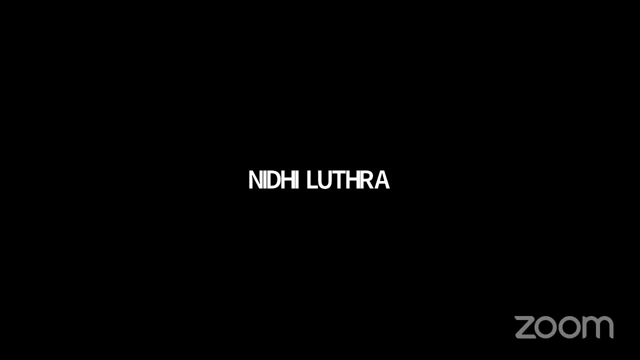 or in the form of a micronutrient. so i can't say that all the micronutrients are taken up in or root interception or mass flow. they vary means for different micronutrients, different mechanisms. okay, this question i'll also tell, because in book also they have given macronutrients. 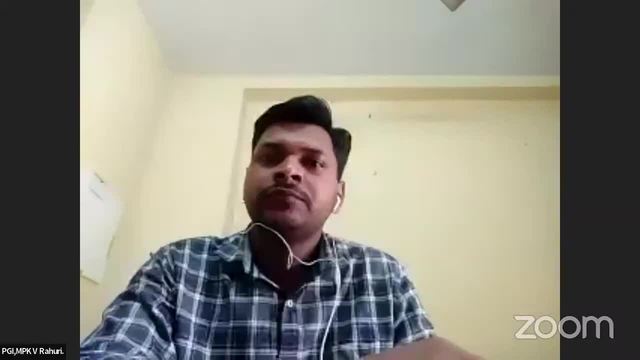 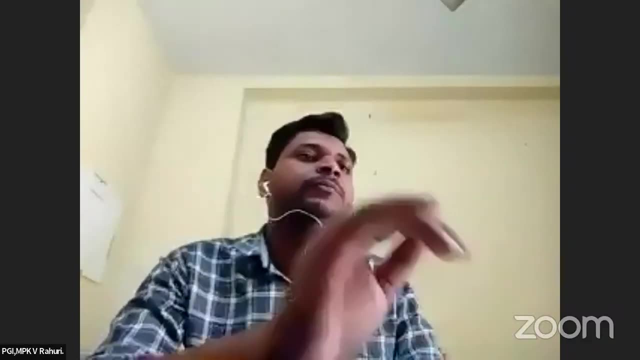 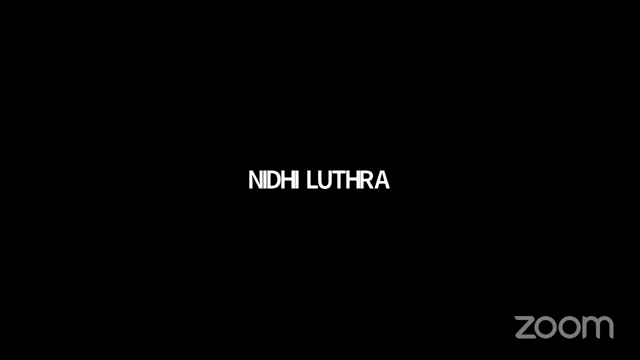 way of transporting no information about micronutrient. but i'll tell you. i have noted what the questions. i'll tell any other. okay, ma'am, no problem, ma'am, please, admin whatsapp group. when i send in my chat, i'll send to someone, sir, and here. okay, okay, i, okay, i. 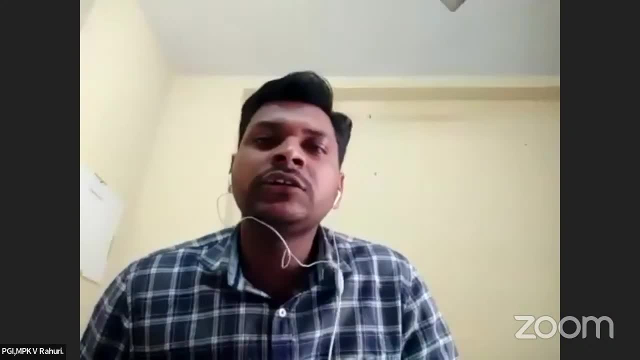 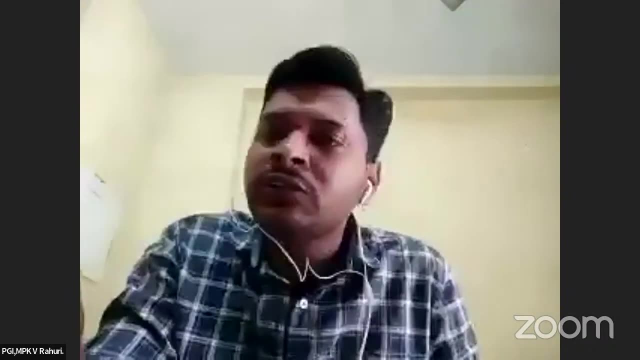 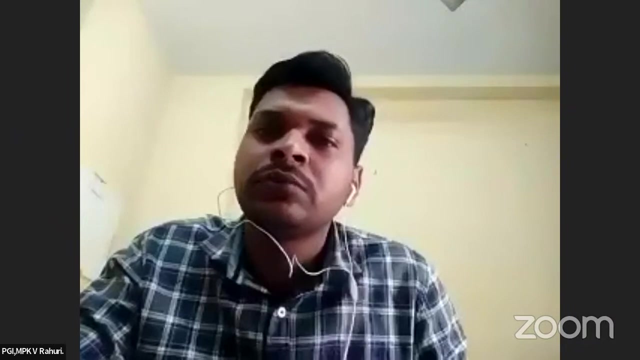 please, uh, hello, uh, take me number eight, eight, eight, eight, zero nine nine. hello, sorry, i i sent in my number in the chat box. please take this number and please, uh, give one personal message to me. i add you in the group, don't worry. okay, at the time you concentrated. 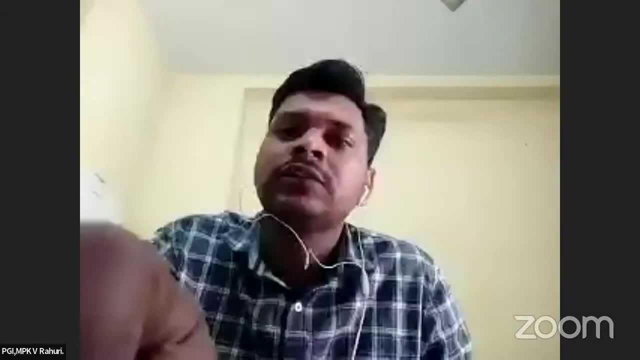 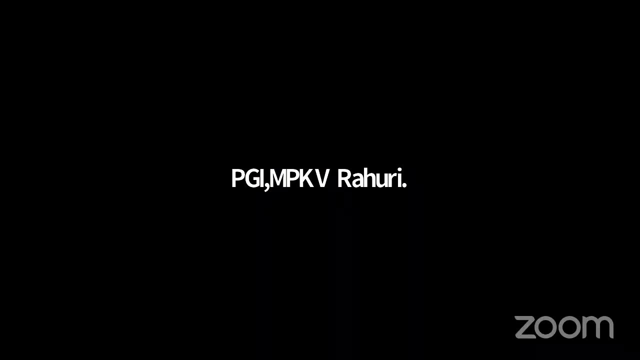 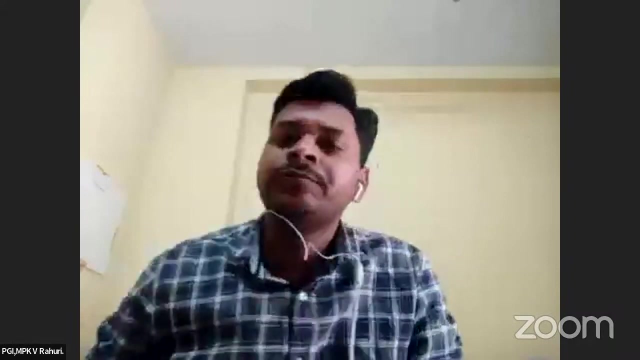 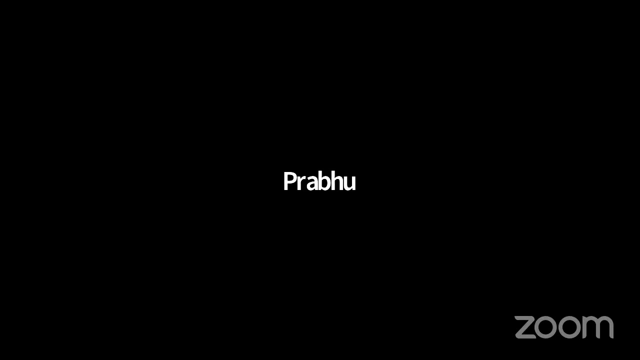 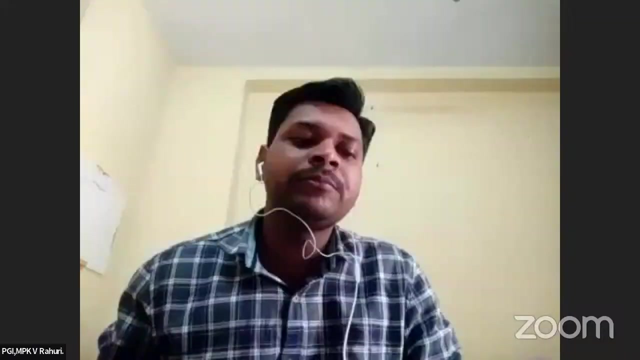 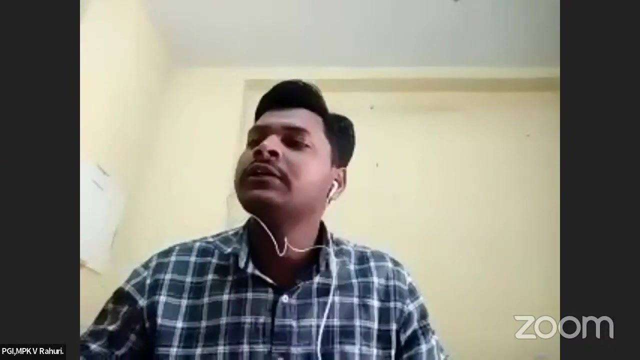 on the class sir in charge there is one guy i said i said please wait one or two minutes, okay, okay i. i said. i said i said you wait okay. so hello, hello, okay sir, hello. yes, sir, class session is in the social. please give some pivot about this. yeah, thank you. 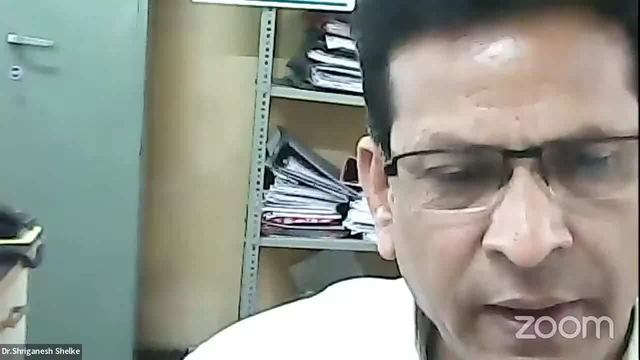 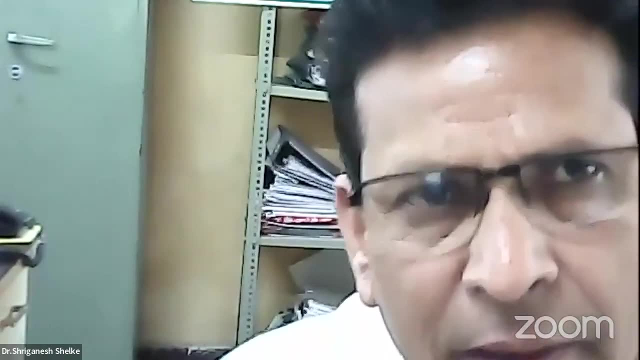 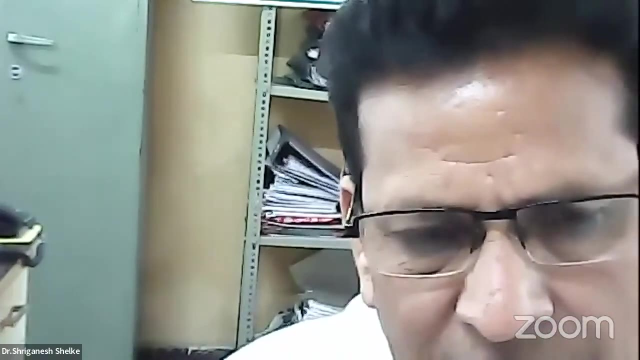 suman. thank you very nice information regarding the all the micro regions, along with all the explanations and all the deficiency symptoms and the methodology that is usually used for the acidic soil as well as the alkaline soil. you are drawn very nice and very informative information regarding. 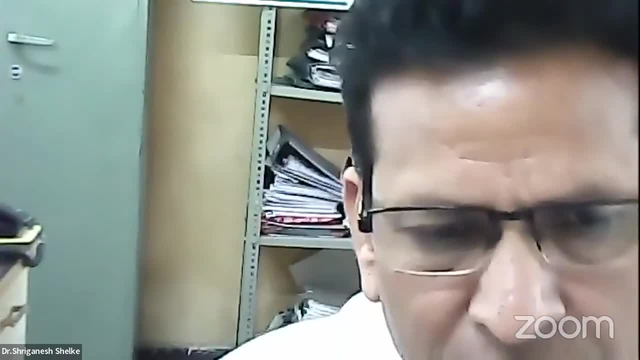 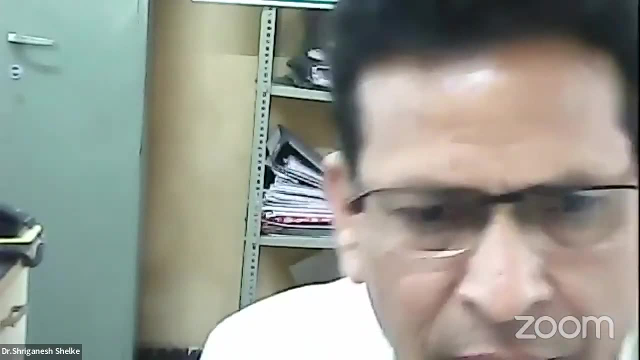 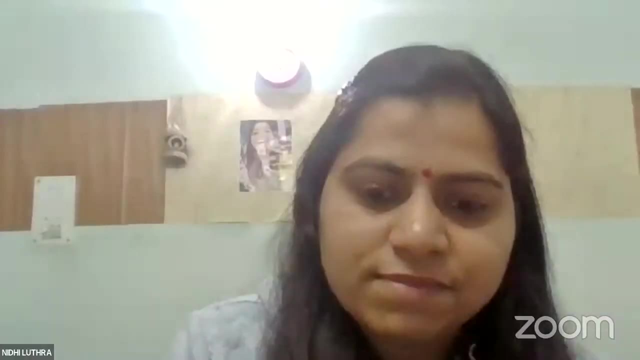 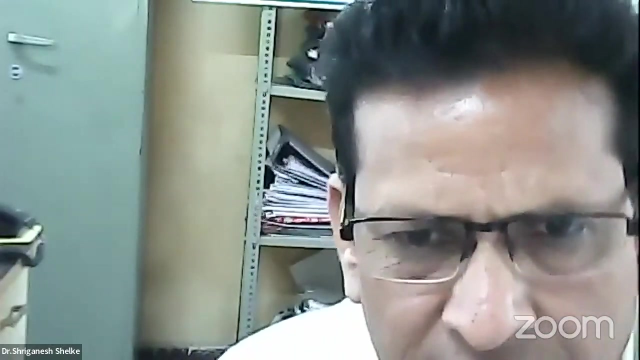 the, all the micronutrients. i am thankful to you, man, on behalf of all the post director, the faculty and all the students. i am very thankful for giving you such a nice information. definitely this information will help all the students who are preparing for the net areas and area, thank you. thank you very much, ma'am, given very, very, very, very nice information.